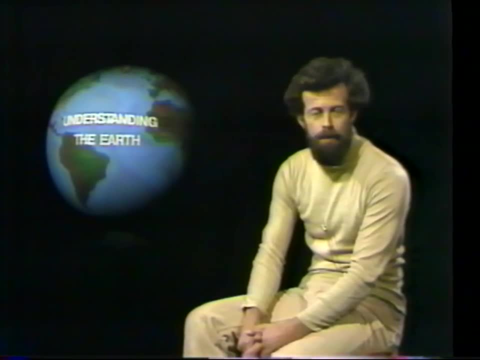 perhaps they were rather like the wrinkles on the surface of a dried-up apple, In other words, that the earth was contracting and the mountains were wrinkles on the surface. Even when I was an undergraduate, which was quite recently, mountains could not really be explained. We were simply told. 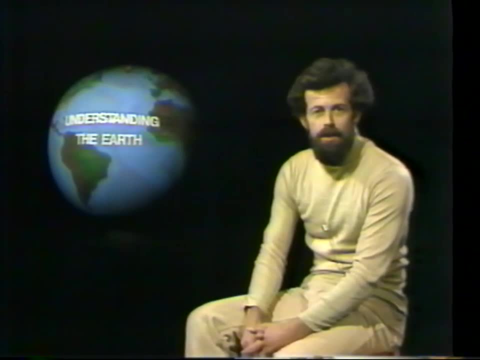 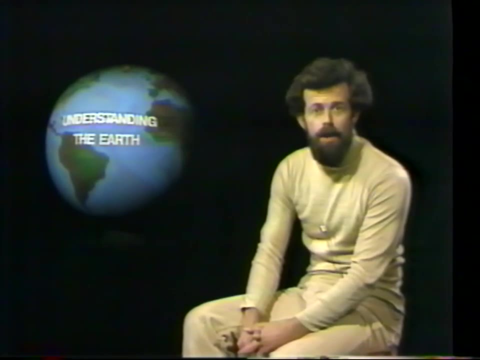 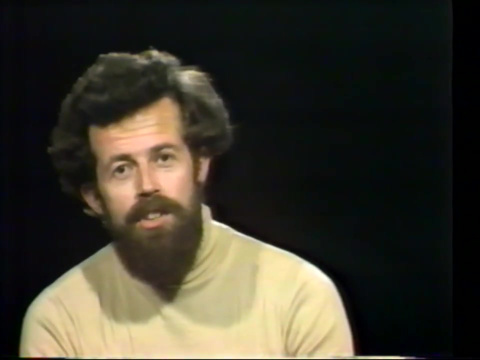 that they were great belts of sediment that had somehow subsided into the crust of the earth and been squeezed from both sides. It's not really satisfactory explanations at all, but we can now explain mountains quite well. with the advent of plate tectonics, Mountains also have their place in mythology. The Siebengebirge on the 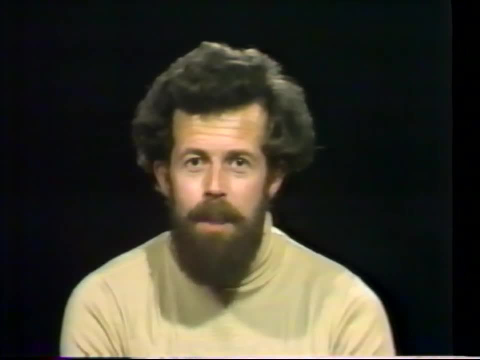 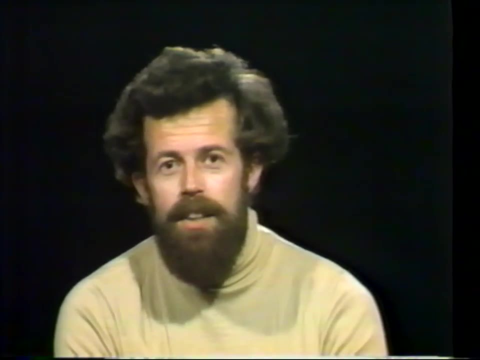 shores of the Rhine and the Rhineland are thought to be the piles of dirt that giants knocked off their shovels after they'd dug the canal, which is the Rhine, And the giant mountains on the borders of Czechoslovakia are thought to be giants who were caught out in the daylight. 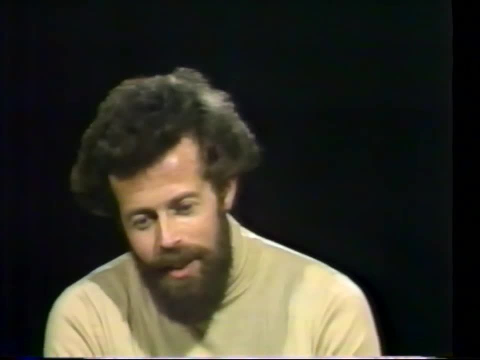 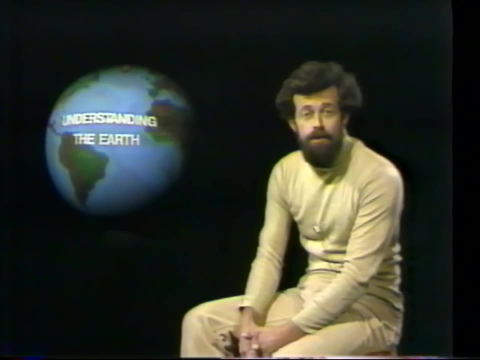 And they were only allowed to walk at night. In this program you will see first of all the discussion of the formation of mountain belts and secondly, in the second half hour, one of the Planet of Man programs, a case study on the Appalachians. 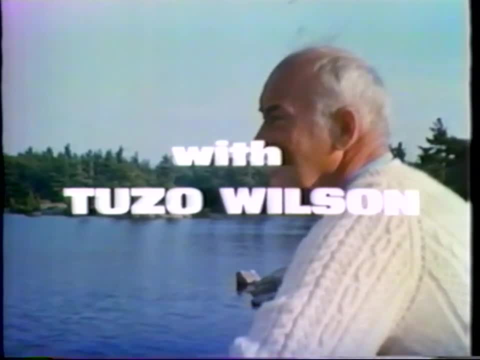 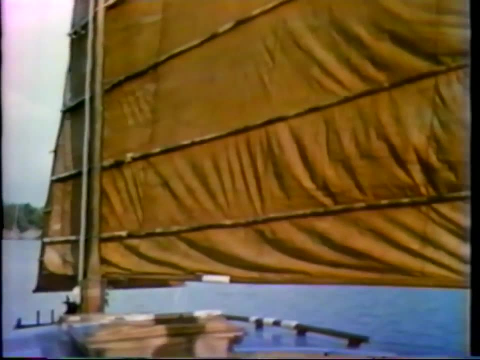 This program is about the Appalachian Mountains, which run from Newfoundland to Alabama. They've been long studied and many details have been well known for a long time. But there were certain mysteries about them, in particular why they were formed at the edge of the continent. 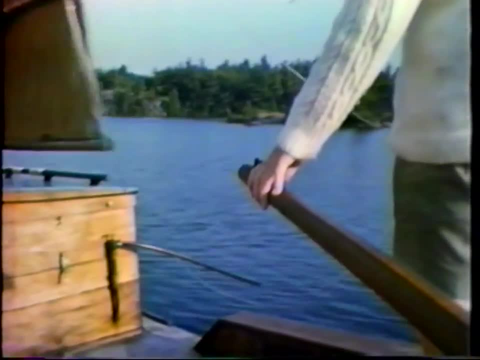 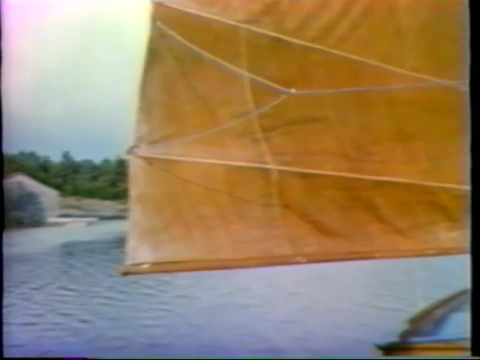 The advent of ideas about continental drift and plate tectonics has done much to explain this mystery. It's now thought that three or four hundred million years ago, the continents of Africa and Eurasia bumped into North America and the collision pushed up the Appalachian Mountains. 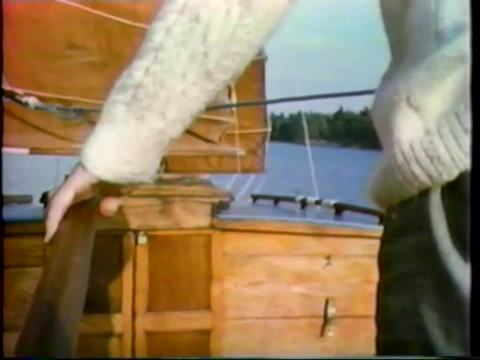 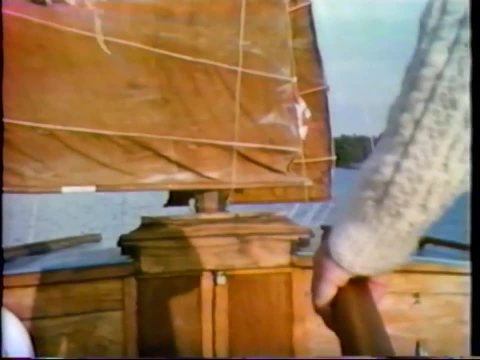 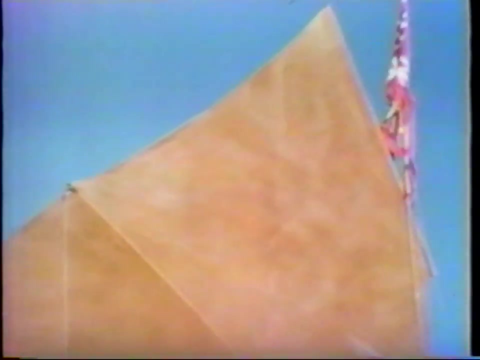 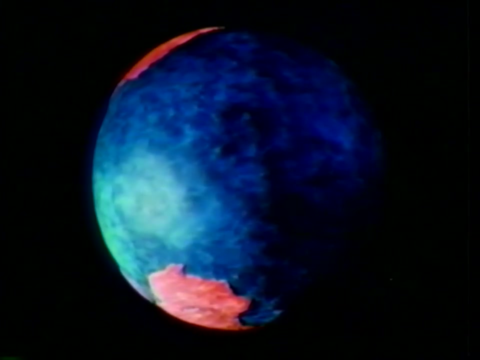 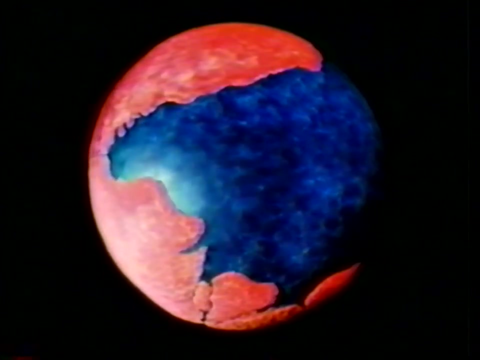 At that time they were probably much higher than they are now and resembled the Himalayas or the Andes, But the passage of time and erosion has worn them down to their present general slopes. Our world two hundred million years ago, The supercontinent Pangea. 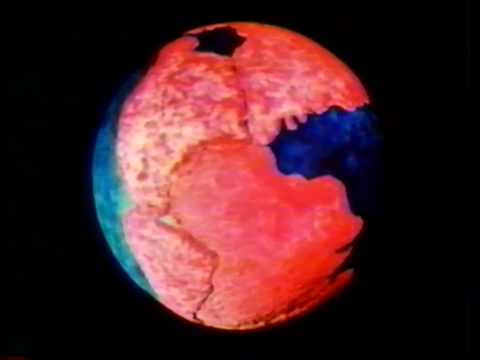 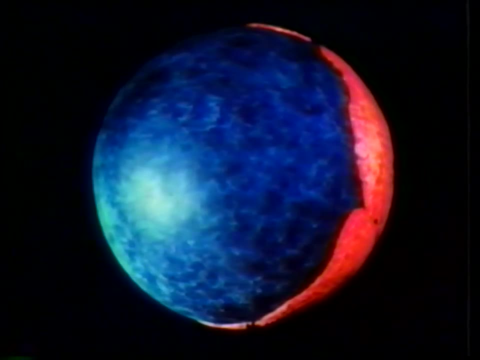 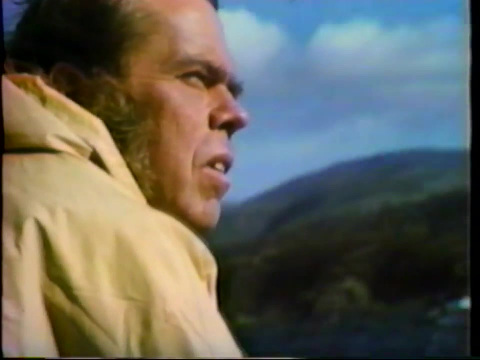 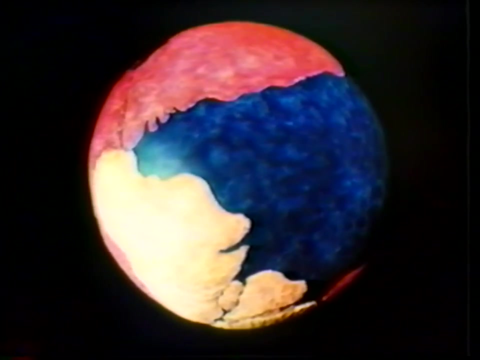 Its continuous coastline, bordering on a universal ocean. In its irregular forms, we can read the shape of things to come. as we can read familiar shapes in clouds, We can infer where India, now wedged between Africa and Antarctica, will soon commence its long journey north to collide with Africa. 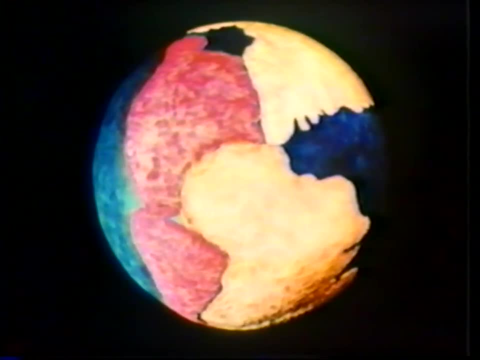 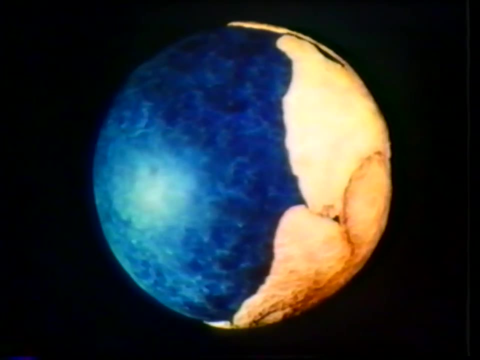 Where the Atlantic will open, moving north in South America to the west. But we will have to infer much more, For on the immensity of this supercontinent we will find none of the great mountain ranges. That too is yet to come. 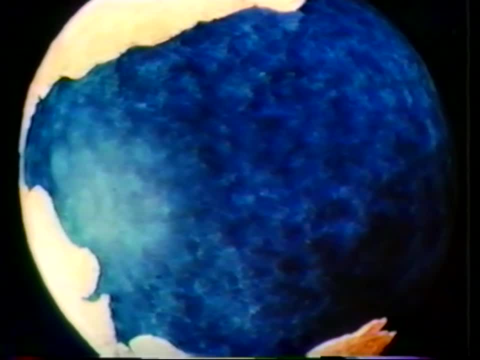 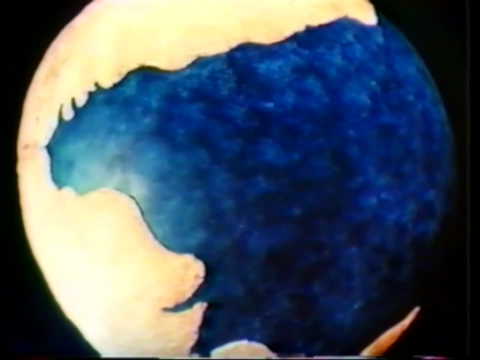 The margin of southern Asia is flat, For the Himalayas will not begin to rise for another year. The Mediterranean will begin to rise for another hundred million years. That event waits for India's drift north and the collision that will lift up the mountains. 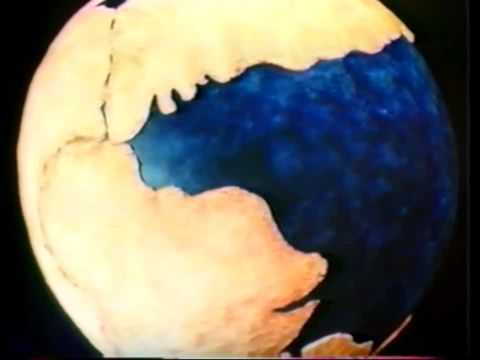 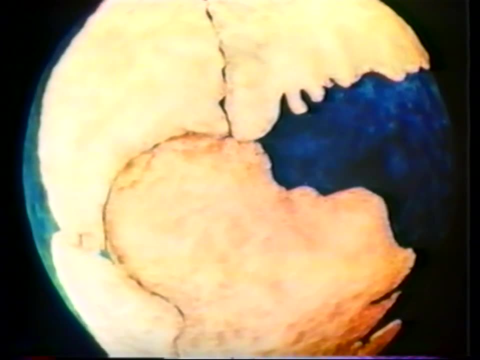 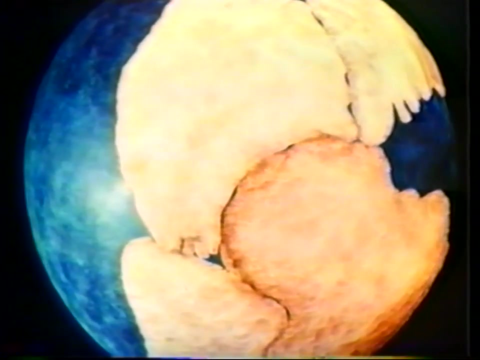 The Alps, too, are nowhere evident. Before they appear, the Mediterranean must begin to close, bringing Africa in collision with Europe and folding up the great range we know today. The Andes and the mountains of western North America will begin to appear some million years hence. 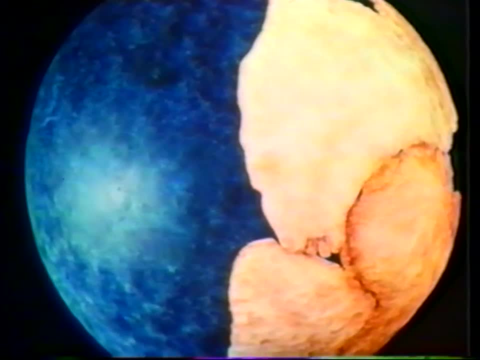 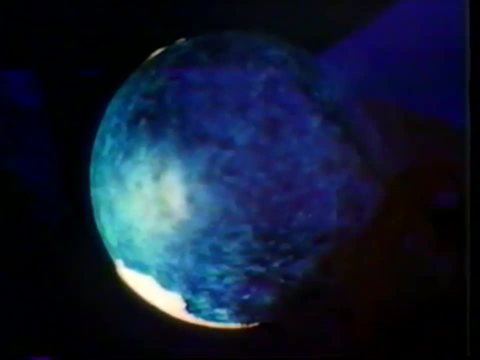 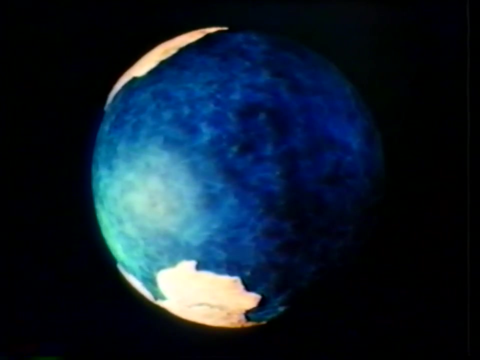 They will rise up when the westward drift brings the two continents into conflict with the crust of the Pacific. Are we looking at the prelude to the world as we know it? This picture of our planet is a mere two hundred million years from the present. 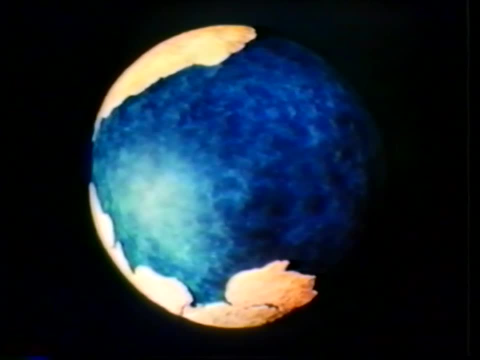 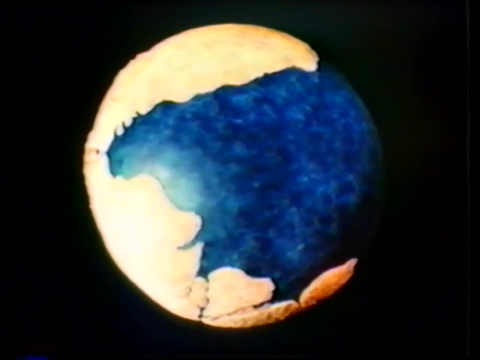 A small space of time in the four and a half billion years of its existence. Is it possible that this was the beginning, Or were there other shapes and continents, Earlier drifts and earlier oceans? Are we looking merely at a stage in a continual process? 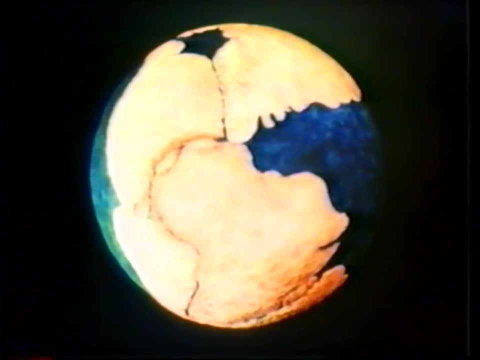 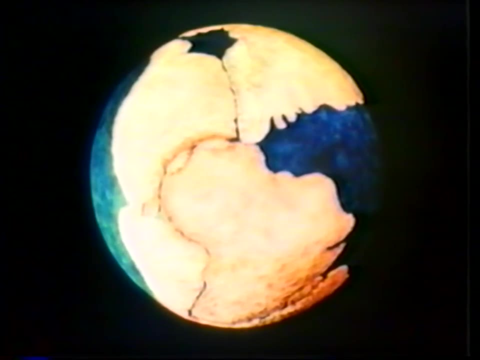 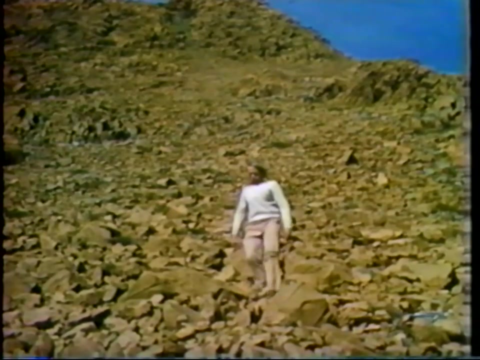 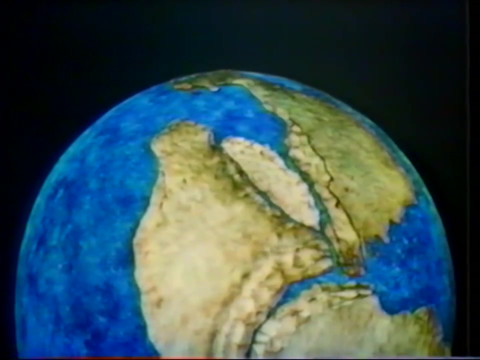 The answer is yes, And the evidence rises here, in the heart of the supercontinent, near the point where North America and Europe will be separated by the still unborn Atlantic Ocean. The, The range of mountains, the Appalachians, stands as high as the Himalayas. 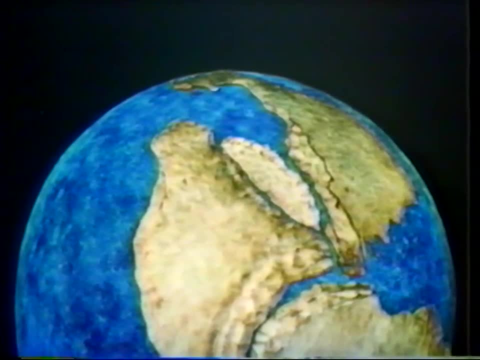 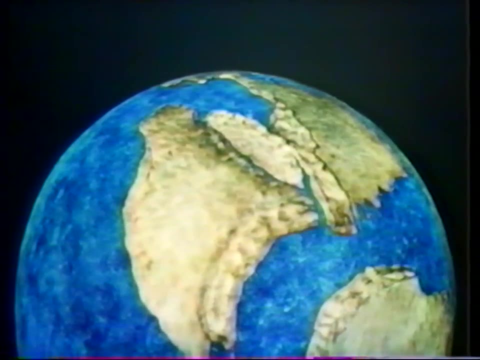 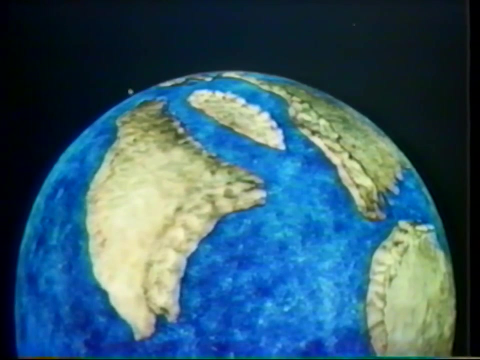 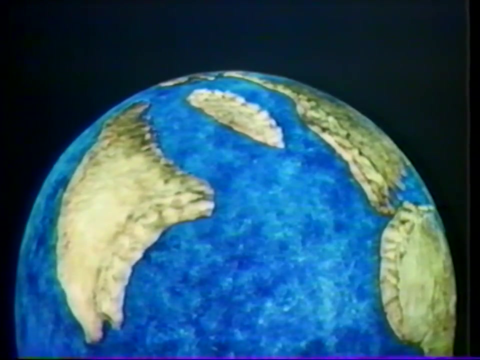 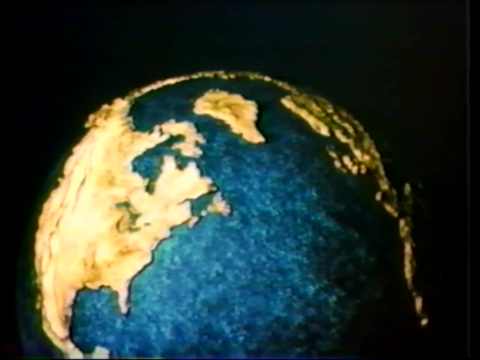 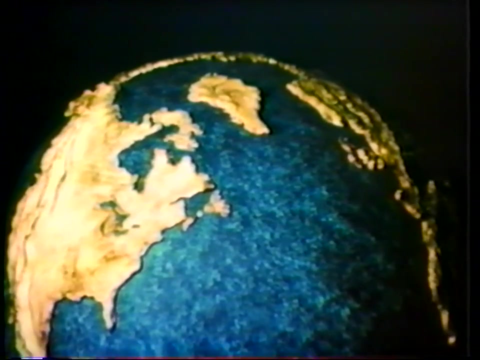 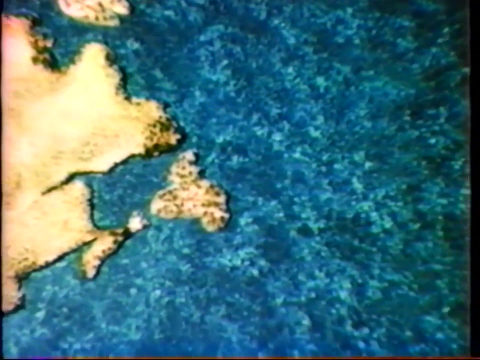 And, like the Himalayas, was probably formed by a closing ocean basin. Two hundred million years ago, Pangea started to break up And in time, were christened with new names. Inescapable, the movement of time watched them eroded to gentle rolling humps. 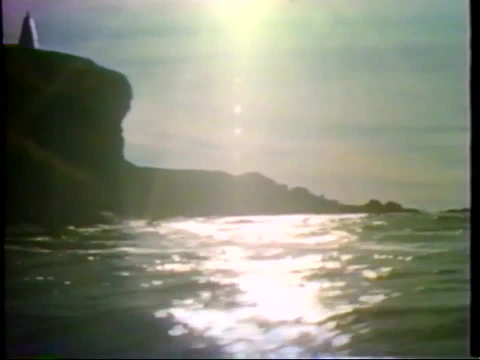 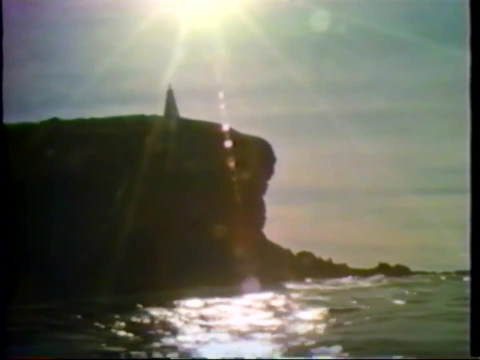 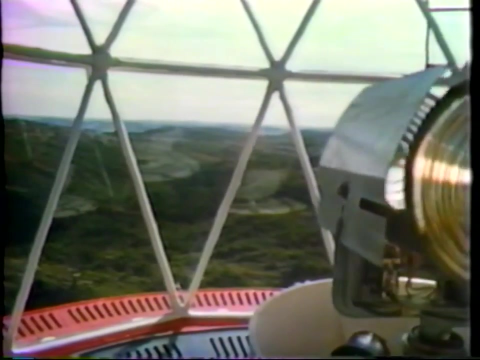 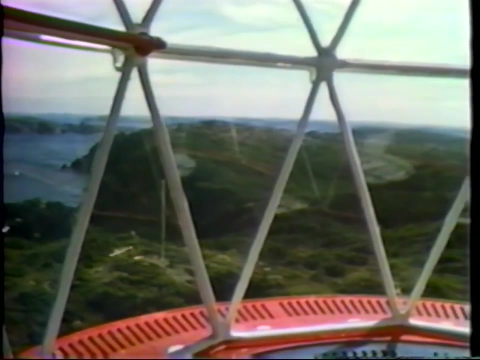 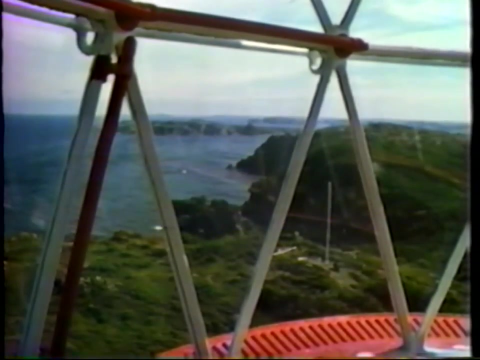 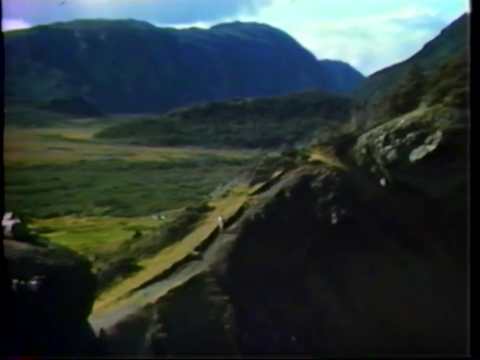 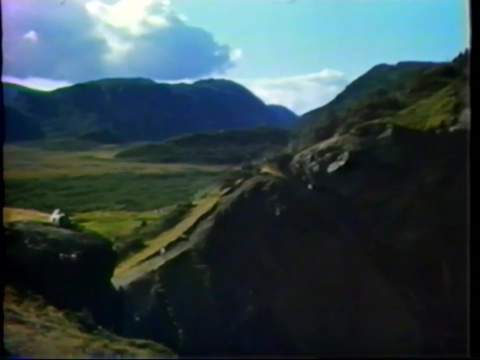 nubbed and subdued, like the well-thumbed features on an ancient coin. This is Newfoundland. These hills are the remnants of the old Appalachian Mountains. The scene is weirdly similar to parts of western Scotland and even to parts of Norway. 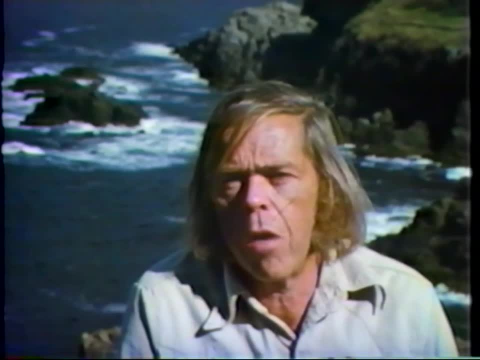 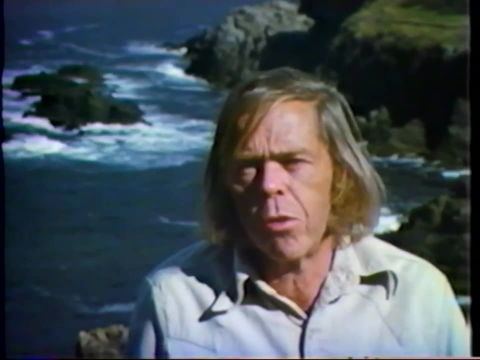 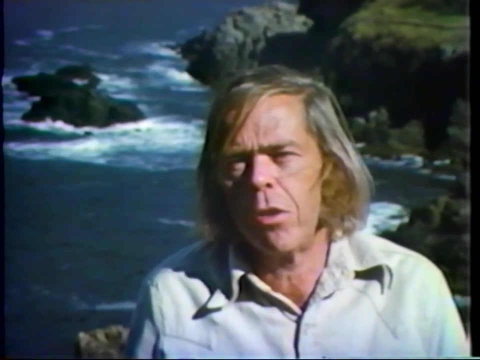 In the beautiful coves, little harbors and along the coast there are really fantastic rock exposures. And these rock exposures have become world famous to geologists, at least because of the story they tell, And it's the story of the history of the formation of the Appalachian Mountains. 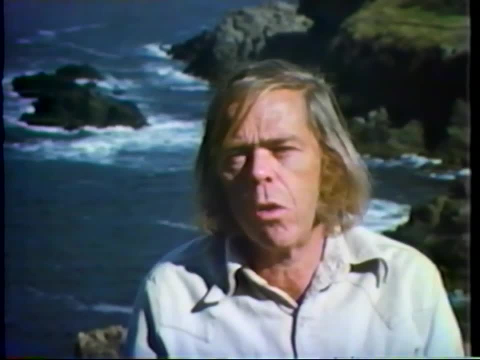 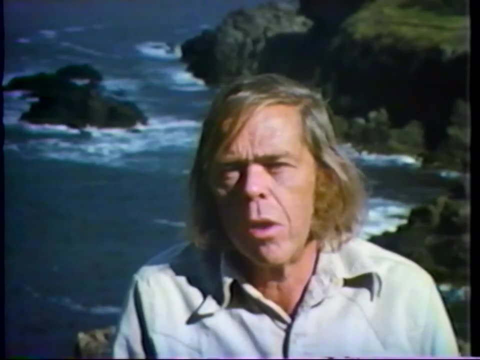 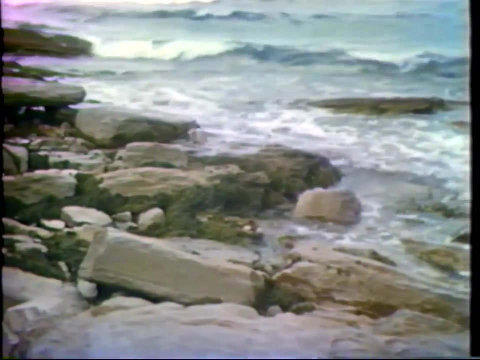 And it's quite a history, involving a shrinking ocean and the collision of two continents. This story began over five hundred million years ago when Pangea was done. Newfoundland was divided by an ocean. Newfoundland was divided by that ancient sea. 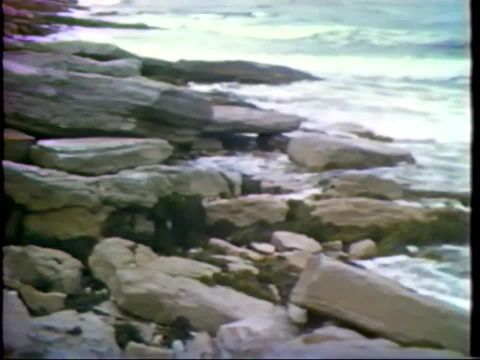 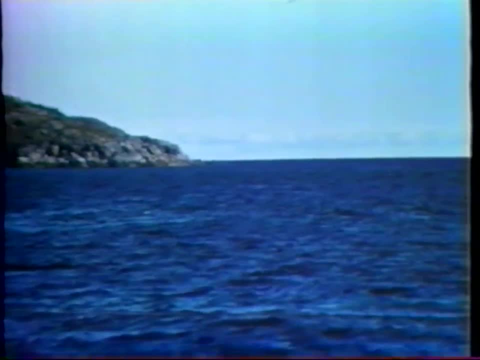 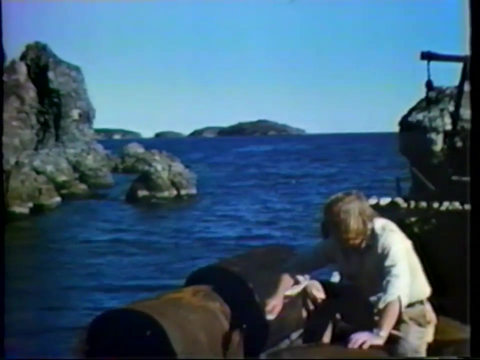 The western part of the island belonged to one continental mass, whereas the southeastern part of the island belonged to the opposing continental mass. Now, off the edge of the old continent, we would have found pretty much the situation that exists today along the Atlantic coast. 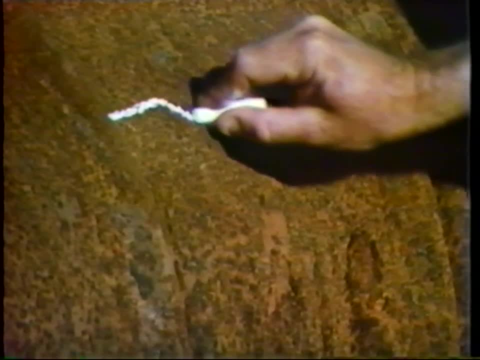 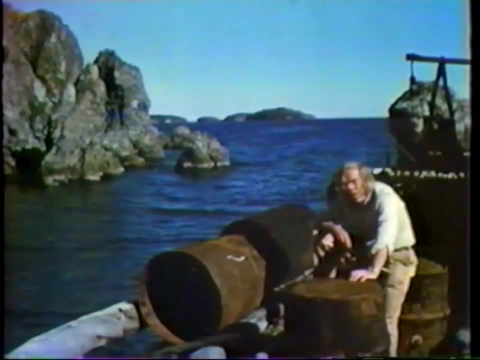 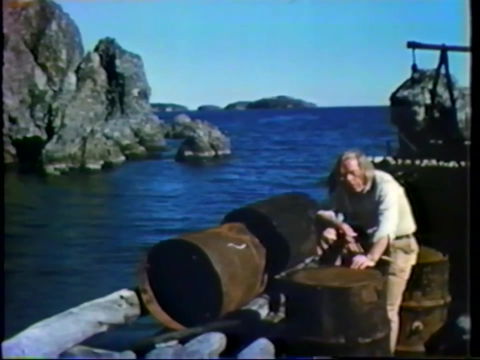 Namely a continental shelf, continental slope dipping somewhat steeper and a deep ocean floor bottom. Now how do we know that an ancient ocean existed here? Well, the answer is simple: In Newfoundland we find rocks from the ancient ocean floor bottom. 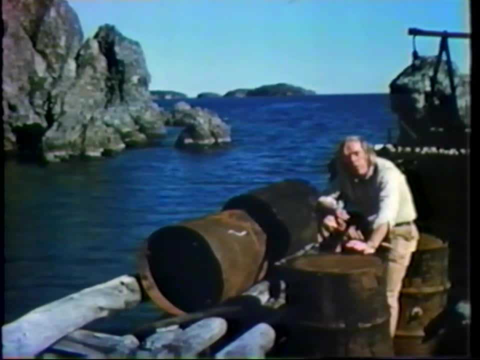 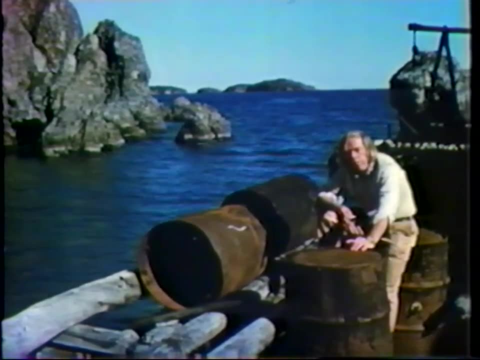 and from its continental slope. In fact, about a third of Newfoundland is underlain by rocks from ocean floor bottom. Such rocks are well exposed around Nipper Harbor. Some of the rocks we find cover the entire width of the ocean floor bottom. 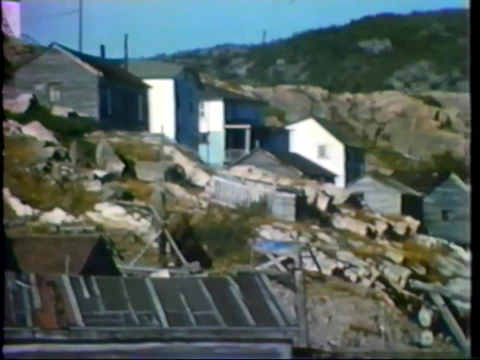 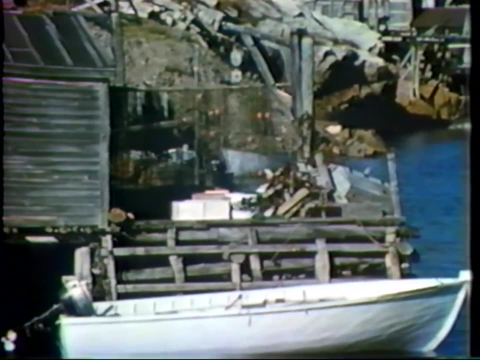 One would say they are called The Newfoundland Sea. In fact, Nipper Harbor is the state of Newfoundland that has expanded its systems. In the past three centuries. Newfoundland has suffered the most olmayance from the ocean floor and has become stronger and stronger. 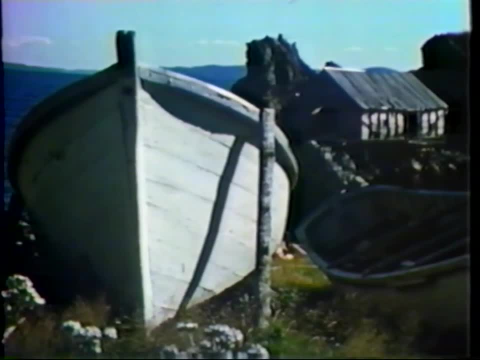 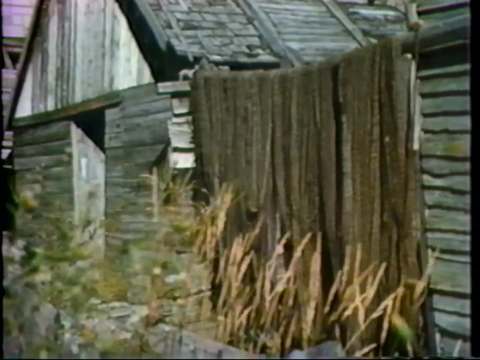 However, the most lasting harbour in Newfoundland is the Nipper Harbor, which is the first place in the world where you can have the greatest of experiences. In conclusion, Newfoundland sea's edges are very connected to the ocean floor, So the fishermen at Nipper Harbor who live off today's sea. 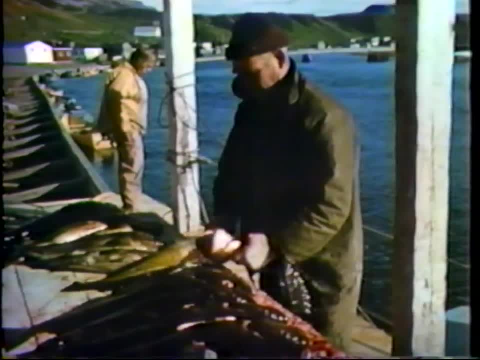 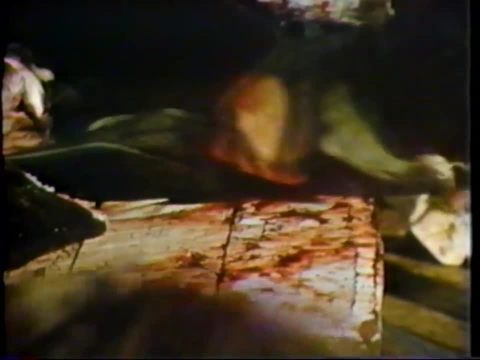 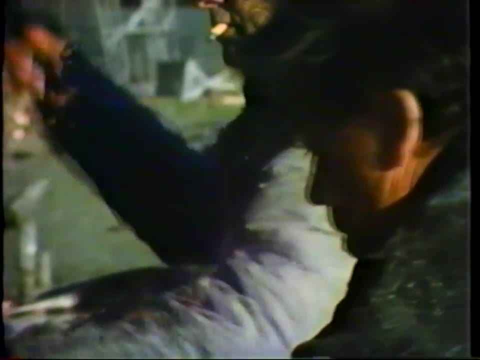 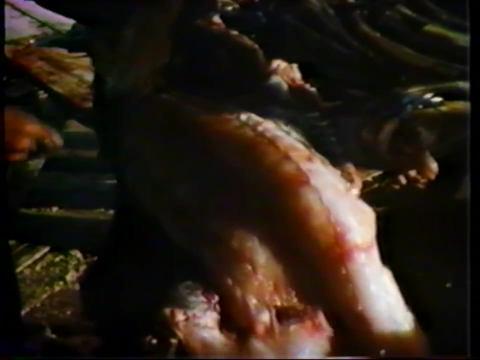 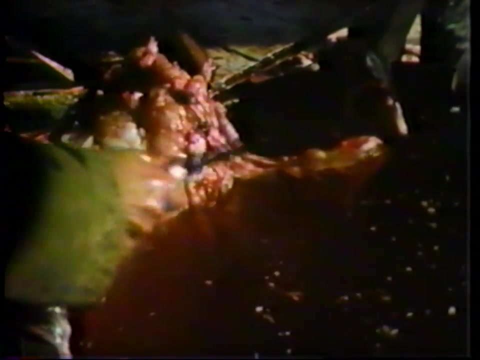 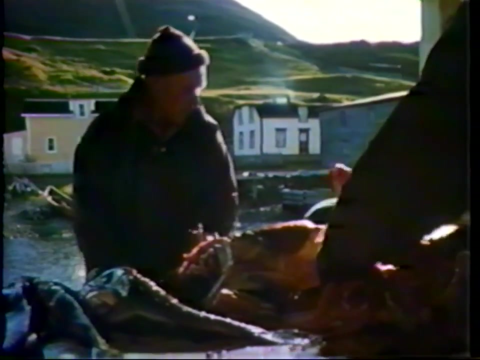 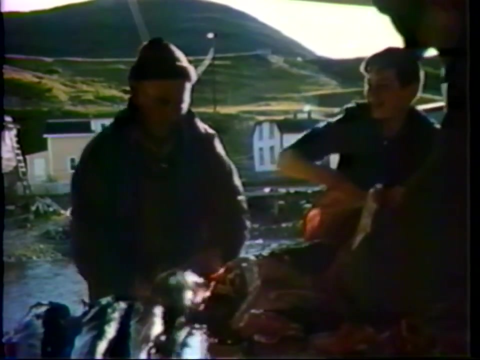 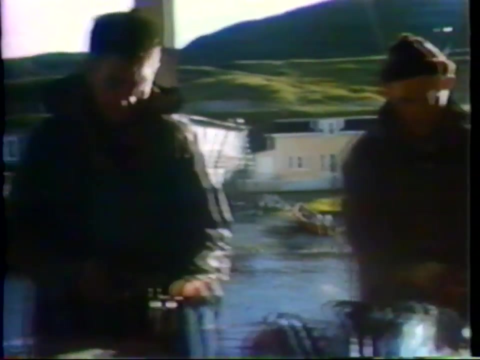 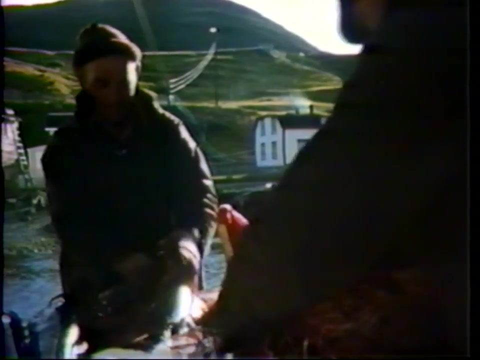 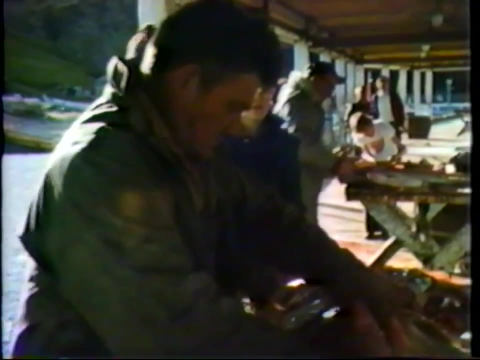 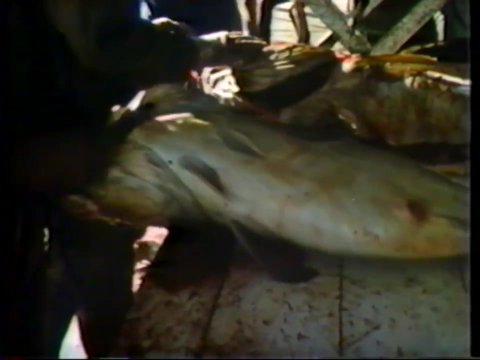 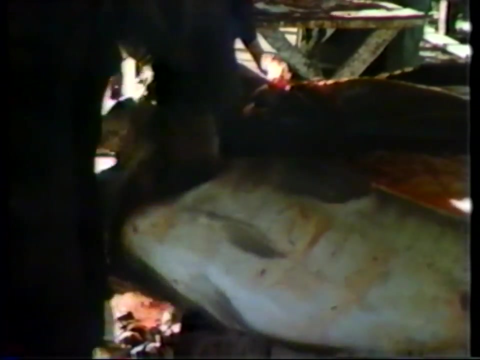 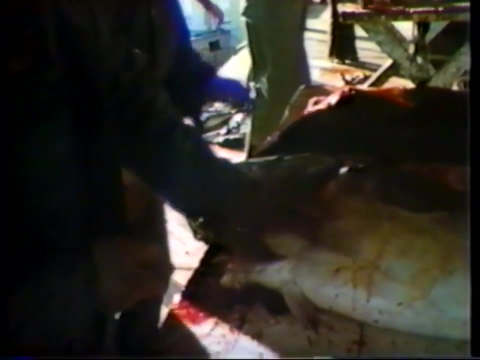 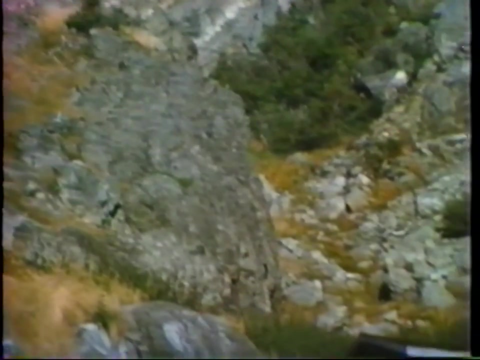 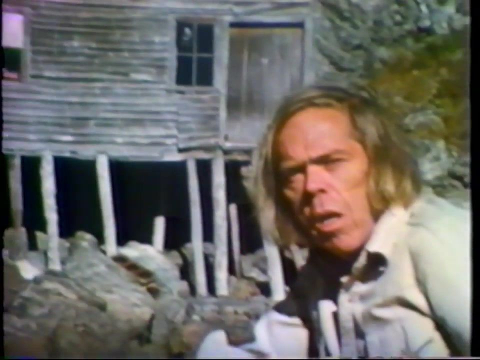 live on the floor of an ancient sea. I've got one, sir. Thank you, Hold on. Thank you, Hey. Hey, We know these rocks once formed the floor of an ancient ocean. How did they get here? Well, the process is a very complicated one. 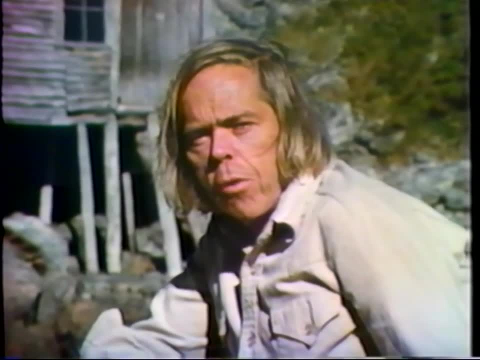 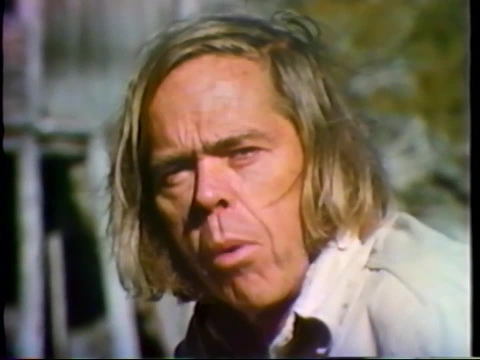 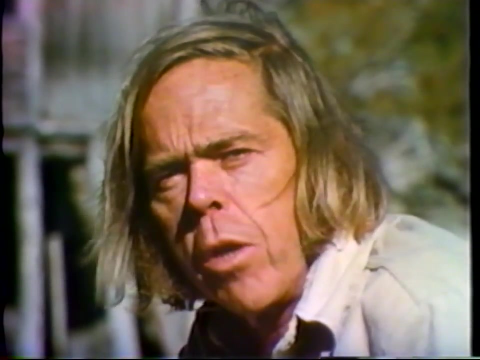 and it really is a story of mountain building. And so, for the Appalachian Mountains, we began with an ancient sea. Now that sea differed from the Atlantic in one rather important way. The modern Atlantic Ocean is spreading Sea flora crust is being created along the Atlantic Ridge. 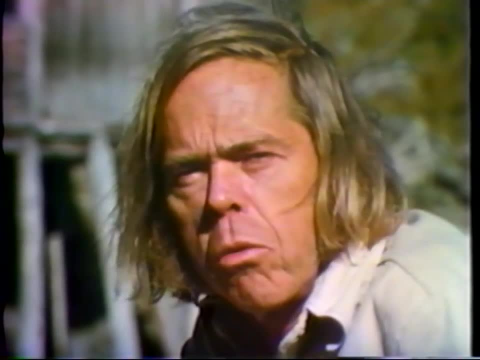 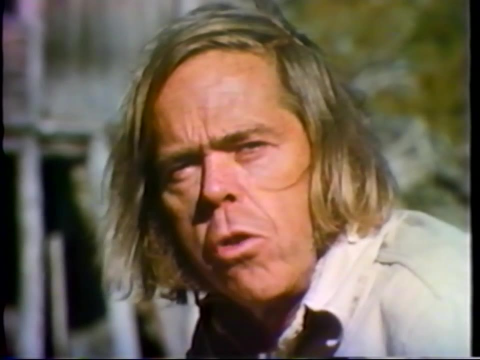 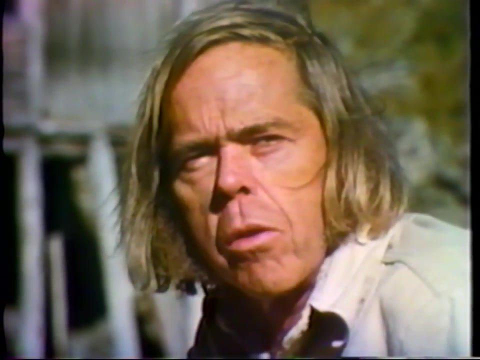 In fact, North America is moving from Europe at the rate of about two or three centimeters a year. The ancient ocean was shrinking. In other words, Europe and North America were coming together. Now how does that happen? Do the rocks between buckle? Do they fold? Do they bend? Not so. The first part of the process begins with a slab of crust or ocean floor bottom sinking into the earth like so. As it gets down deep, it gets hotter, It begins to melt. Magmas are generated, They move up to surface and you have off the coast a series of volcanic islands or volcanic arcs, much like modern day Japan, Small and weak, a bit less than mor, but may be even more. They're all in spots of ocean surface. 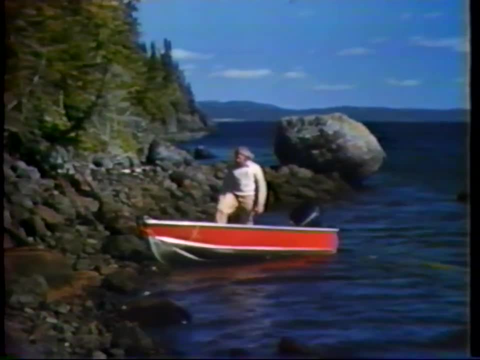 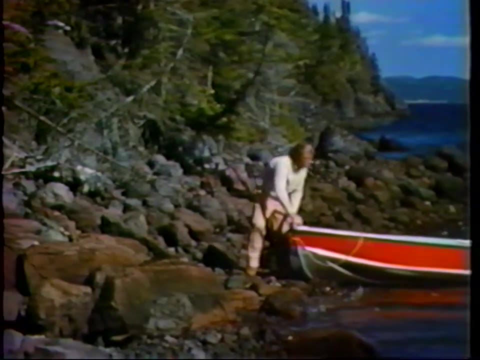 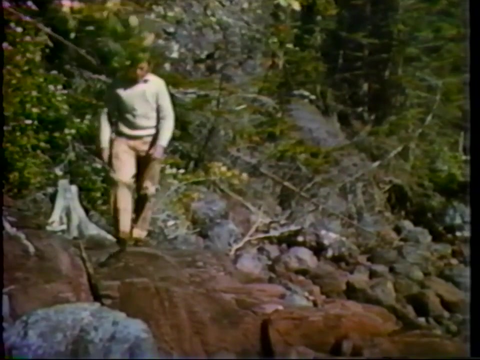 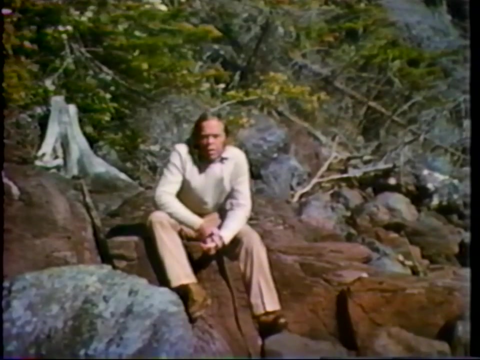 They form frescoes called chiaroscurophagous fovara. who guess the same as we do? How do they go down? They're just coming to the surface, They mix, they Doorrrrrr. Well, here we are, at the roots of the volcanoes. 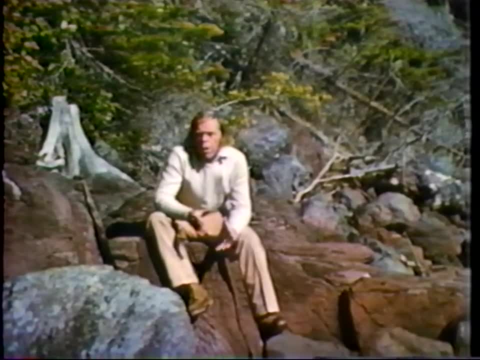 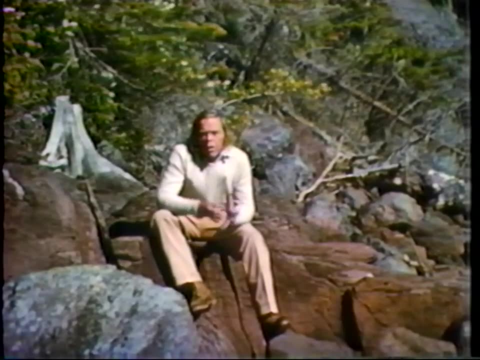 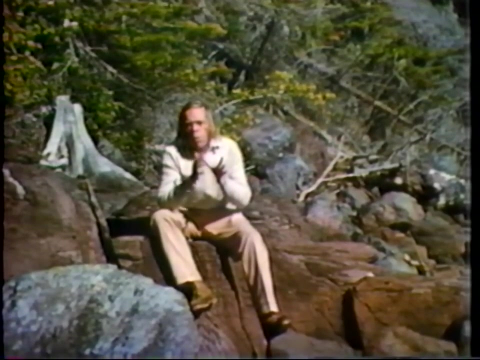 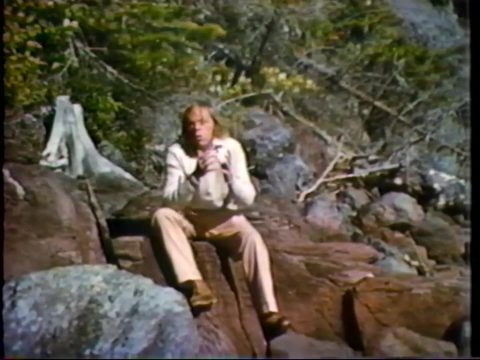 Time and erosion have done their work, leaving only craggy remains which frame these really beautiful, tranquil coves that dot this part of the coastline. Now. contrast this tranquility with the explosive violence of the past, when you had hot molten material spewing from the earth moving down into steamy seas, when you had explosions. 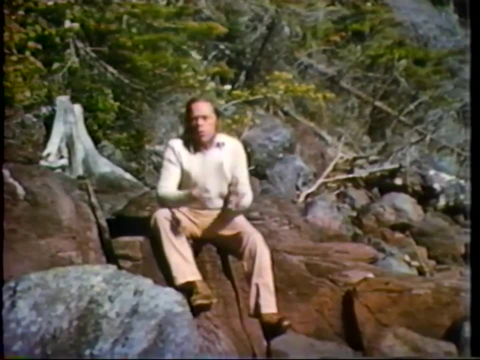 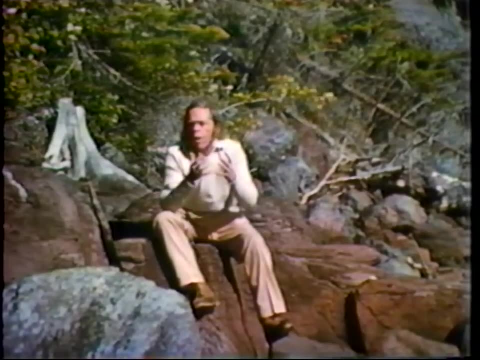 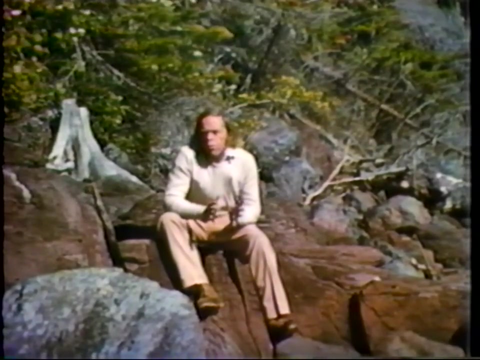 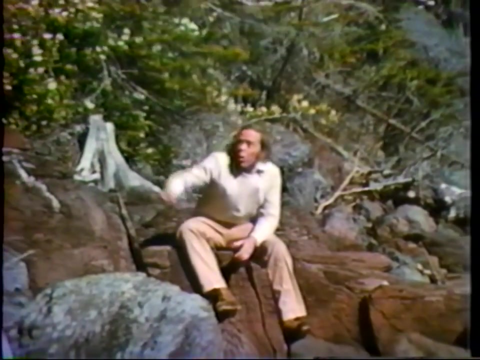 of gas and fragments of rock into the air, settling on the earth, when you had really explosive mixtures of hot gas, rock fragments streaming down river valleys and hillsides, etc. Really explosive times, spasmodic but explosive. Now you want proof of all of this. well, here it is. 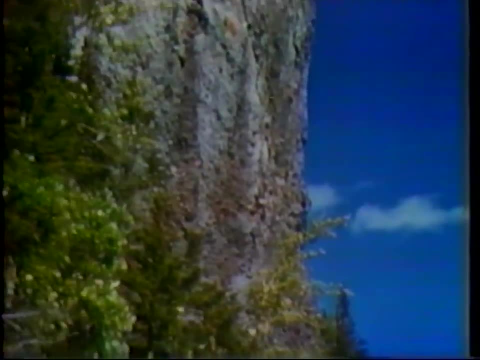 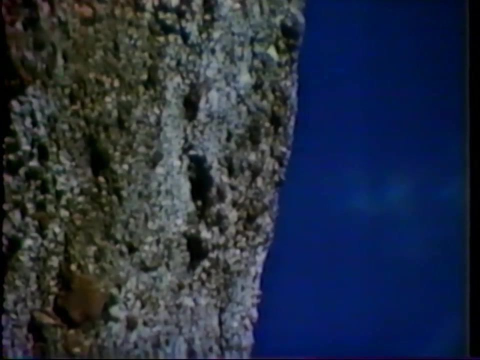 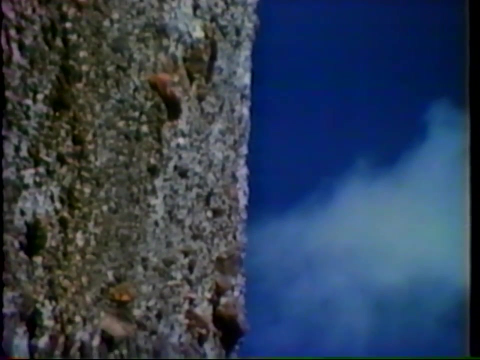 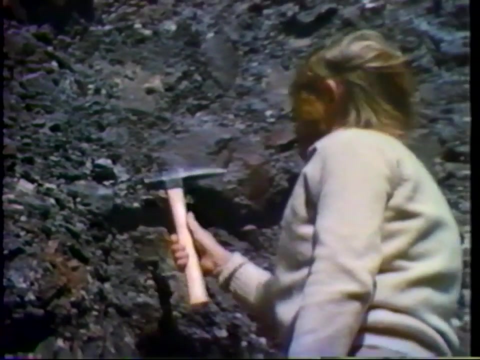 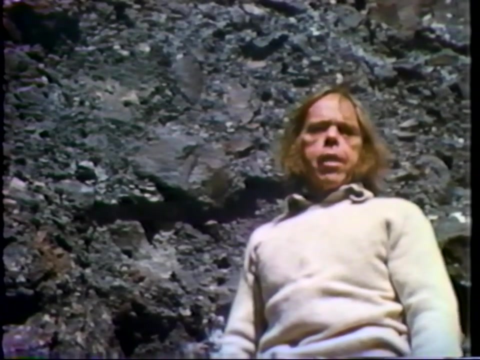 A volcanic vent from which rock ash lava was ejected, some of which fell back to fill the vent. Well, it looks like a mixture of boulders of volcanic rock and ash, and in fact that's what it is. However, with time, the ash has consolidated. 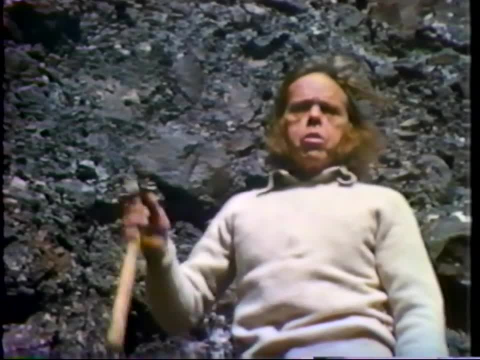 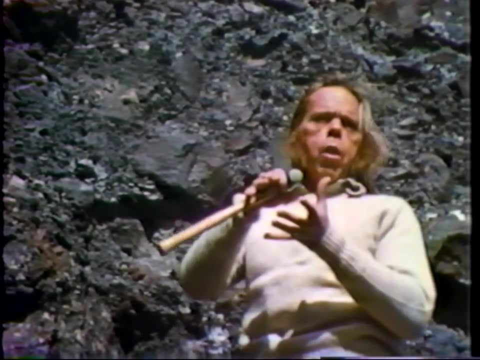 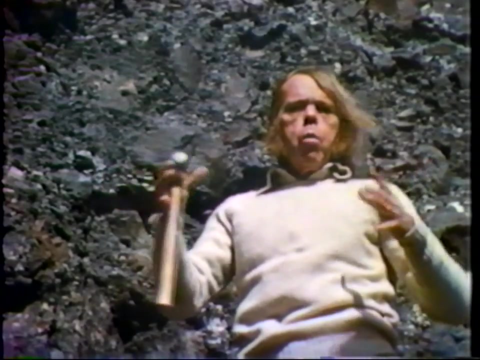 Now if you want further evidence of volcanism, just a short distance from here there is a place where lava has come from, From a vent not unlike this, into seawater. On contact with the cold seawater, it has broken into bulbous, pillow-like masses which 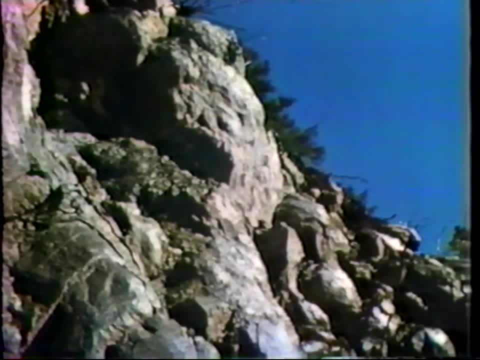 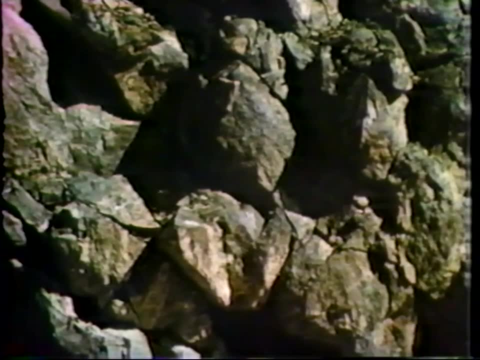 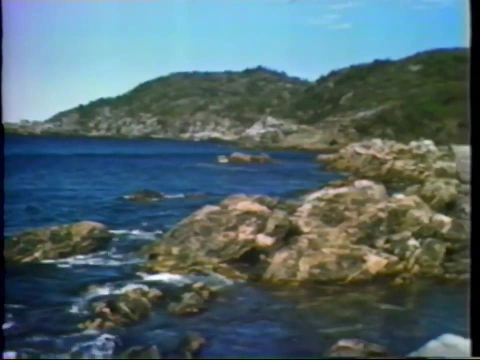 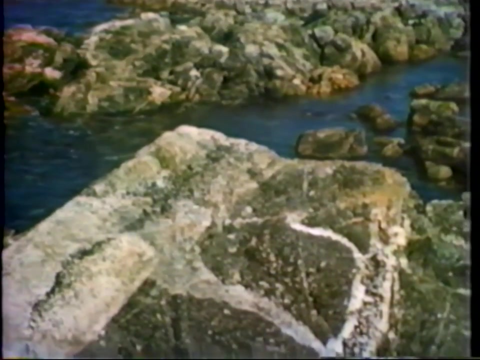 move out and pile one on top of another to form a rock called pillowed lava. If erosion destroys some of the evidence of volcanic activity, it also exposes the roots of these volcanoes. Maybe get a look at the plumbing of the system, if you like and can see where molten rock. 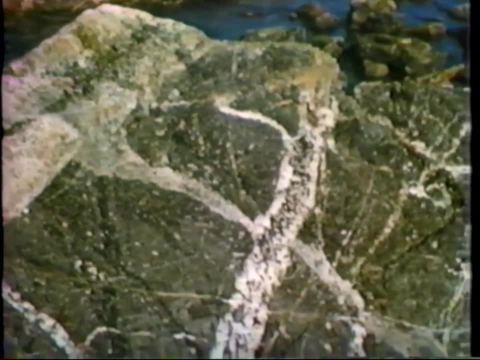 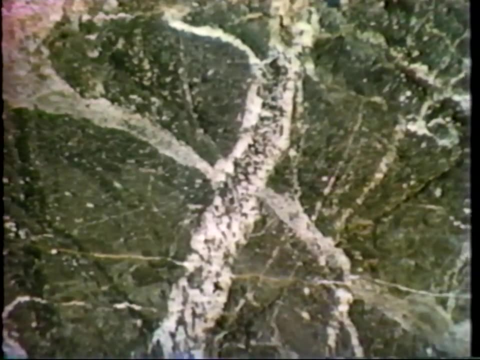 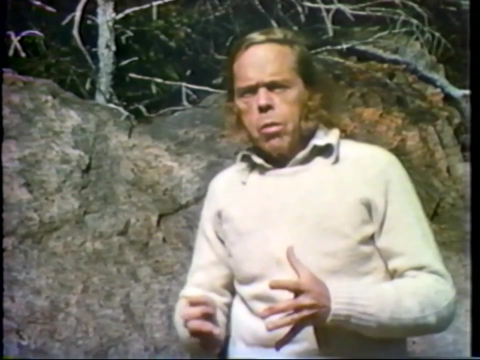 on the way to surface, crystallized or solidified at depth in cracks in the rocks. Now, at about the same time that this volcanic activity is taking place, to the west, there are some pretty impressive movements taking place in the earth's crust. Remember now. 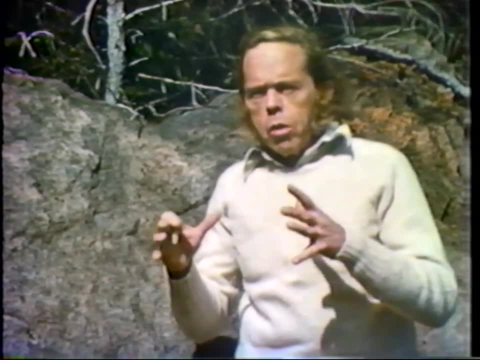 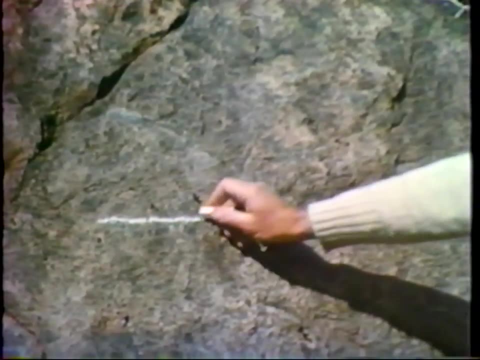 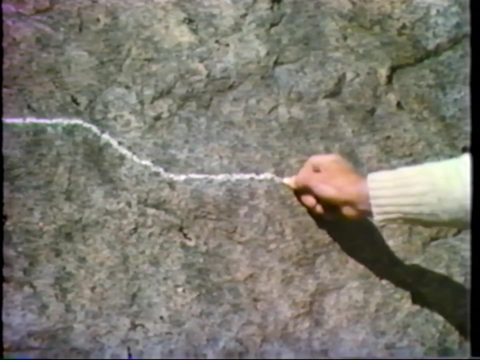 All through this process, the oceans, or the ancient ocean, is shrinking. The continents are moving together. Let's take a look. We have the continental shelf, the continental slope, draped in sediment, and the ocean floor which is being moved as a slab down into the earth's crust, underneath another slab of ocean. 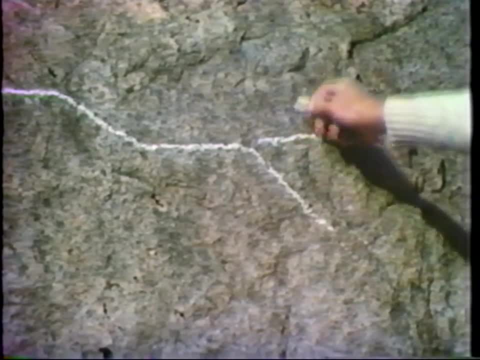 floor. Now, this is where the volcanic activity that we have seen takes place. 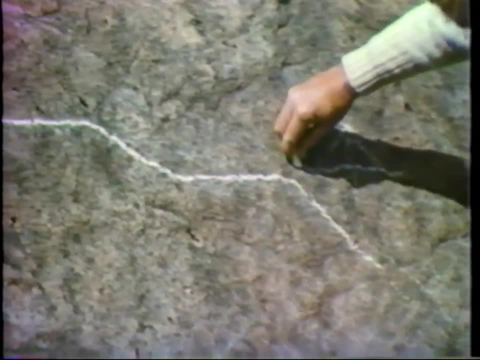 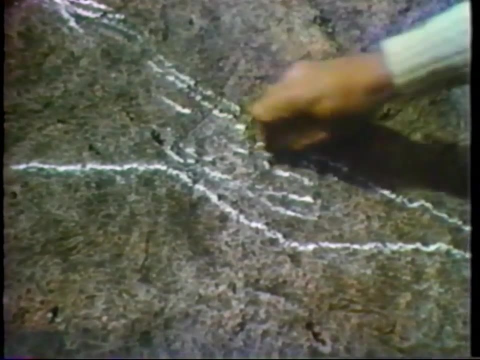 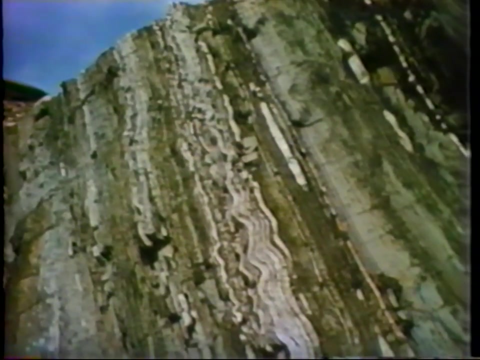 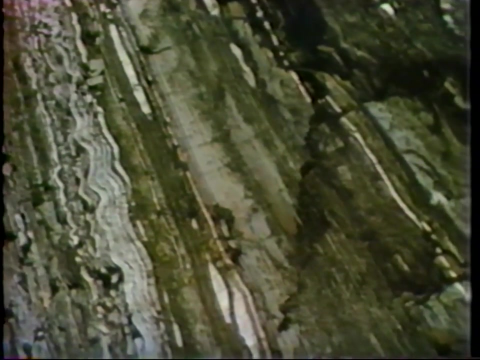 As the oceans shrink, this slab is moved right over the continental margin like so, taking with it sediments from the continental slope. In these sediments we can read a sort of shorthand history of the ancient sea. The gray layers are shales which were deposited in very quiet water. 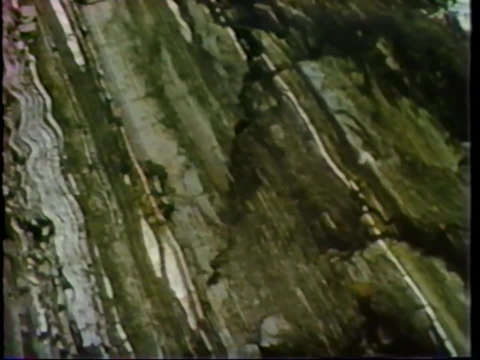 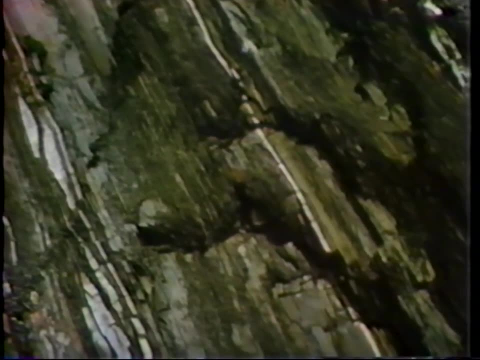 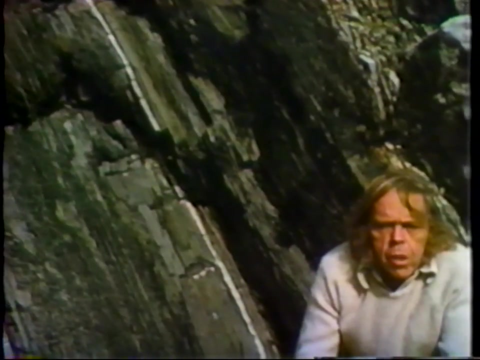 The white layers are sands which were on the continental slope and came streaming down that slope because of sort of underwater landslides, if you like, caused by maybe a violent storm, an earthquake. This process of sedimentation continued until the character of that ancient sea was really. 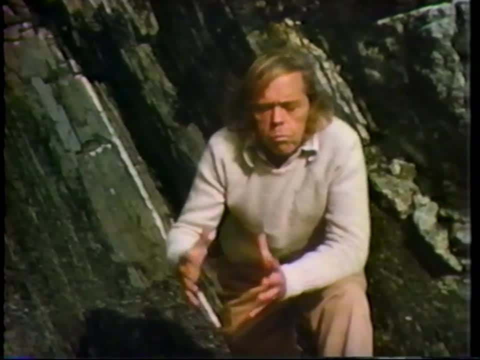 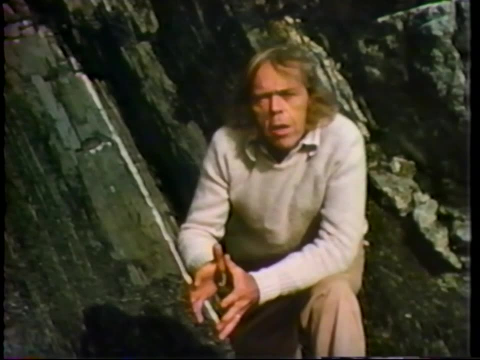 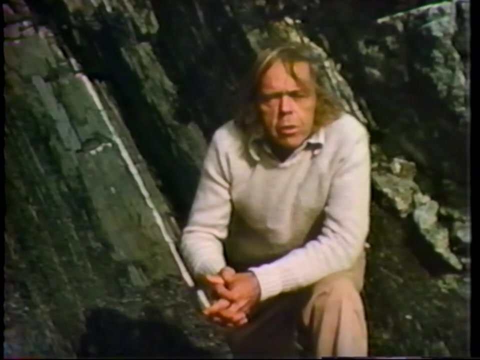 unalterably altered by the great earth movements that took place. These sediments were carried 50 miles from where they were deposited along with that slab of ocean floor. They're fairly well preserved and not too badly deformed because they were not caught. 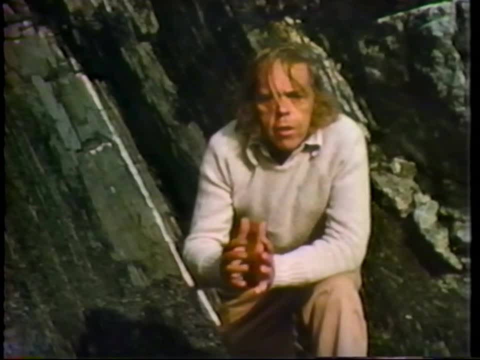 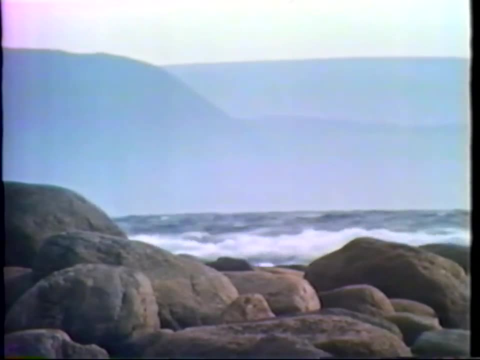 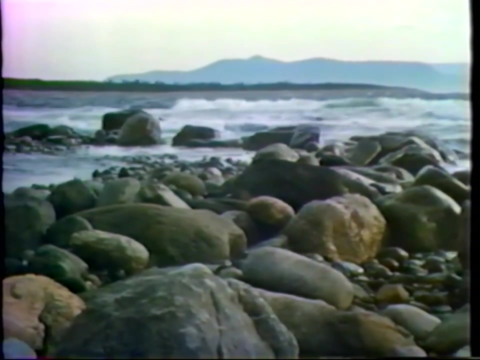 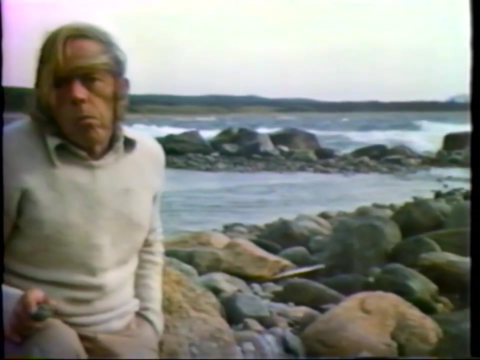 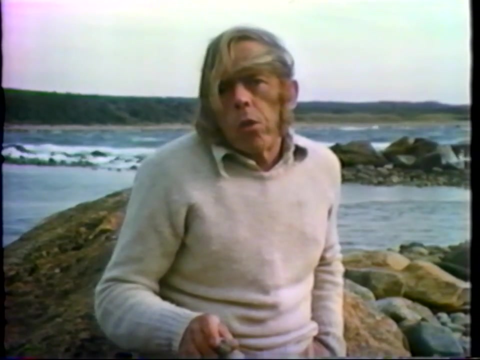 up in the vice of two colliding continents and therefore escaped the intense heat and pressures that existed there. Our seas contain a rich and varied life. Along any beach, you can see the shelly remains of such life. The ancient sea, 500 million years old or better, also contained life, maybe as rich. 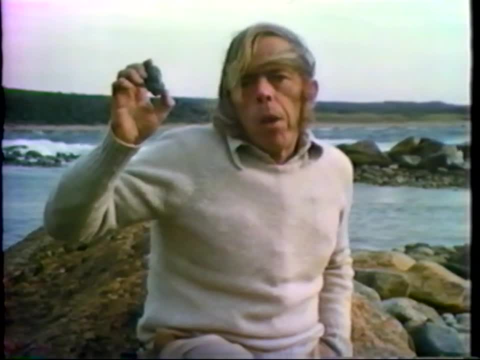 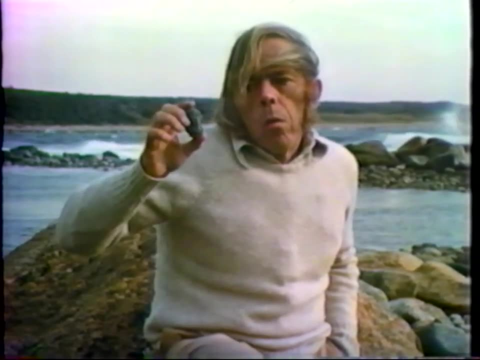 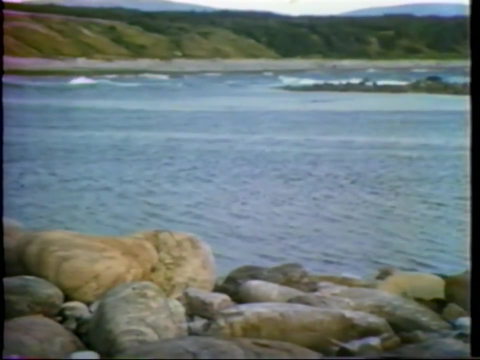 as ours, maybe not so varied. This bug is a trilobite and is part of the family that dominated the seas of those times. Well, they died, They became extinct, And their hard parts were preserved in sediments to become part of the geological record. 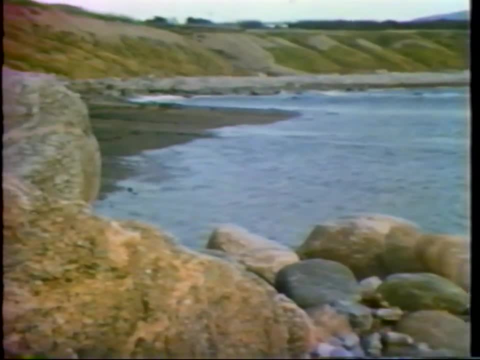 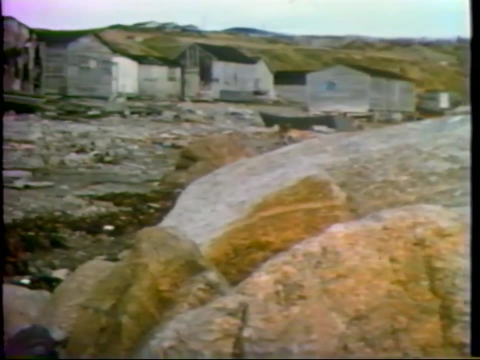 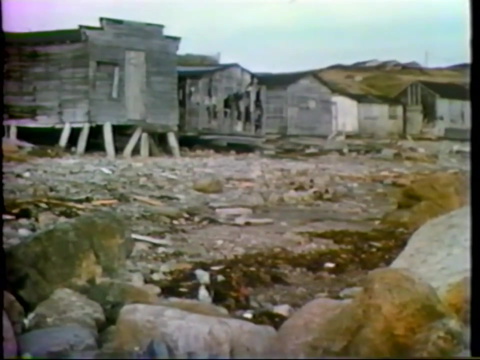 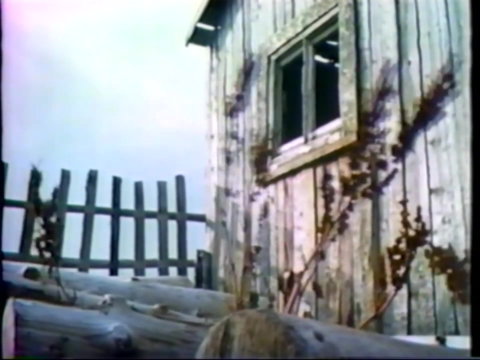 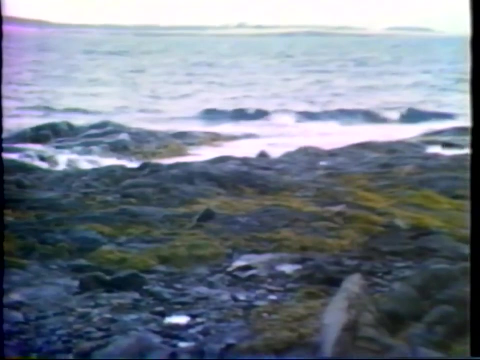 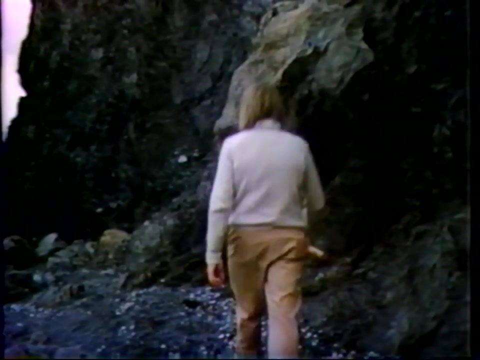 Well, man also has his record. This abandoned outport is, if you like, a fossil outport and is part of man's history. As the sea floor is moved over the continental margin, the rocks immediately underneath become really rather badly messed up. 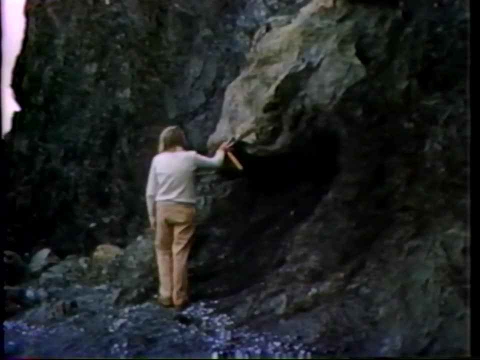 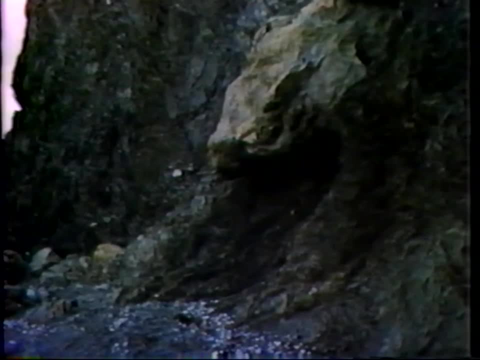 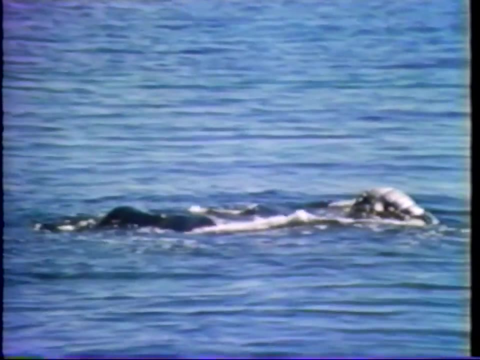 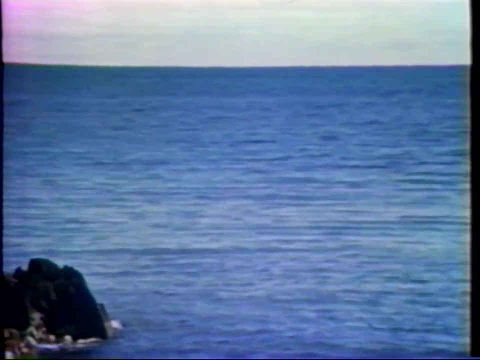 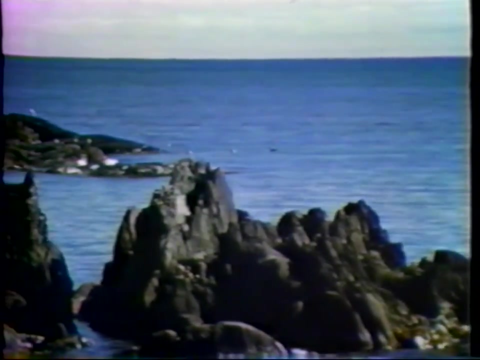 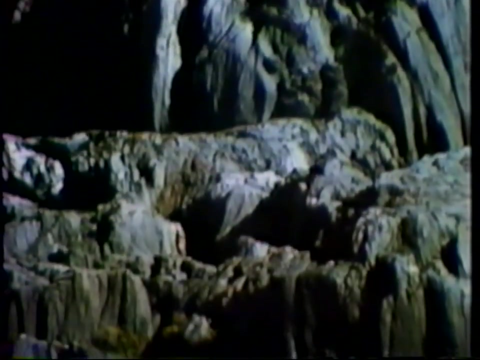 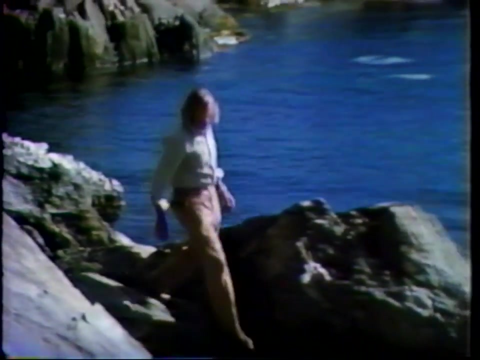 Shaley Rock. We're now in the heart of the Appalachian Mountains, or what was the Appalachian Mountain Range, where two continental margins came together. It's a very large area. Rocks caught between these margins were subjected to terrible pressures, as if caught in a vice between these two. 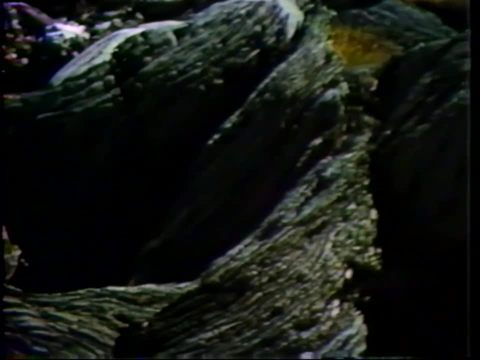 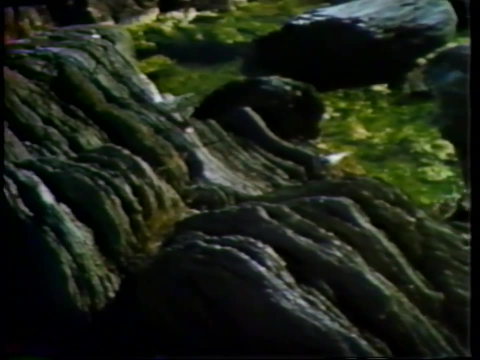 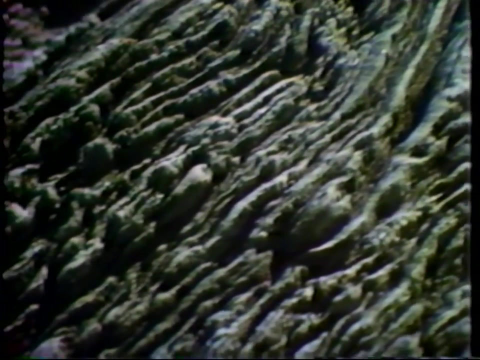 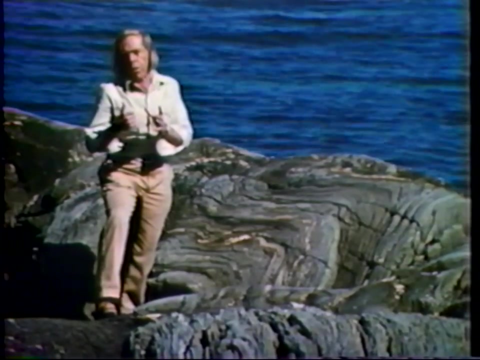 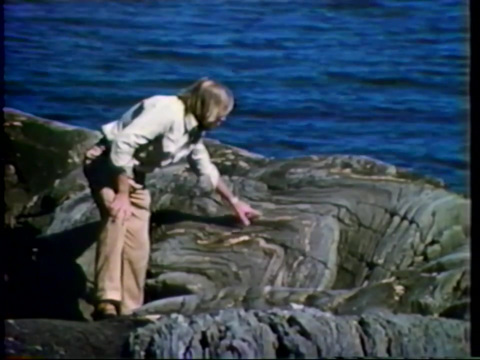 crunching continental margins. The contortions and folds in the rocks really are evidence for the pressures that they have been subjected to. Now these rocks are the very ones that we saw at Green Point. We see here folds, contortions, quartz sweats. 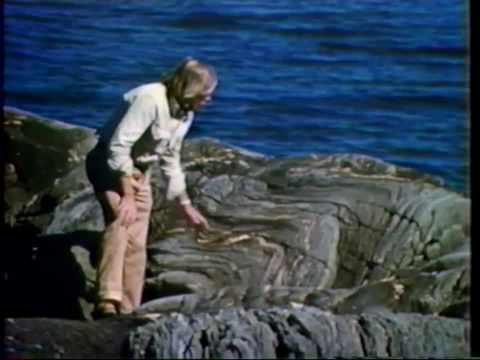 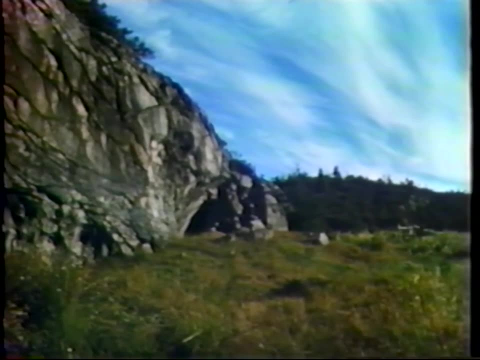 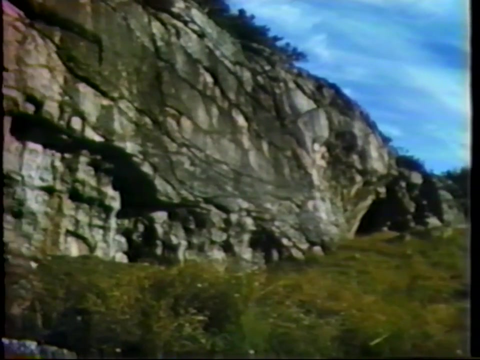 quartz being sweated out of the rocks during the folding, which are really miniatures of major broad structures which occur in this region. The seafloor also becomes involved And this deformation then becomes sheared and altered to give a rock with a peculiar blocky structure. 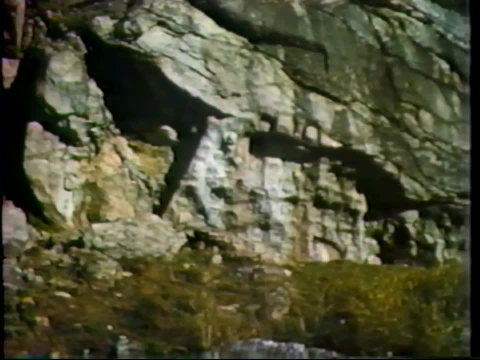 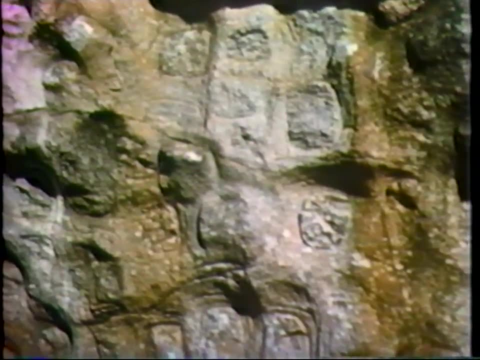 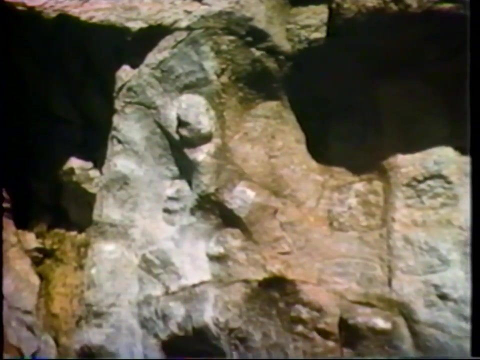 It has been said that early man carved these blocks from the rock. In fact, the rock is a soapstone And early man may have modified it by emphasizing its natural blocky structure. So we may have soapstone carving done by man and by nature. 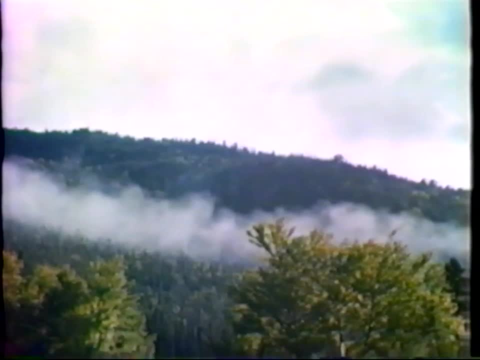 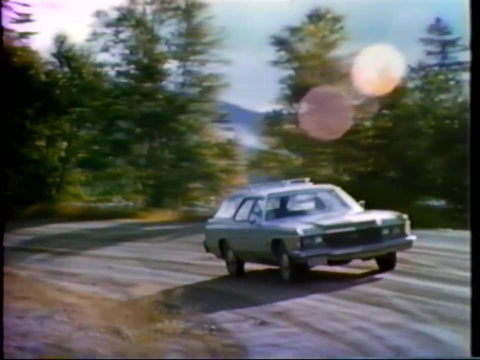 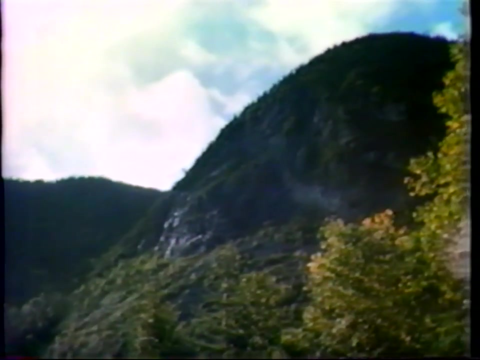 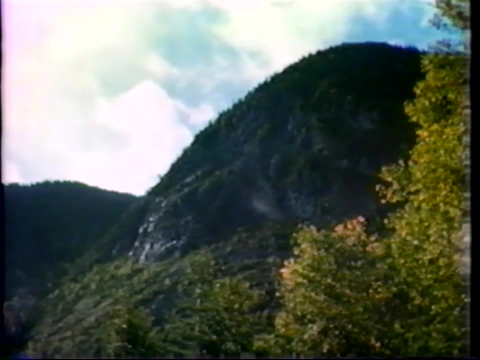 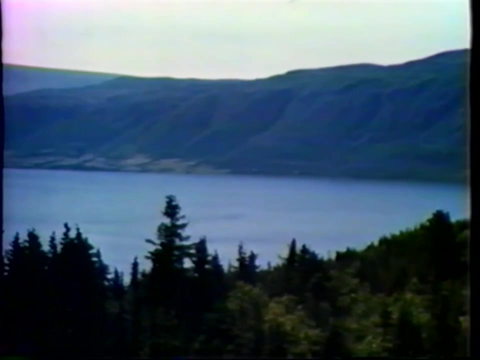 The work of the. Now what happens as this process continues? Well, as the continents get close to each other, things become more complicated. Instead of one sinking slab, there may be two or three, And they may move into the Earth's crust. 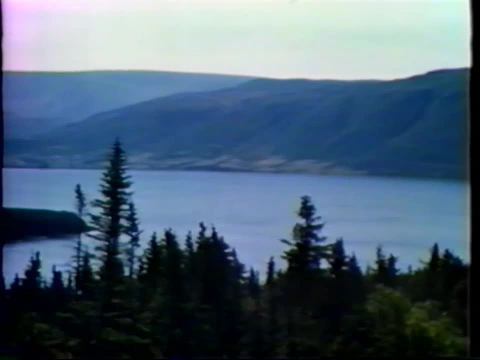 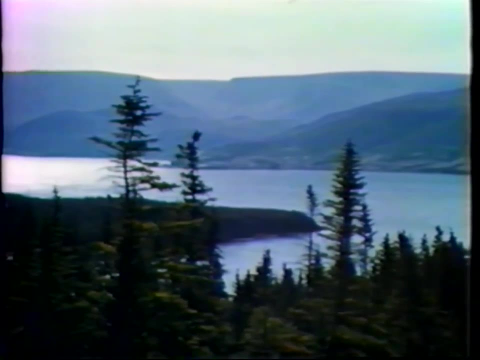 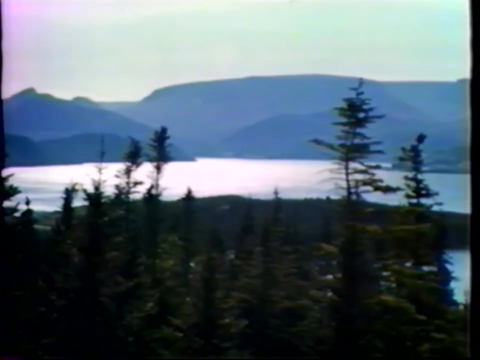 in different directions. They melt, so volcanism continues spasmodically, But as they sink into the crust, heat is generated, rock is melted and molten material moves towards surface and crystallizes, thereby thickening the crust from below, When the continents actually collide. 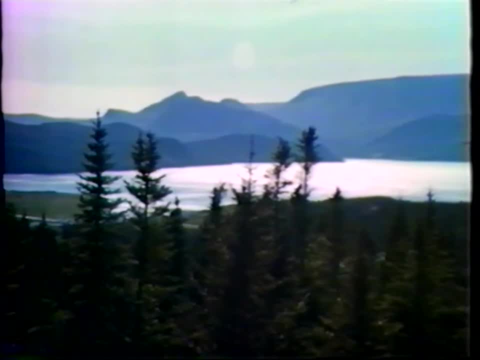 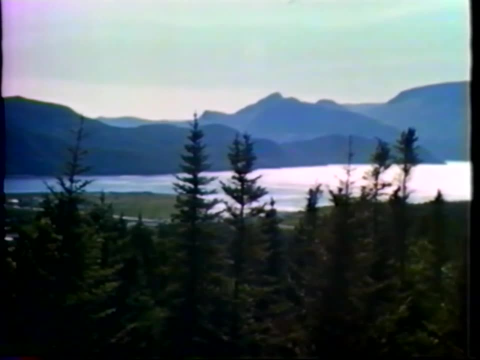 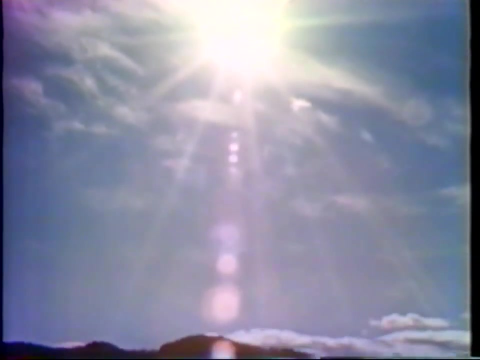 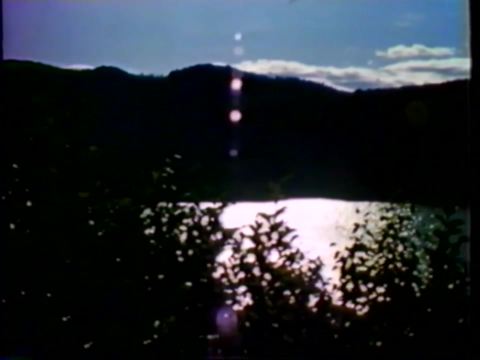 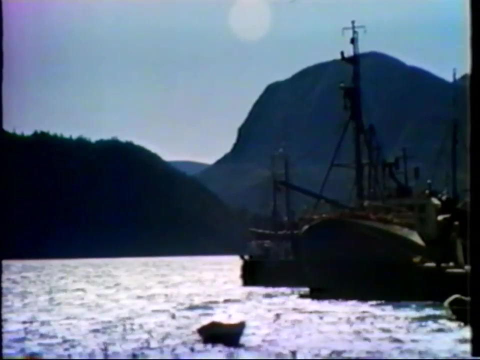 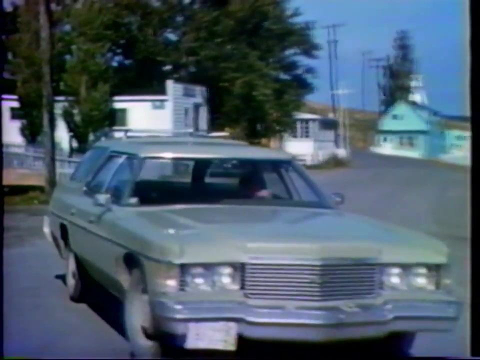 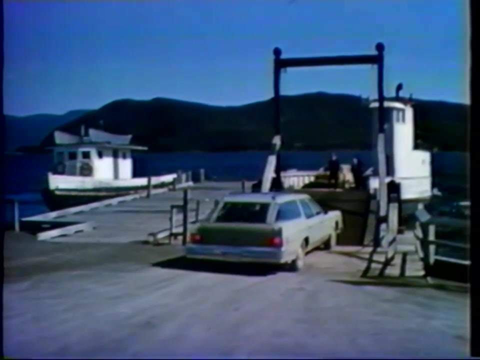 they intermesh or pile up on each other or under each other, forming a very thick crust. Sediments In the collision area become folded and are thrown into mountains, much like the Himalayan Mountains. Bściegsan, Bściegsan falls. explore the island of Donal. 726. 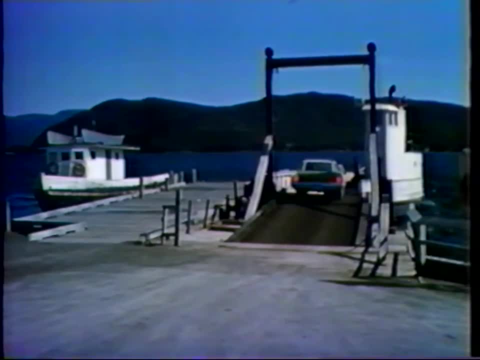 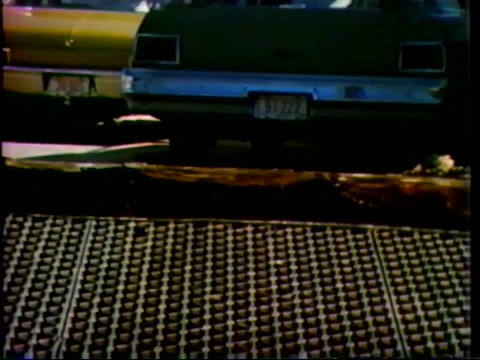 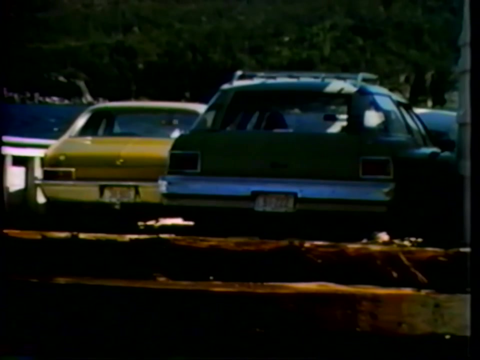 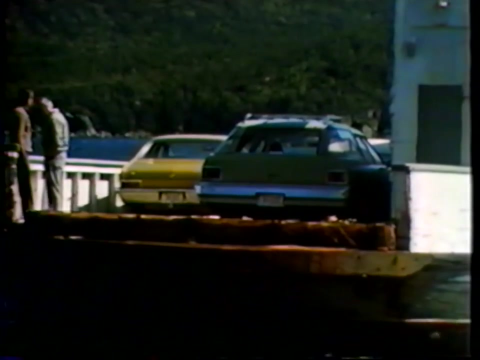 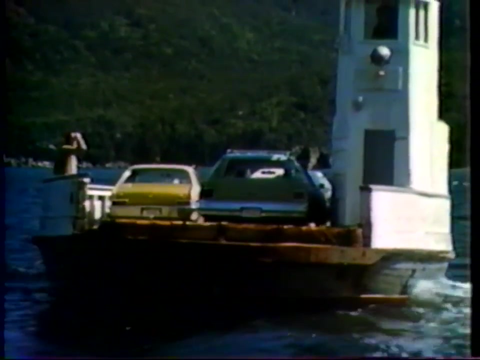 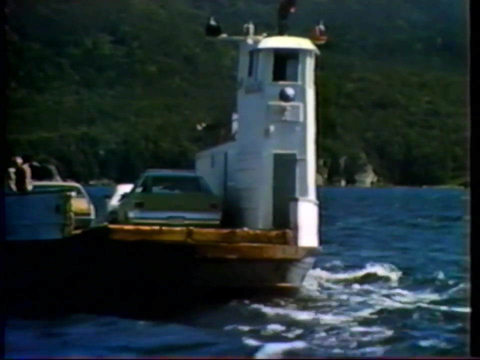 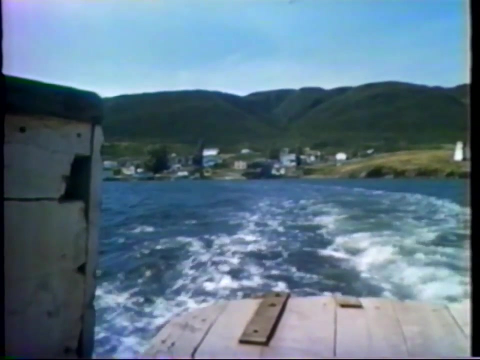 about one and a half kilometers away. It was once squared in two and a half miles to a mere hour, and about two or three miles and 20 miles to a mere hour and 10.7 seconds per minute, Bella, Oh my God. 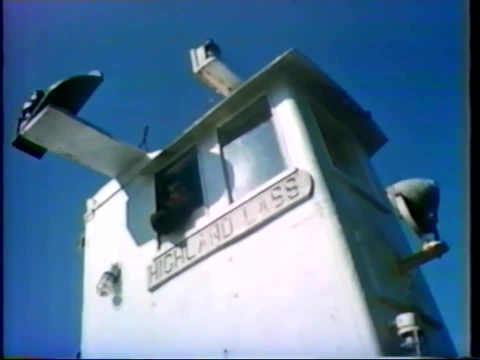 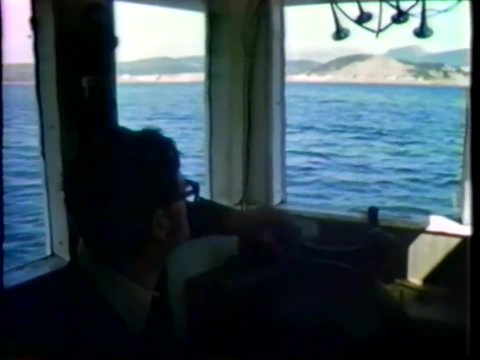 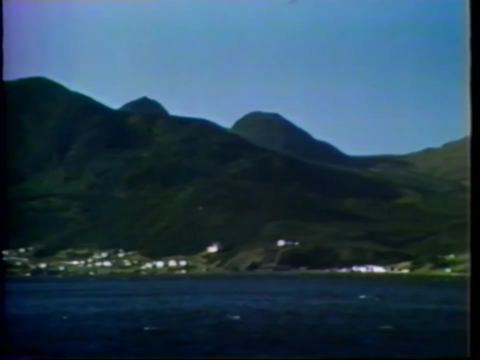 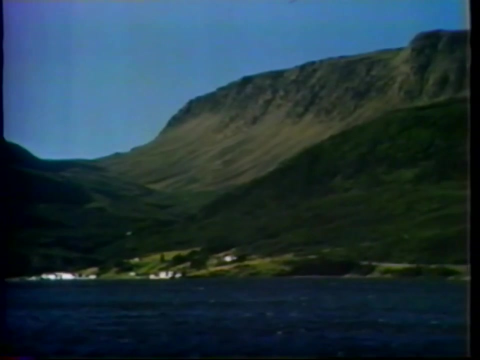 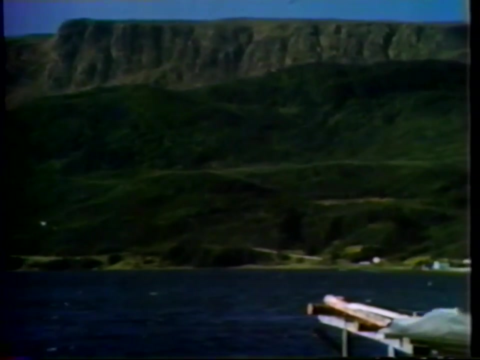 Oh my God, It's important to remember, I think, that these Earth movements take place very slowly, not rapidly at all. Things creep imperceptibly, At the rate of a few centimeters a year, or less than 100 feet per century. 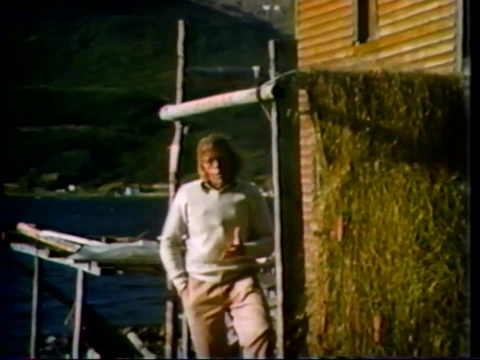 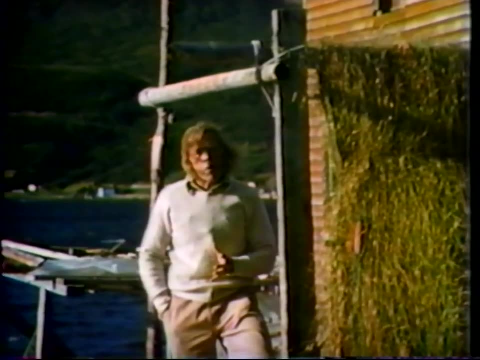 So we need time, and do we have it Well in Earth history? we're dealing with a planet that's 4,500 million years old. Now, that's a lot of time, And we sort of have to reset the clocks in our minds. 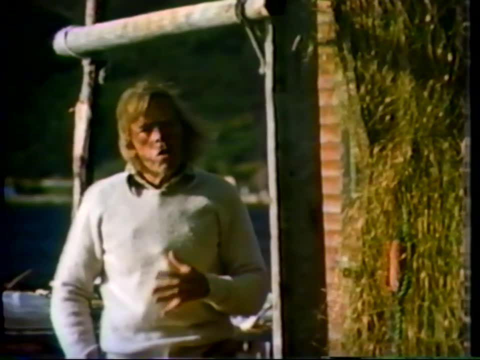 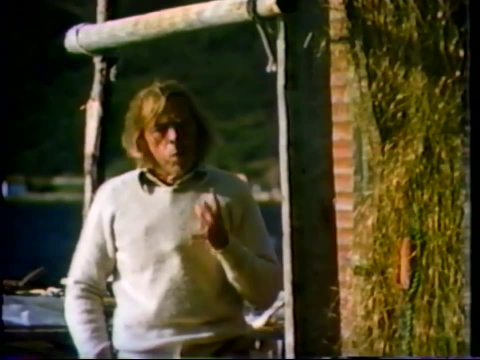 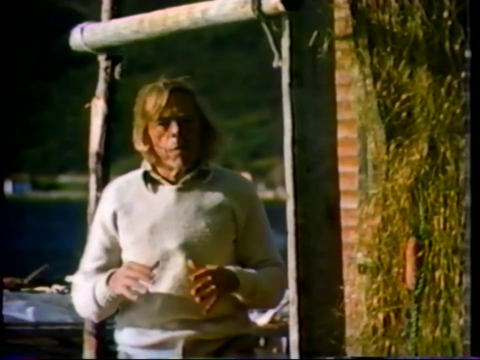 to that time frame, so that years become thousands of years, centuries become millions of years. That is a time frame we have to think in. So there is time for continents to creep imperceptibly together, for oceans to shrink or expand, for ocean floors to be moved up. 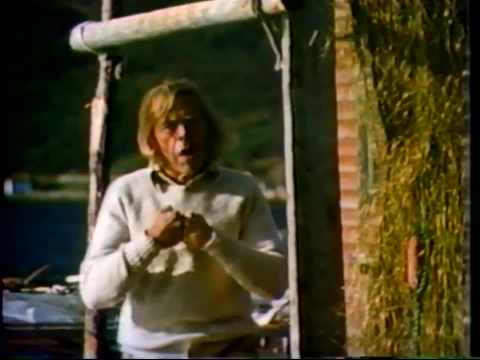 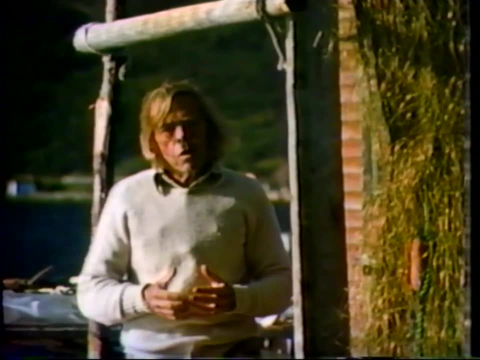 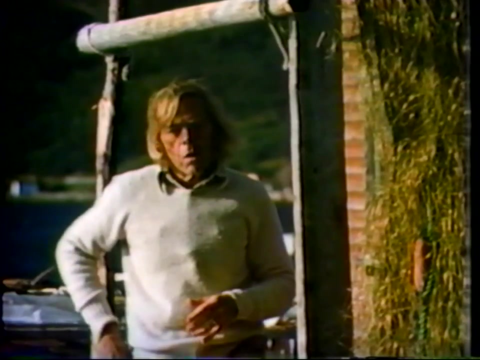 onto the continental margins, for continents to collide and throw up great mountain ranges. We have the time, but the process takes millions of years. This Earth simply was not built in six days and it never rests on the seventh, always moving. Now, if we have a problem with time, 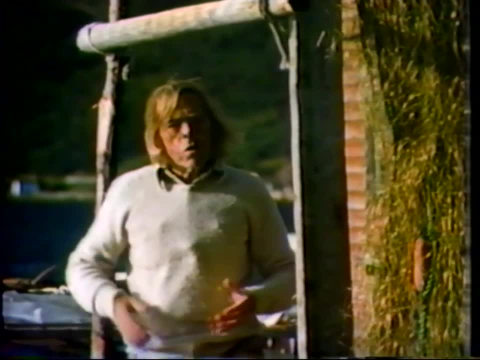 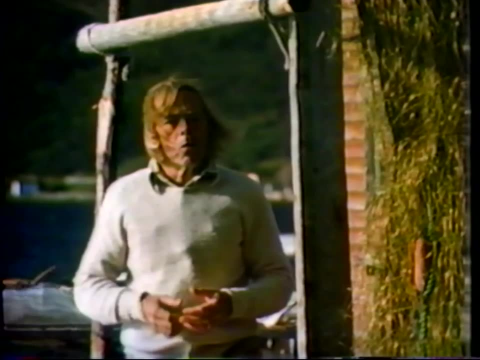 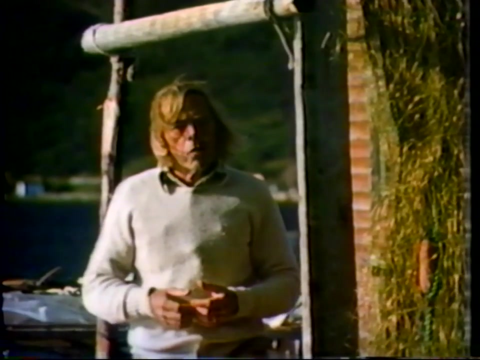 and think in terms of hours and days. we may question the whole process. Continents moving around bumping into each other, ocean floor being moved up onto land surfaces, continents colliding and throwing up mountain ranges sort of sounds like science fiction. 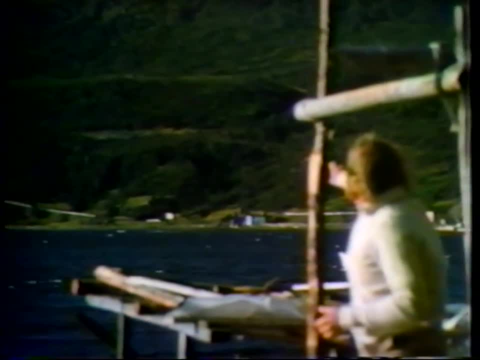 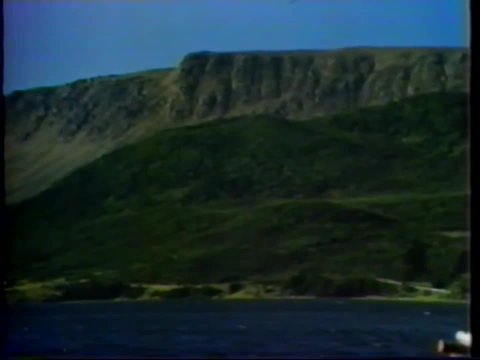 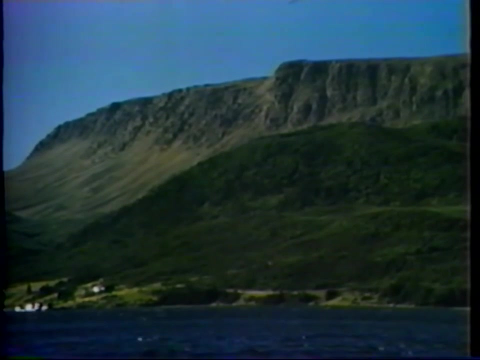 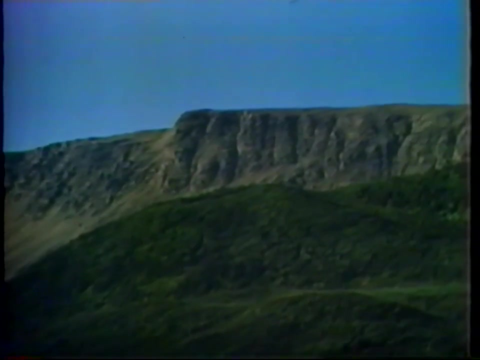 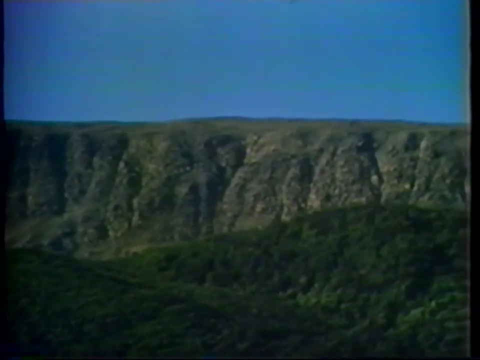 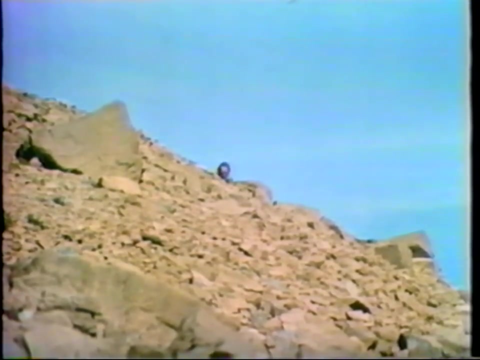 And yet that orange slab of rock there on top of Table Mountain moved 50 miles from its original position to where you see it now. Now, how else do you explain that kind of phenomenon? If you like, we can compare the sea floor to a sandwich. 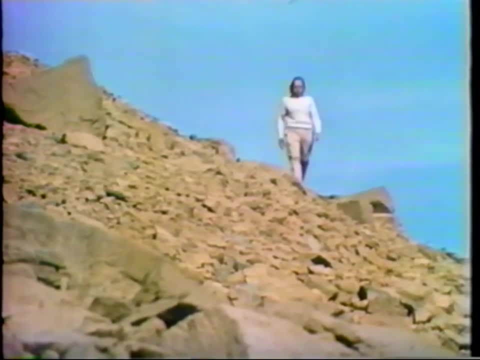 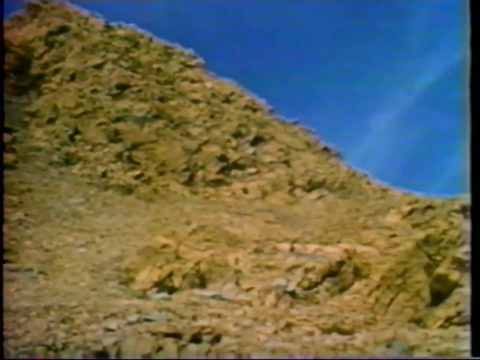 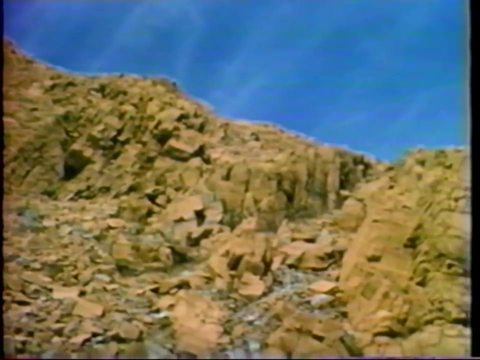 a thick sandwich because it consists of a number of layers of different kinds of rock. These rocks are the bottom slice of bread of that sandwich. There are mantle rocks from below the ocean floor. A few years ago, a lot of money and effort was spent. 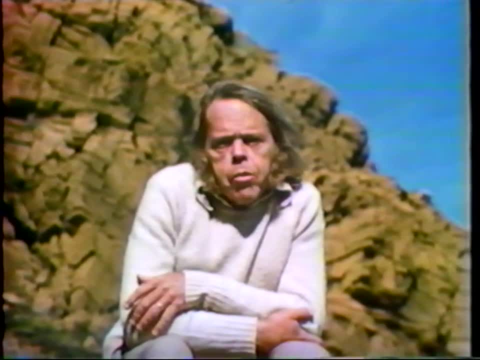 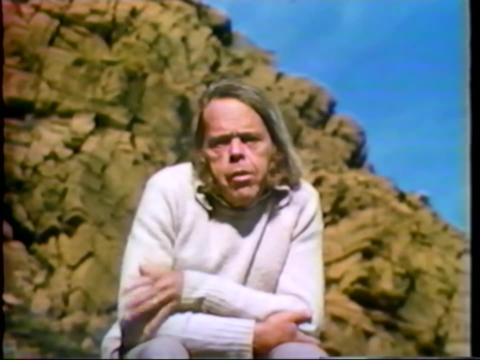 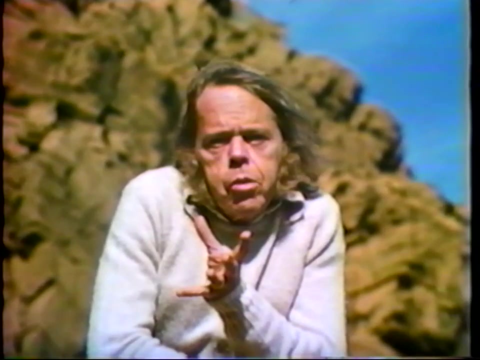 in an attempt to drill through the ocean floor to the mantle rocks below. It failed. It had to be abandoned. Here one can sample a mantle that's 500 million years old simply by knocking chunks of rock off a cliff face, And it turns out that the composition of the rocks 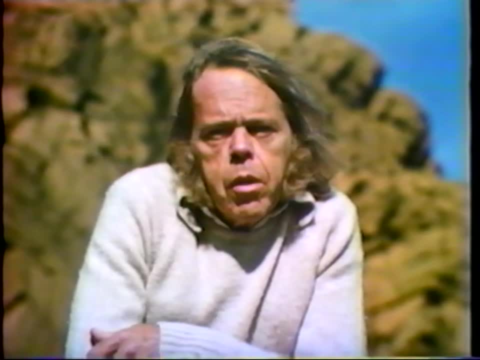 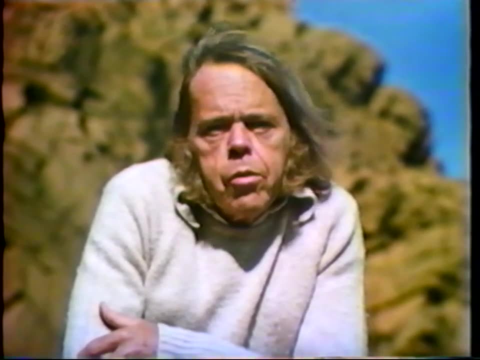 really haven't changed that much over a long time span. This is a barren, desolate, harsh place: No vegetation, Weird orangey-colored rocks, Almost a moonscape. Lack of vegetation is caused by toxic elements in the rocks. This is no place for man to live. 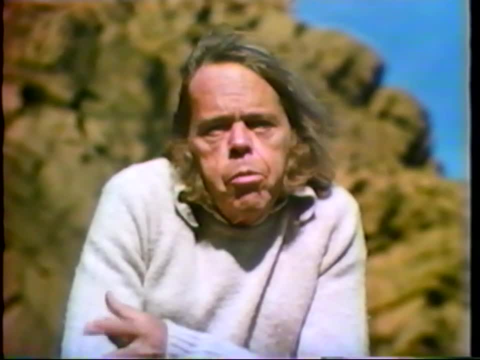 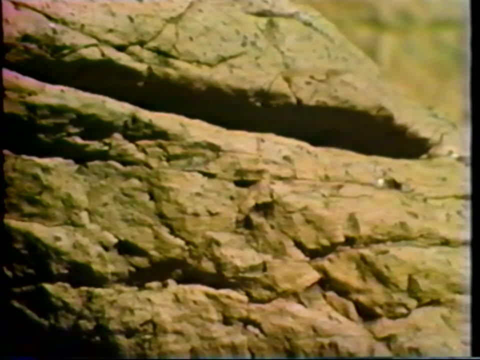 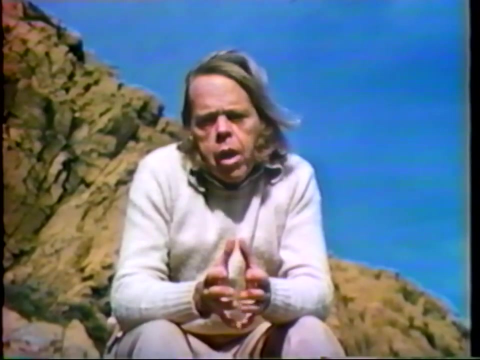 But then these rocks came from the sea floor. Man wasn't meant to live here. Now we tend to think of the ocean as a permanent thing. Landmass is permanent, And so on. And in our lifespan they are. Even in man's time on Earth they're permanent. 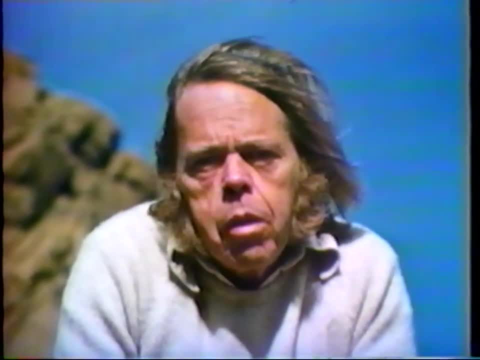 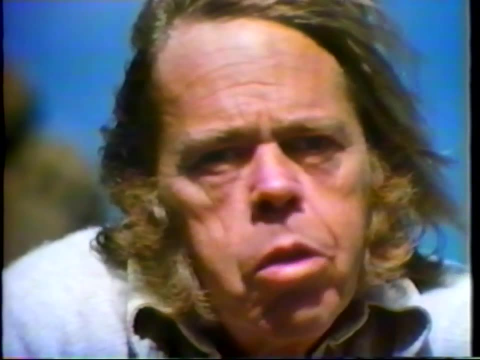 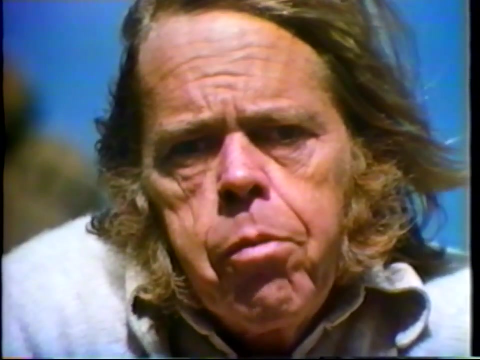 But in geological history, nothing is permanent. Everything is always moving. Today, the Mediterranean is closing, The Pacific is closing, But don't change your holiday plans. It will take a long time. So we study present properties and processes: ocean expansion, ocean shrinking. 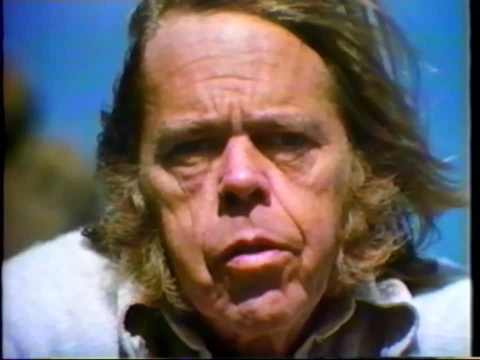 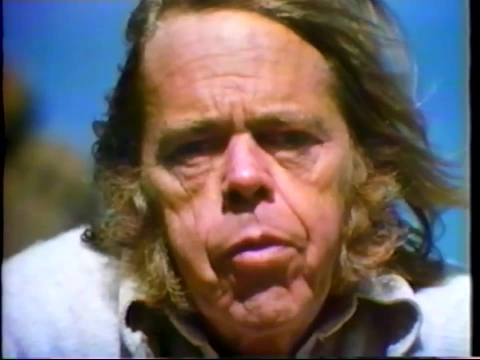 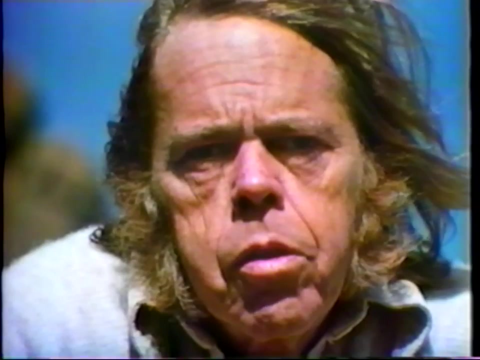 to learn how mountain ranges like the Appalachians get built. Looking at the remains of the Appalachians we really sort of see the shape of things to come. So the present informs the past and the past allows us to speculate about the future. 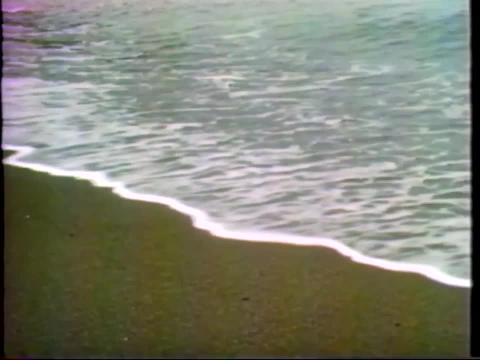 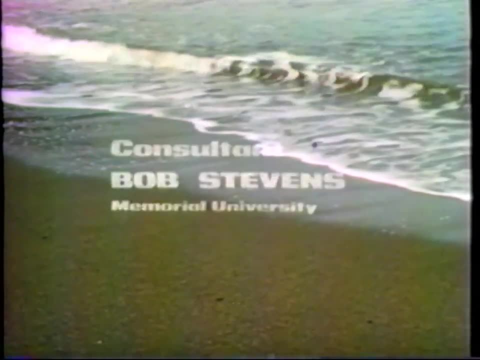 someday. we are on the orbit of the wealthy, of the rich, of the burden of wealth and of all his wealth, Like an old man or someone who's driven from his limo to his great-great-grandfather's house. 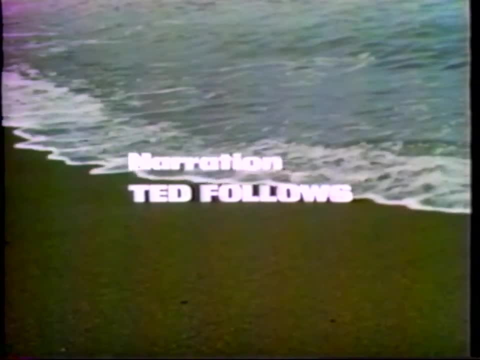 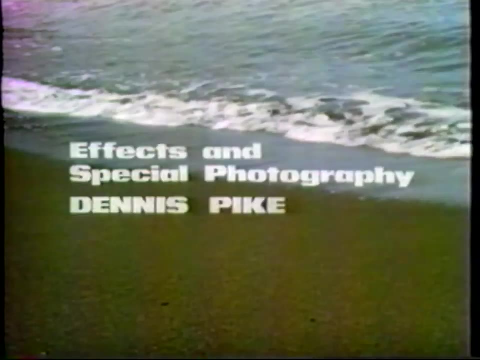 And it is now that cinnamon has come on, Thatbars has에 maybe come on and accepted that gentleman. But moving on, women's property still has arms And they're not just dirt, and p indexes and fastens the lines of that thing. 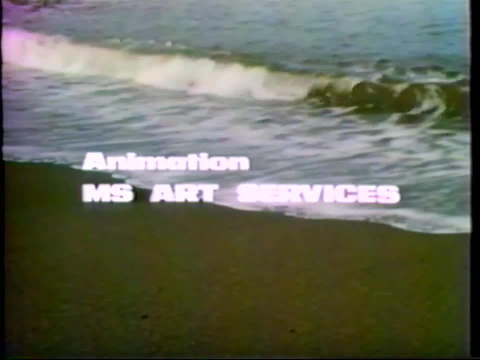 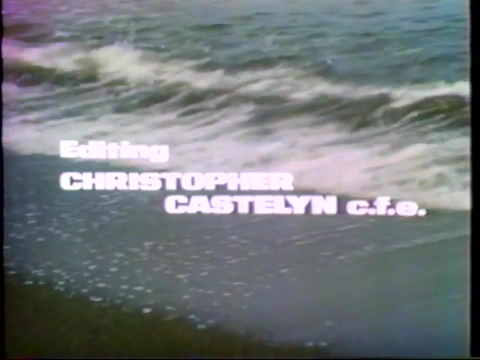 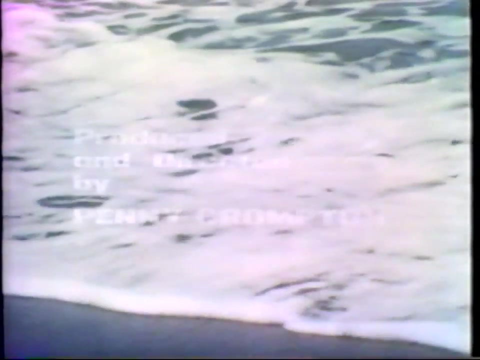 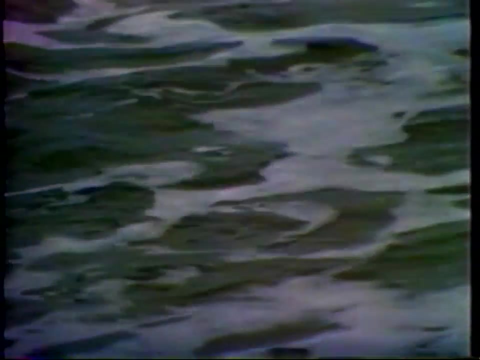 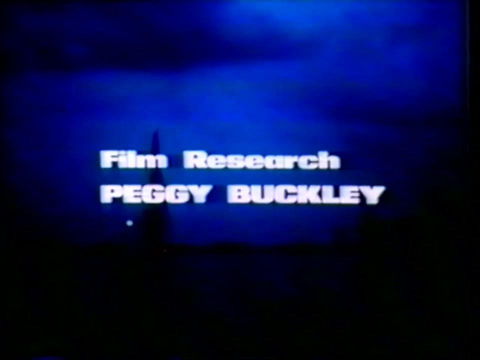 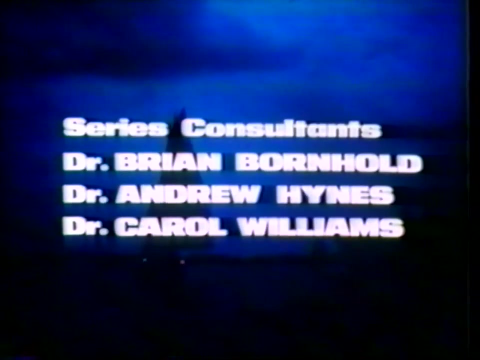 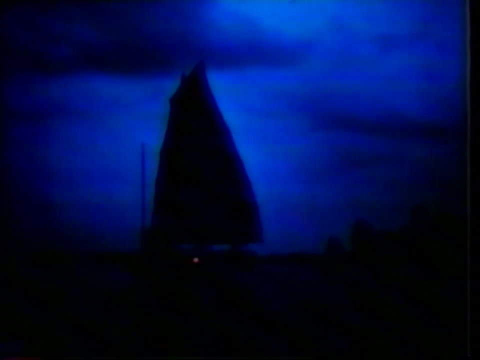 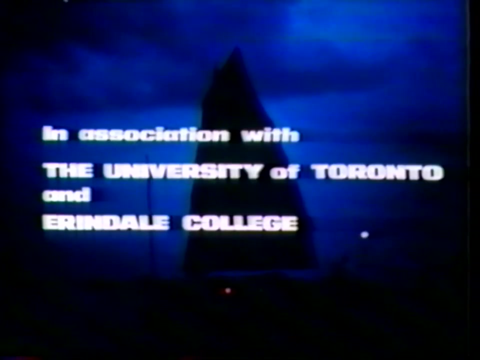 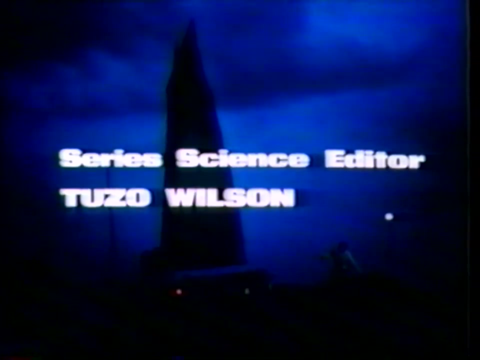 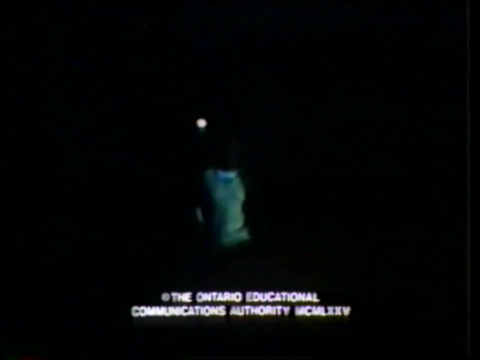 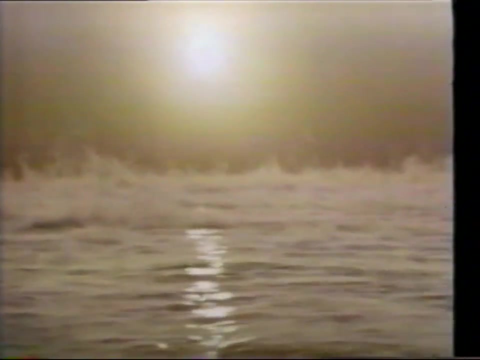 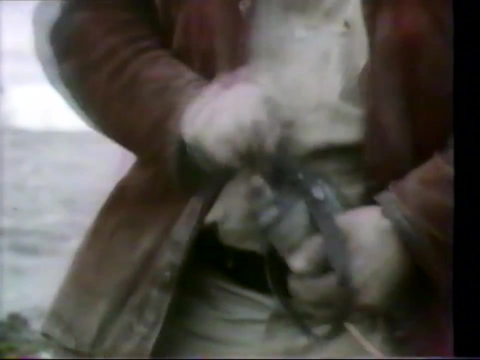 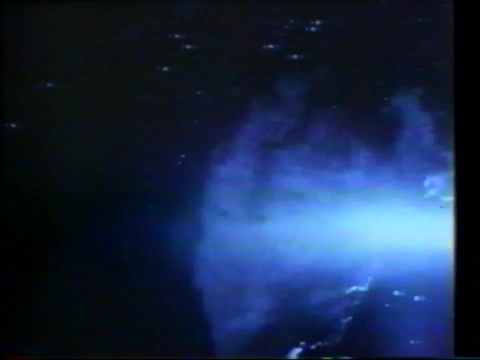 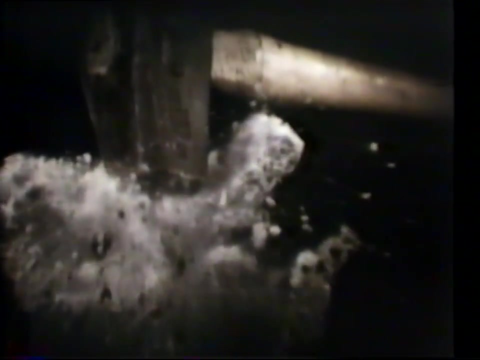 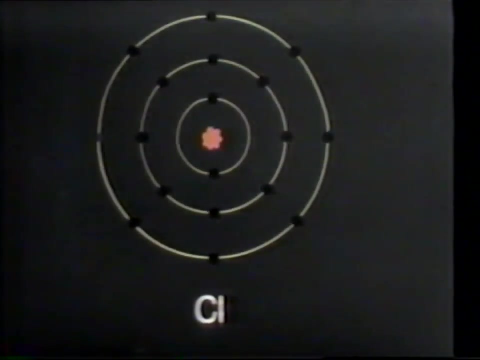 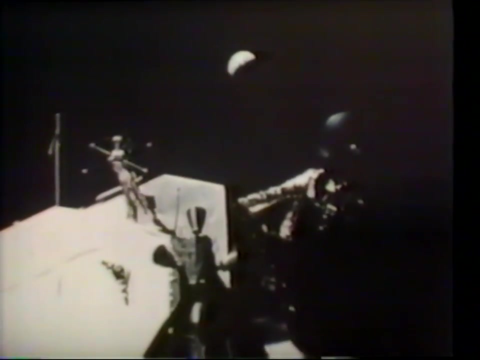 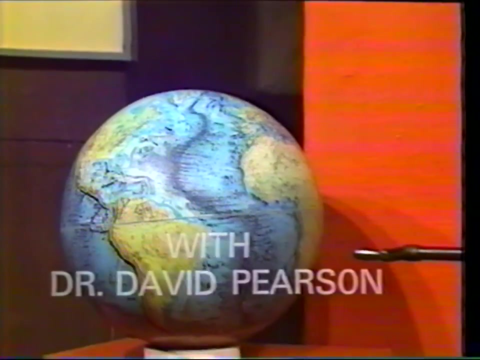 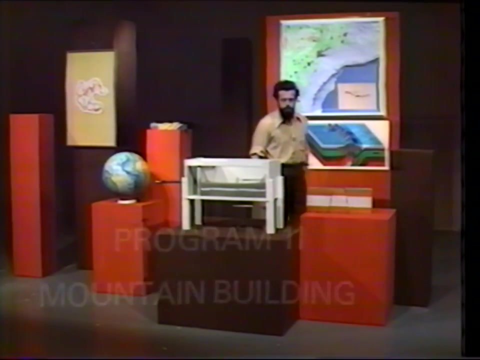 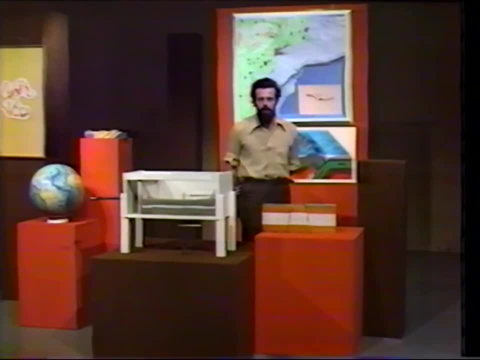 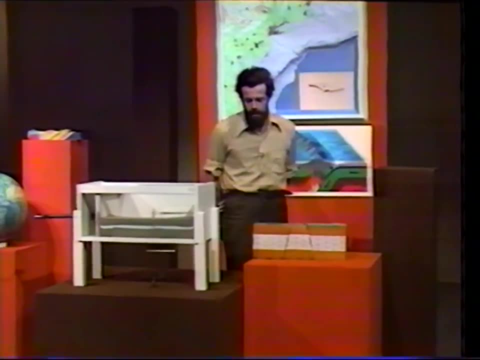 In the unit on plate tectonics we talked in generalities about the fact that mountain bolts occur at the boundaries of lithospheric plates. In this program we'll take mountain bolts a little farther and look at the characteristics of mountain bolts. 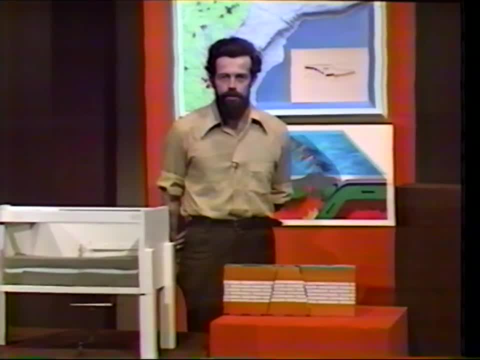 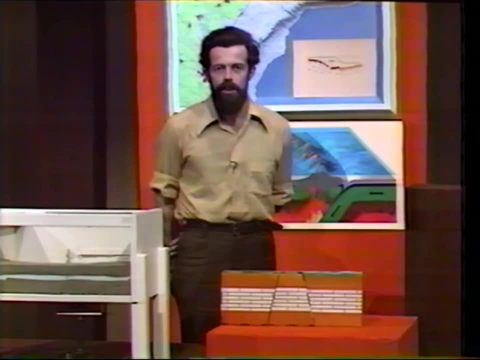 and the detail of the way in which they're produced at the boundaries of plates. There are several kinds of mountain bolts. There are those produced by the collision of plates, for example the Himalayas. There are those that are produced above subduction zones. 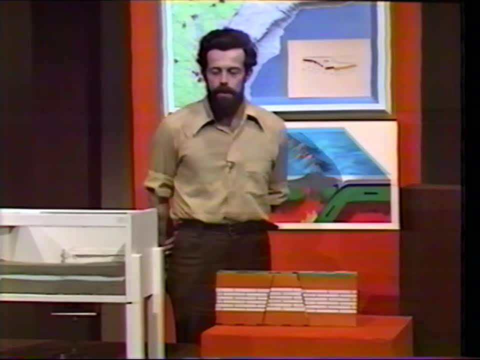 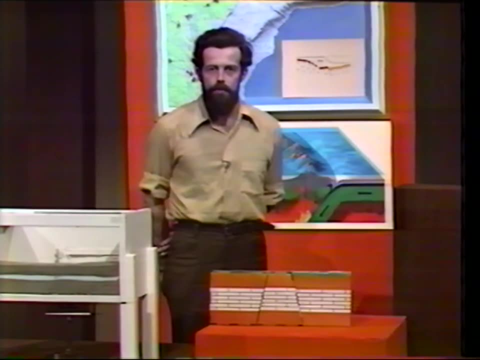 for example the Andes, And there are other types as well. We look at these different types and we'll take as our examples two Canadian mountain bolts: the Rockies and the Northern Appalachians as they occur in Nova Scotia and Newfoundland. 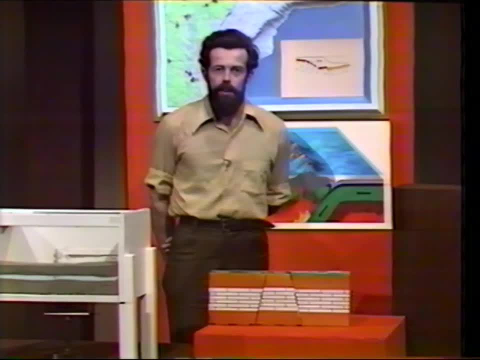 But we'll take a look at the different types of mountain bolts that occur at the boundaries of the plate tectonics. But before we get to the main part of our discussion of mountain bolts, let's remind ourselves of some other kinds of mountains that we've seen. 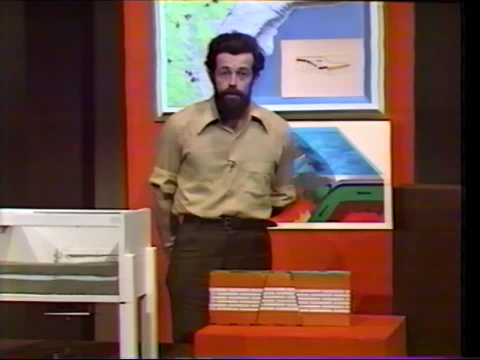 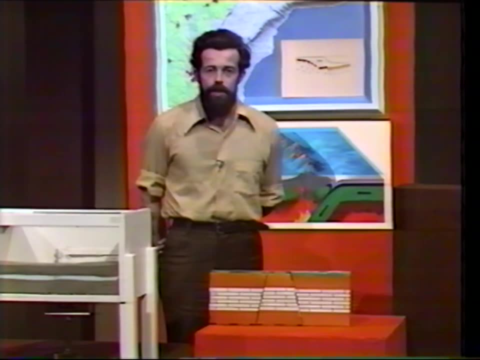 Volcanoes, for example, the Hawaiian Islands form mountain bolts. That's a string of islands on the ocean floor forming the Hawaiian chain. They're very, very high mountains, just the tip of them appearing above the sea level, But they're not a very important kind of mountain. 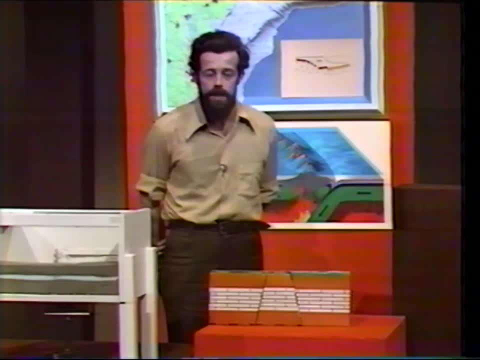 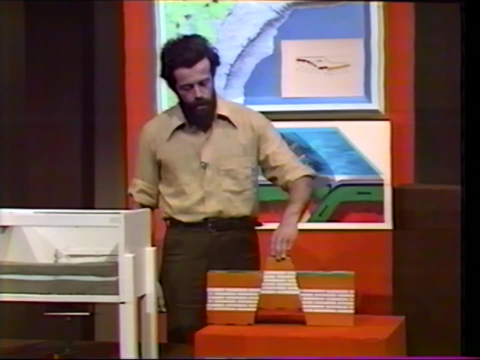 We don't see much of them. Most of them are on the ocean floor and hidden by water. Another kind of mountain that we've already looked at were the Horsts, the uplifted blocks bounded by two normal faults, that we also looked at when we talked of extension. 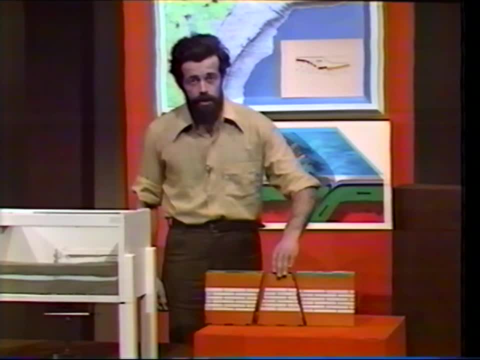 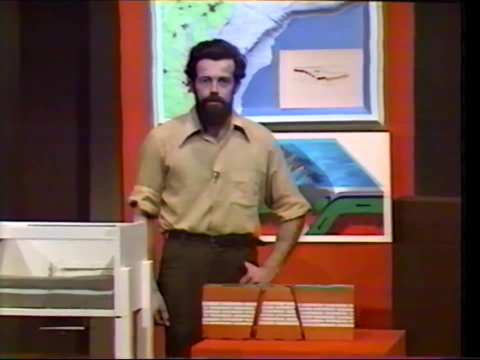 or tension of the Earth's crust and the kinds of forms and the kinds of faults it produced. But the main mountain ranges, the most important ones, are those which form great linear bolts across the ocean, And those are the ones that we're going to look at. 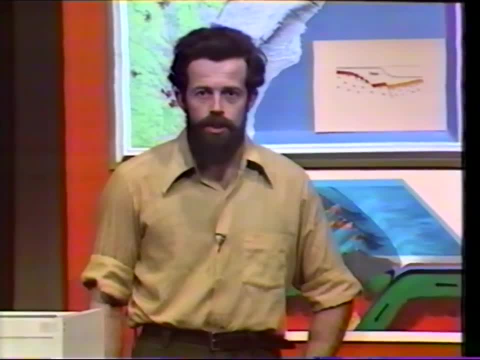 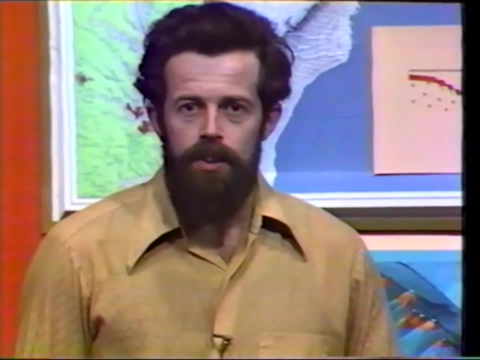 when we look at the Himalayas. the Himalayas, for example, the Rocky Mountains, the Ural Mountains, the Andes Mountains, and so forth, And it's these on which we'll concentrate our attention, Just to remind you of some of the features of a mountain. 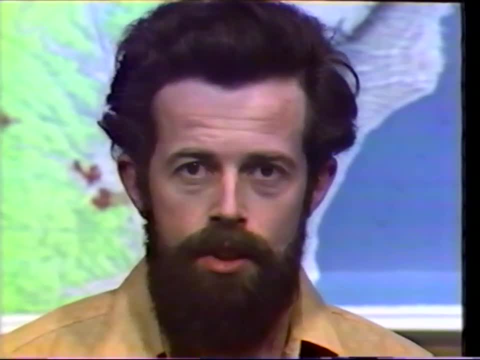 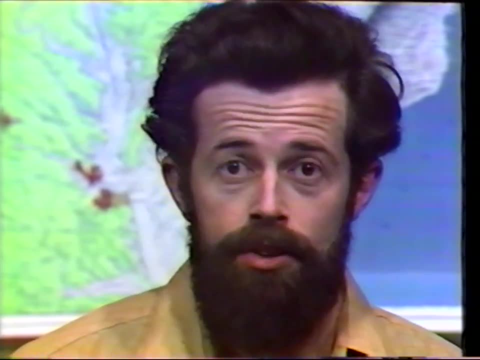 bolt that you have already looked at. let's look back again at the Rocky Mountains and look in particular this time not just at the way that the rocks are deformed, but what kind of rocks they are. Because if we're going to interpret mountain bolts- 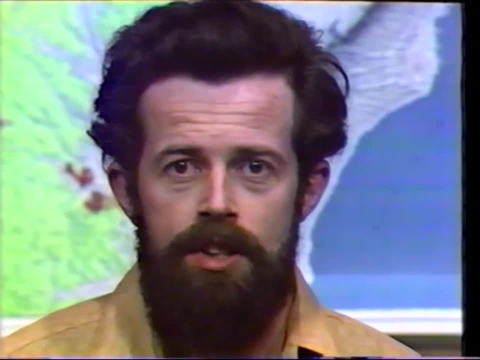 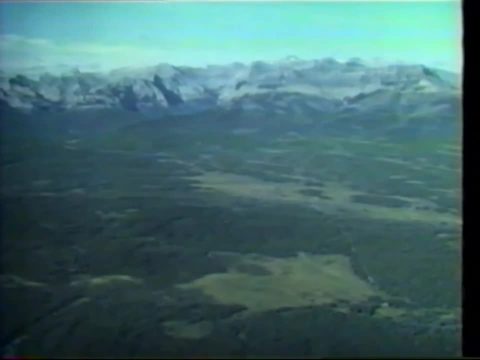 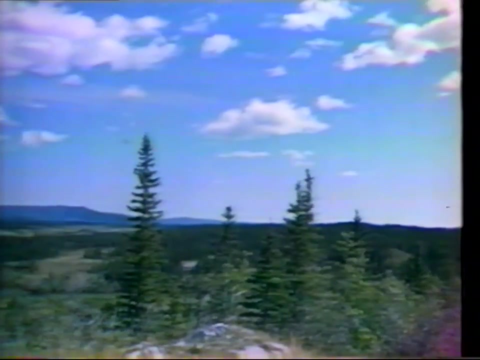 then we must start by understanding the conditions under which those rocks were deposited. The front of the Rocky Mountains, towering over the plains and rounded foothills to the west of Calgary, looks like a colossal limestone wall. In fact, it's built of overlapping slices of rock. 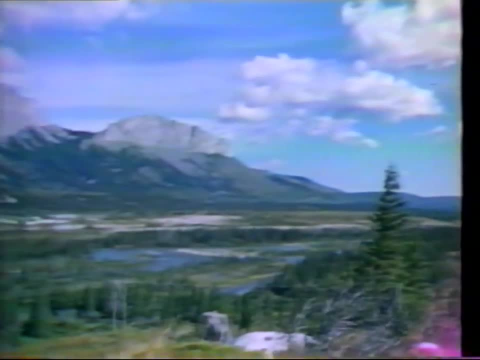 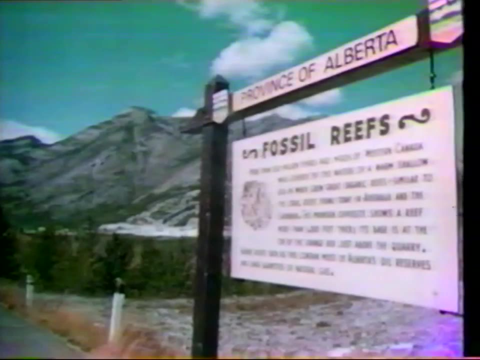 heaved into place from miles to the west along thrust faults such as this one beneath Mount Yamnuska. The fault follows the slope of the vegetation beneath the steep limestone cliff, Fossil-rich reef lines. the limestone is the rock of many of the giant thrust slices. 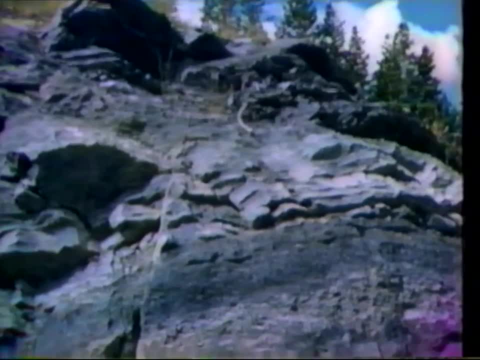 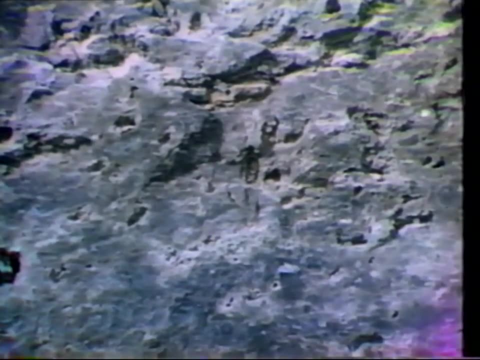 Some exposures, once rich in fossils, are now barren, their fossils having been dissolved by water seeping through the rock. Millions of the tiny cavities left form the reservoir for the great oil fields of western Canada. Many fossils are still, however, intact. 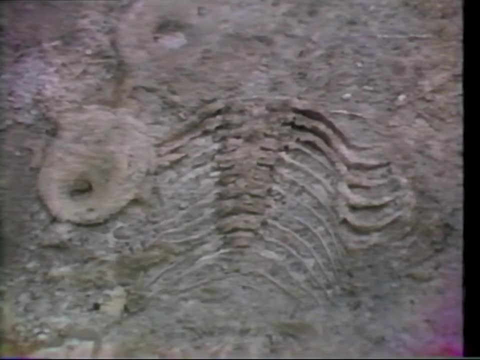 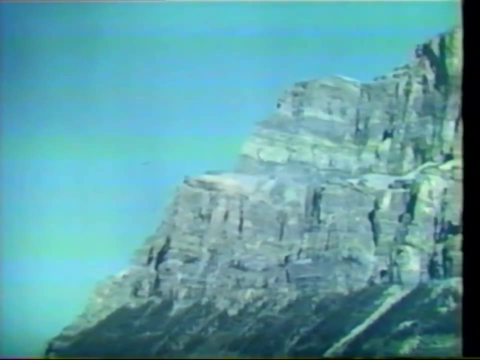 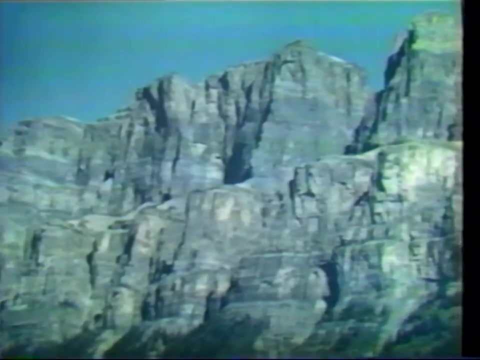 bearing witness to the warmth and richness of the seas in which the limestone was deposited. Mount Eisenhower is a sentinel of fossiliferous limestone, an eroded remnant of a once-continuous sheet now broken itself by a diagonal thrust fault dividing it into a higher and a lower slice. 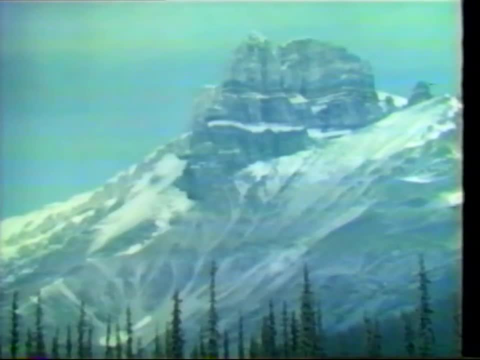 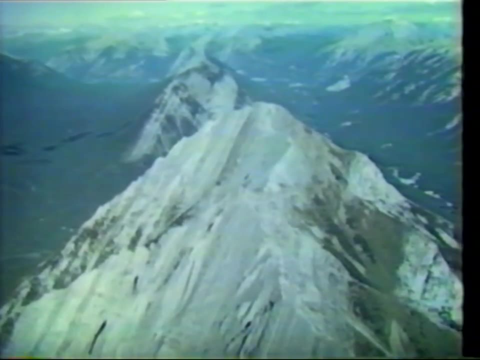 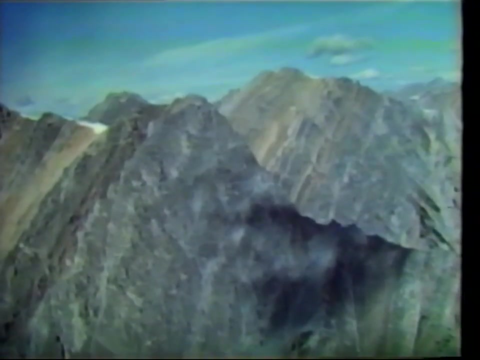 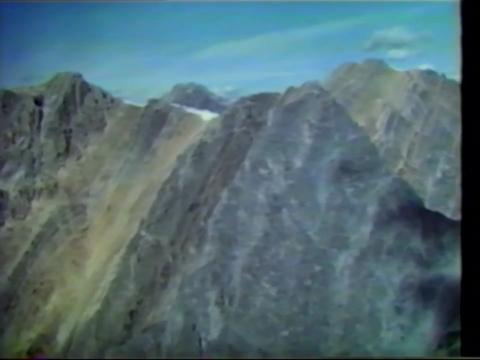 Mount Balfour is another piece of thrust limestone. The upturned edges of some of the thrust slices form distinctive blocky limestone ranges. The upturned edges of more shaly strata produce mountains of a slightly different character, somewhat more rounded, but still very rugged. 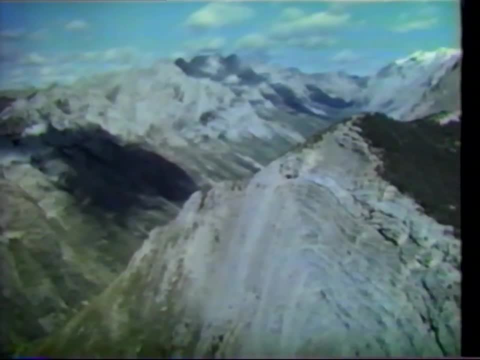 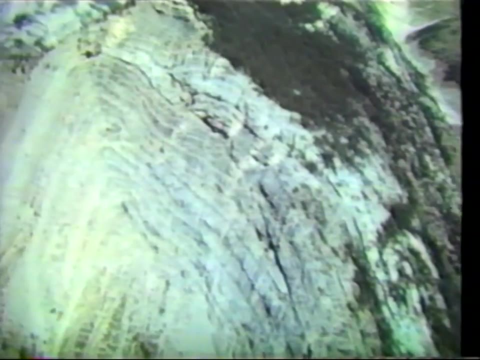 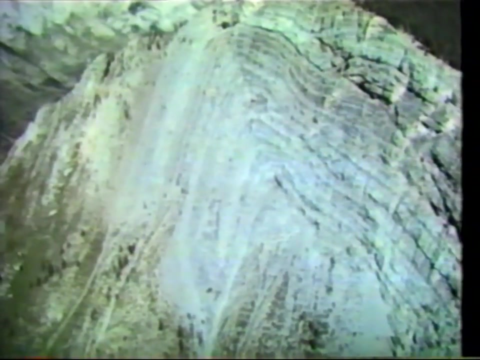 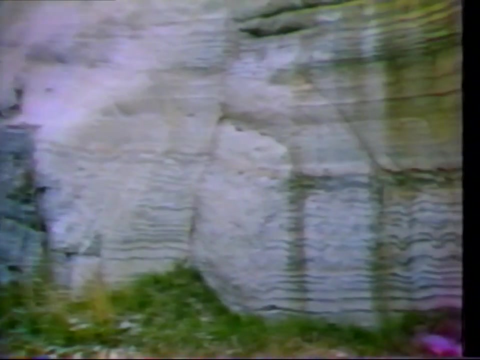 Folding as well as thrust faulting, is often beautifully visible in some of the vertical faces. These strata have reacted somewhat plastically to the deforming mountain building, and the forces Folds in the limestone also occur on a somewhat smaller scale. 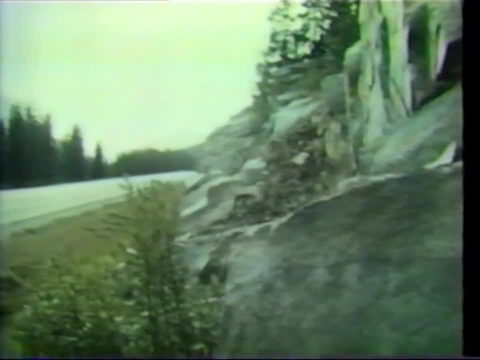 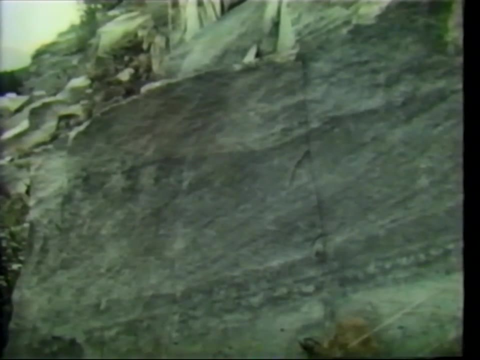 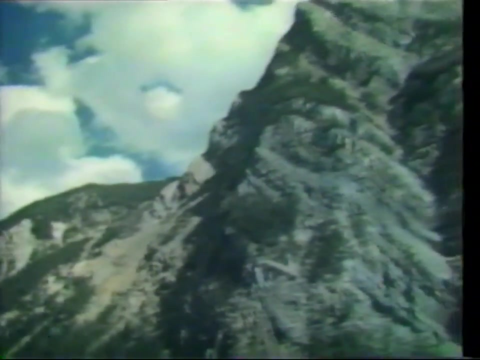 In sandstones, in some of the thrust slices, cross bedding gives an indication of the direction in which the sand was brought, the cross bedding indicating the current direction. Within the mountain bolt there's a quite sudden change in rock type from limestone to shale. 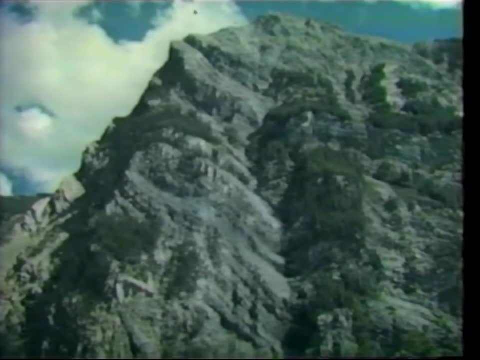 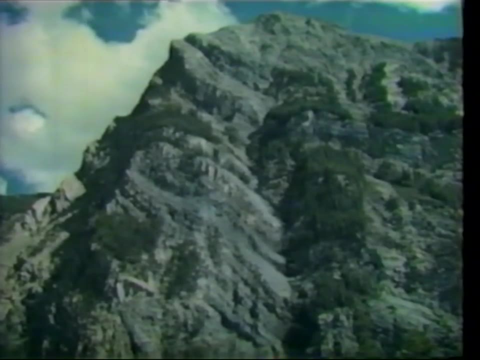 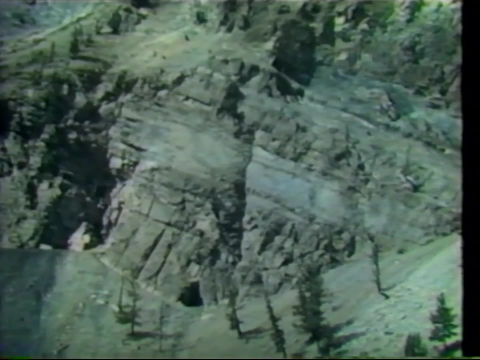 This is an important change for interpreting the origin of mountain bolts and also an important transition for mining geologists, since deposits of lead and zinc, such as reached by the small adits in this cliff, commonly occur at this junction. In fact, the deposits are in reefs, limestone nodules. 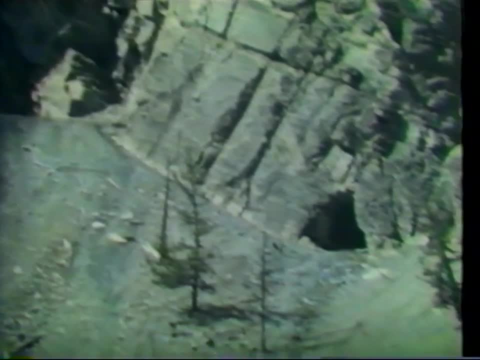 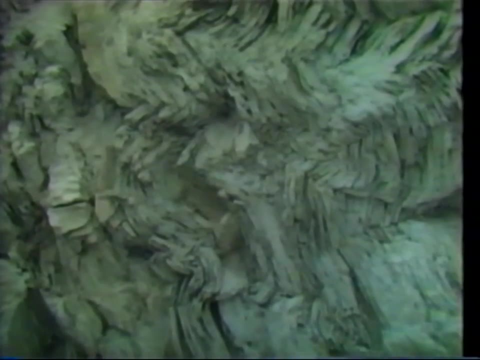 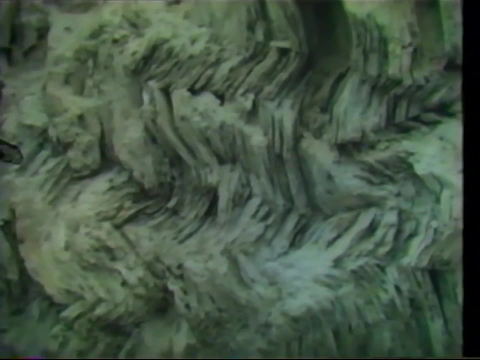 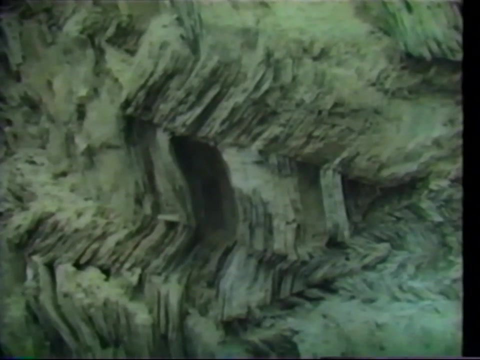 So limestone beds in the shale Shaley strata react in a distinctive fashion to the compressive mountain building forces. In this case sharp kink folds are formed, a type of deformation of rather brittle character, Passing to the west beyond the shale. 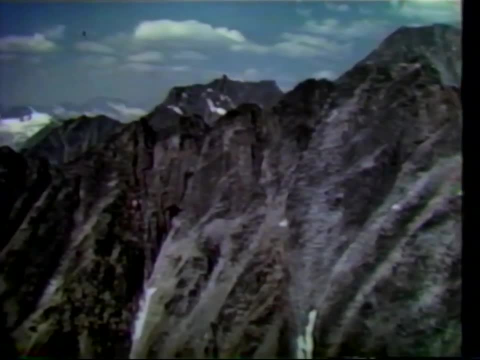 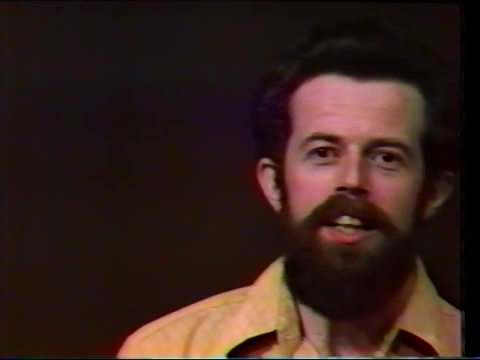 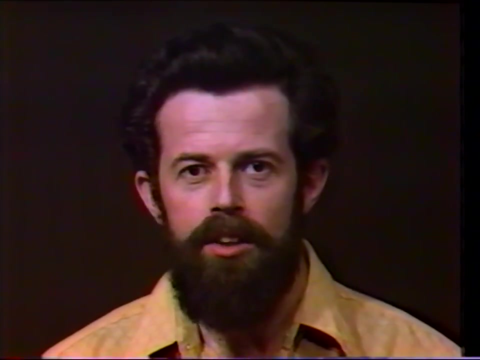 is a rock type of rock. The last rock type differs markedly from the earlier rocks. These are volcanic rocks in the westerly Selkirk ranges of the Rockies. Any mountain range, and that includes the Rockies, can seem very confusing at first sight. 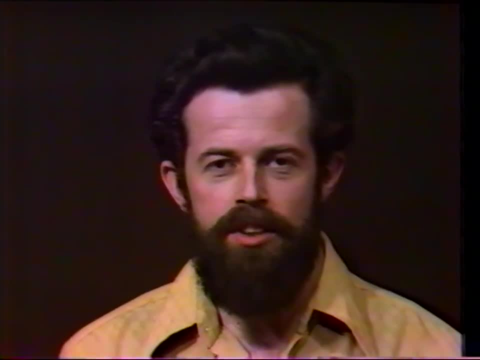 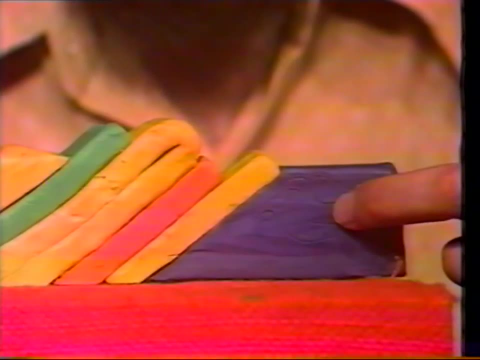 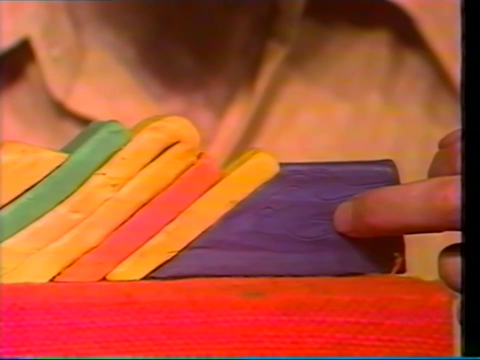 just a jumble of rocks faulted and folded. But if we build a model, then it's quite easy to identify the various elements of the mountain range. These are the strata which are formed from the erosion of the mountain range, sands and muds brought by rivers. 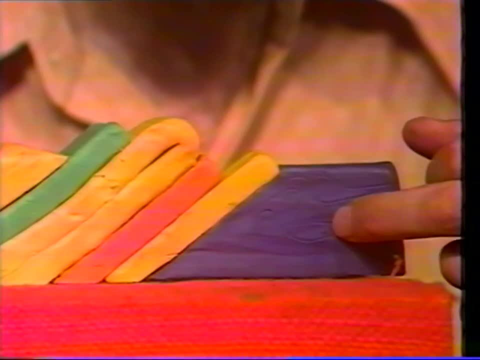 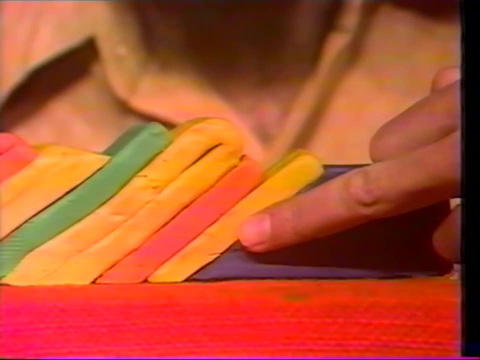 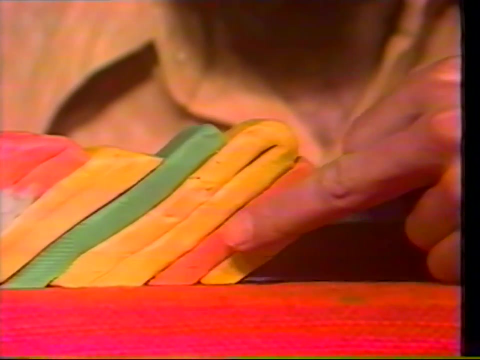 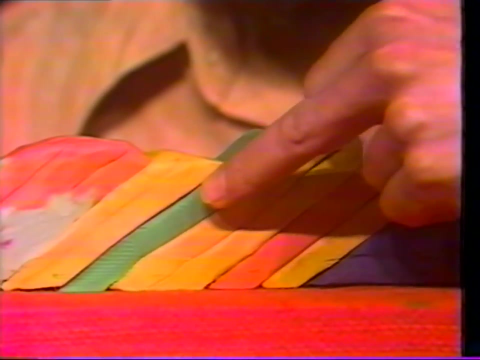 from the mountain range and deposited, for example, in the flat land around Calgary And then into the mountain range proper. the various thrust slices in the Rockies, mostly Cambrian and Ordovician limestones, sometimes folded More sheets. 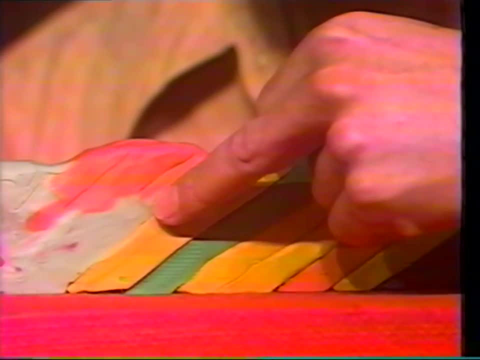 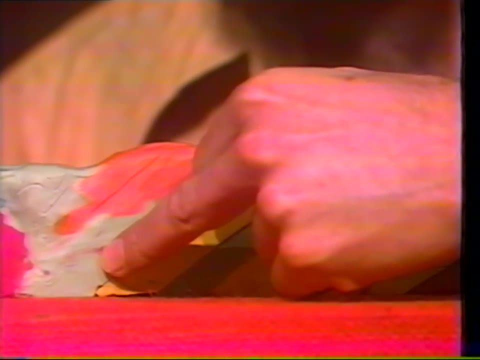 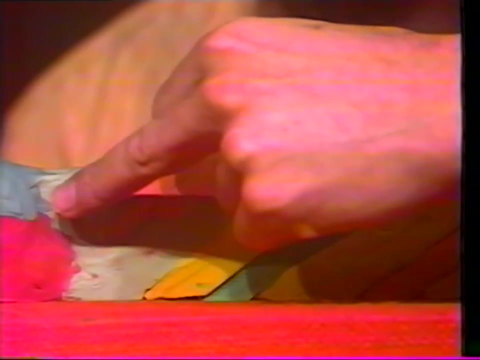 And here the very important facies: change or change in rock type, from limestone to shale, the somewhat darker colour on the model. That's a change that we'll look at in a moment, And then in the very west, volcanics. 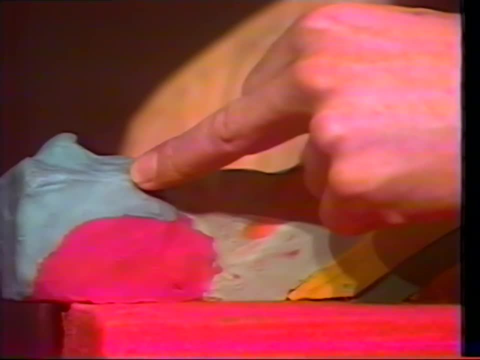 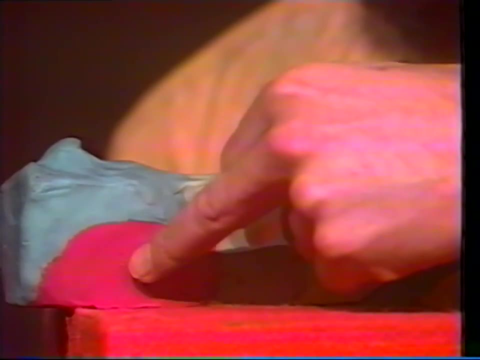 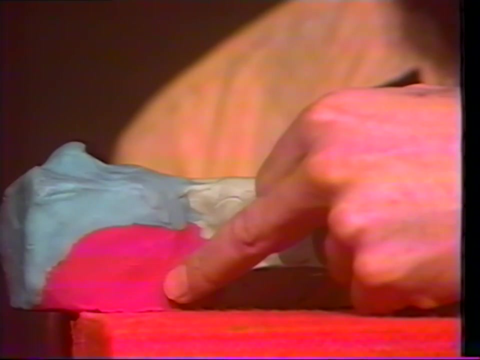 In fact, in the Rockies there are much more in the way of volcanics than we've represented on this model And, within the volcanics, intrusions of granitic-like rocks that we didn't see in the film but are nevertheless quite important. 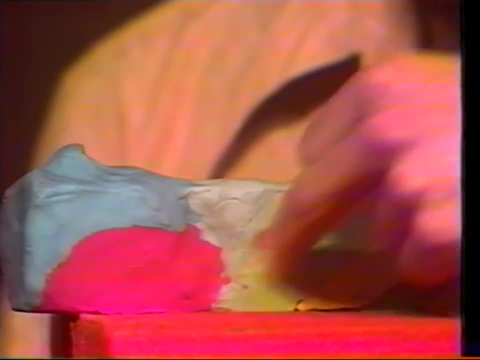 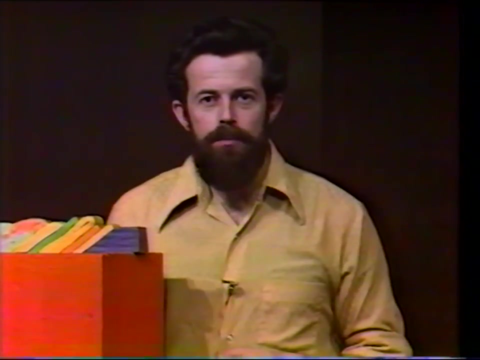 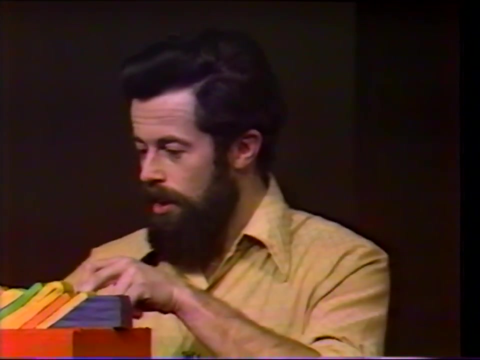 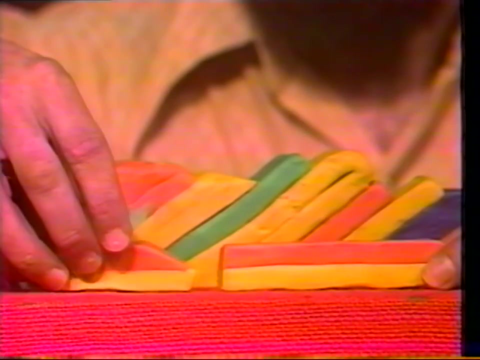 in the westerly ranges of the Rockies. Now, if we're to disentangle the importance of those different rock types, then we must disentangle the mountain belt itself, And to do that, what we have to do is to unthrust the thrust sheets. 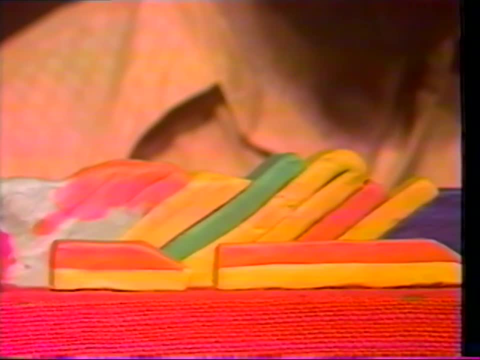 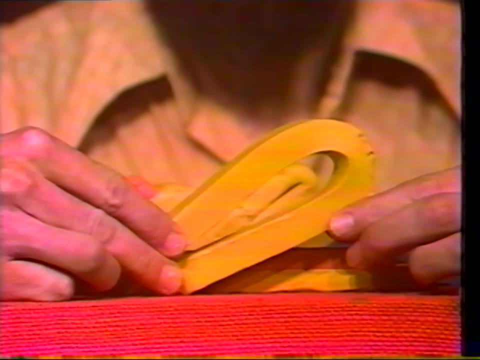 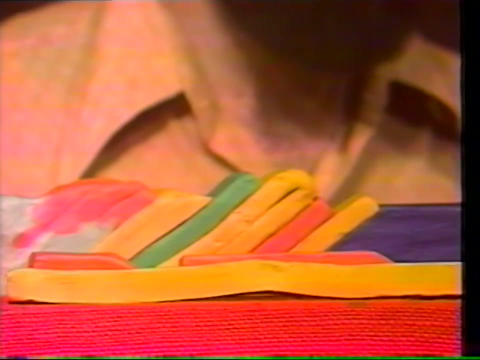 lay them out as they originally would have been, and we must unfold the folds, straighten out the strata as they would have been, And in this fashion we can build ourselves up a picture of what the mountain range was like, how the rocks were disposed. 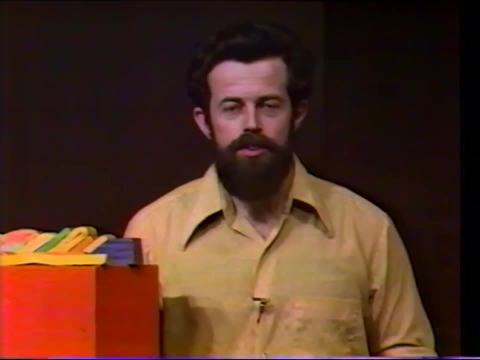 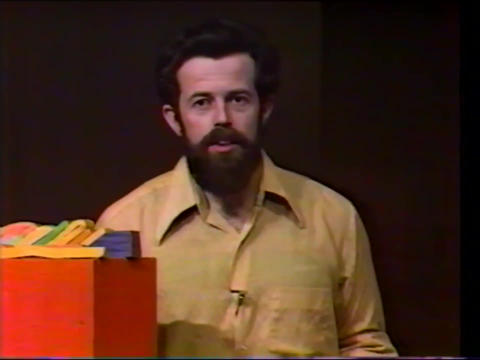 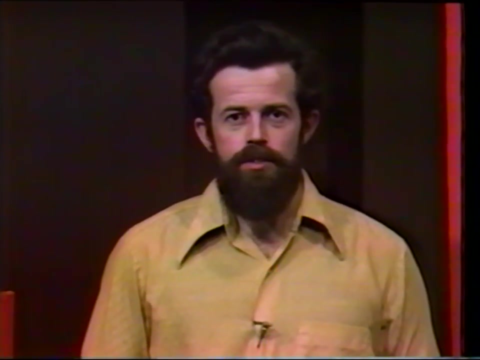 before the compression built the mountain range before the rocks were thrust, before they were folded, And if we do that, we find that we get three belts of rocks in the Rocky Mountains and also in most other mountain ranges In the Rockies. 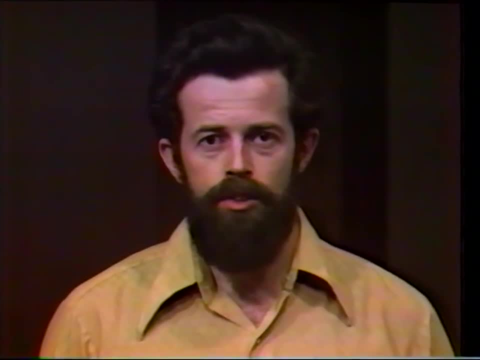 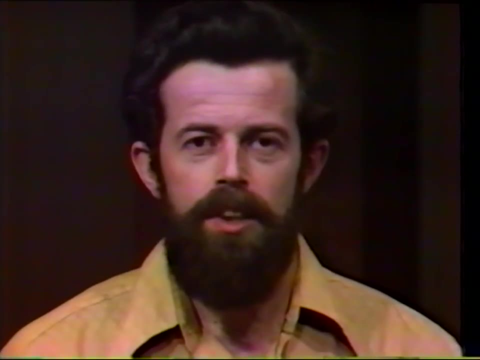 we have a broad belt of limestone with occasional sandstones with cross bedding in them, indicating that the sand has been built up and has been brought from the interior of the continent. So we can envisage there being a broad, warm, shallow sea. 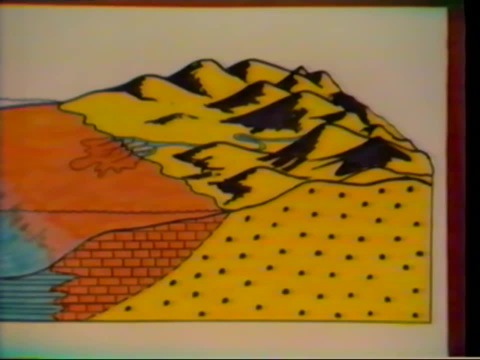 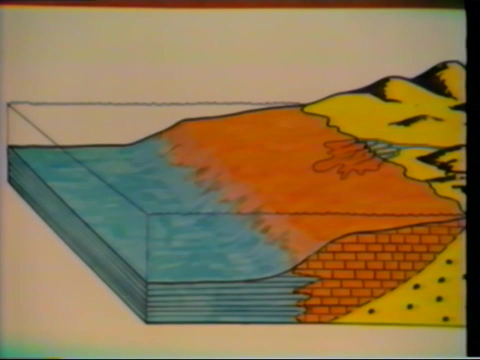 with rivers flowing into it, bringing some sand. That kind of situation is what we find on the continental shelf by Florida And then farther out. under what conditions do you think shale would be deposited? Well, shale at the edge of continental shelves sinks out of suspension. 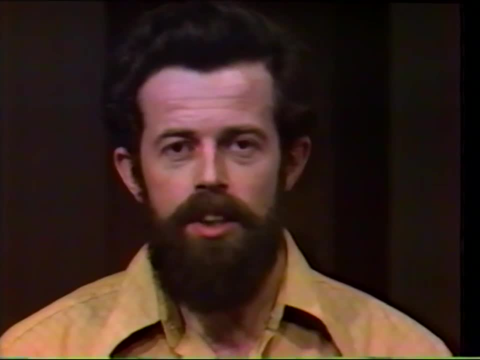 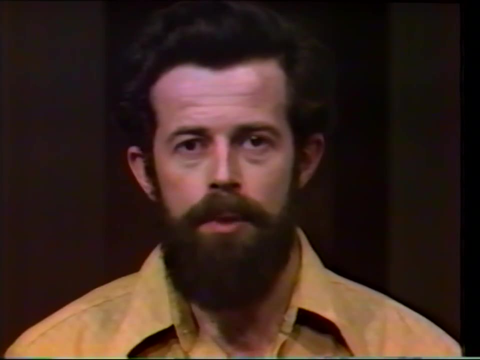 and forms thick muddy layers. That's the kind of situation in which, apparently, the rocks of the Rocky Mountains and also of other mountain ranges, such as the Appalachians, were deposited. Let's look at that situation on the continental margin. 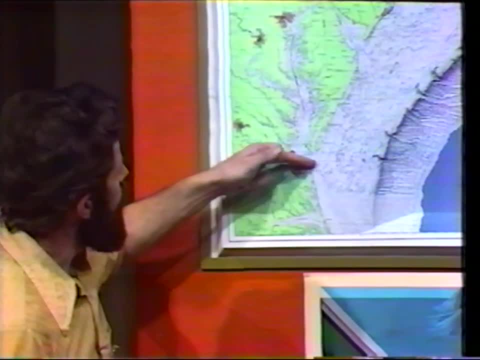 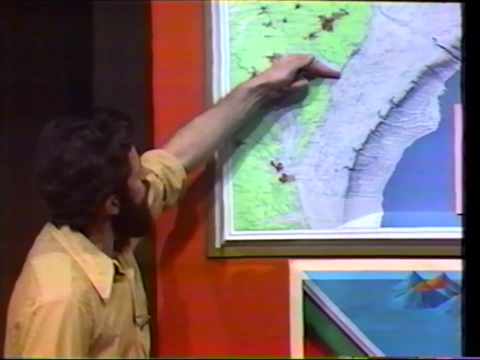 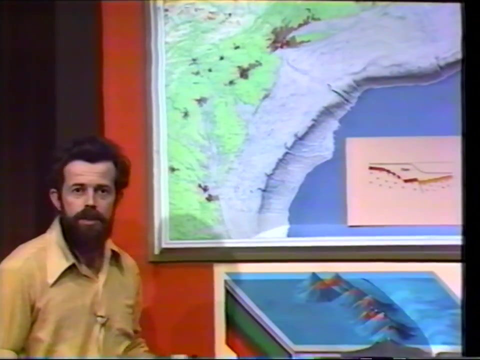 of the eastern United States. Here is the coastline, Here is Philadelphia And up here is New York. You remember we looked at this continental shelf in the first unit when we were discussing the origin of the sedimentary rocks in the Grand Canyon. Then the very broad shelf. 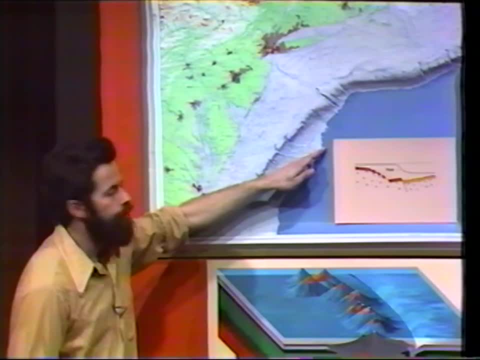 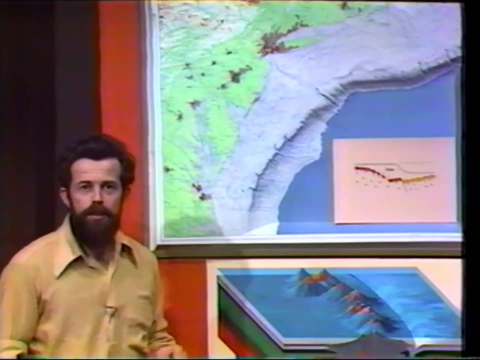 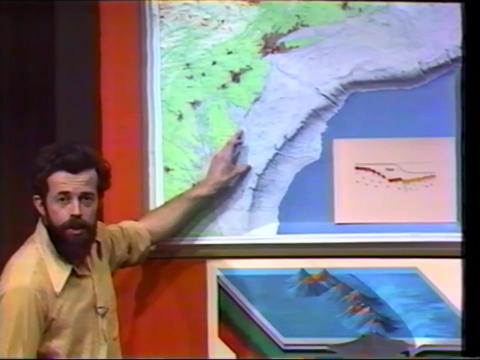 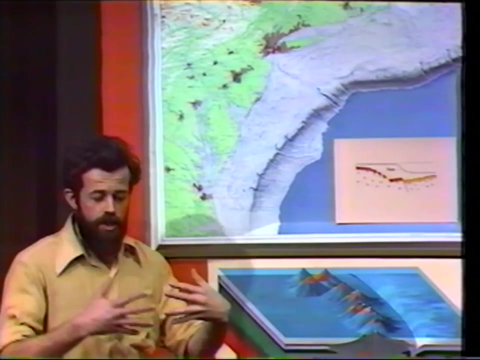 the continental slope and then the deep ocean floor of the Atlantic. In the time of the deposition of the Rocky Mountains. evidently very much of the area was limestone, deposited over a broad continental shelf And the edge was shaley And the transition between the two. 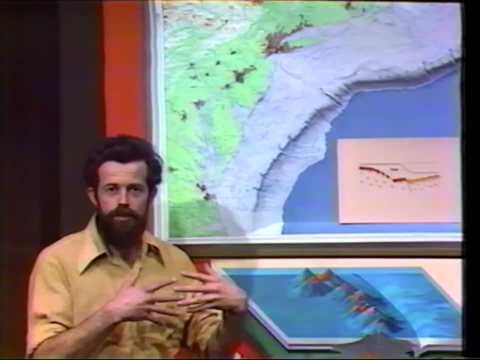 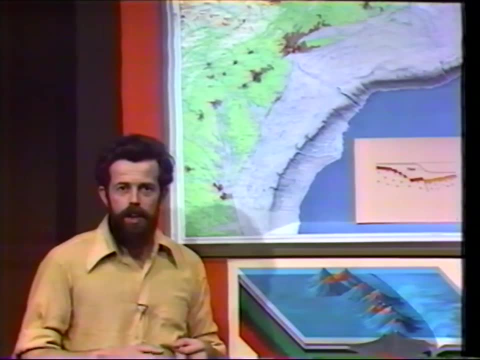 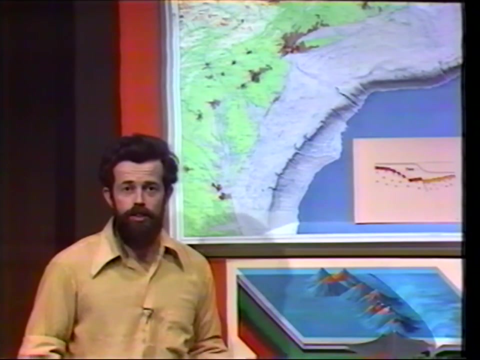 between the limestone and the shale in the Rocky Mountains must mark the approximate edge of the continental shelf, where the water became deeper and fossils, that is, animals and plants, were not able to flourish in the deep water, being out of the reach of light. 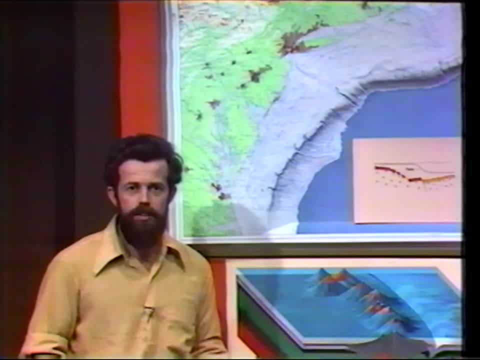 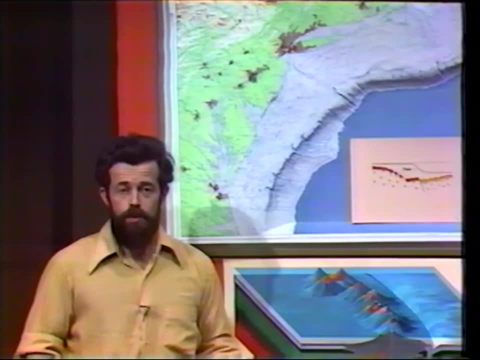 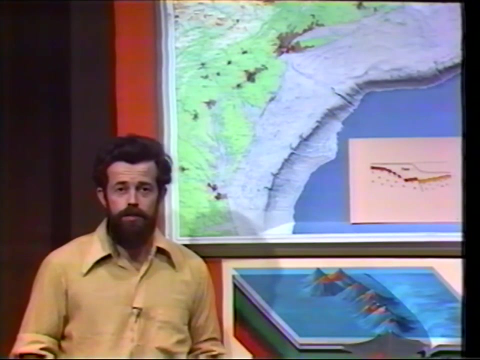 And therefore limestone was not deposited in that area and what we got was shale. Now you may think that sediments deposited on a continental shelf shallow water would only be thin, But in fact seismic work across a continental shelf, the continental shelf around the eastern United States. 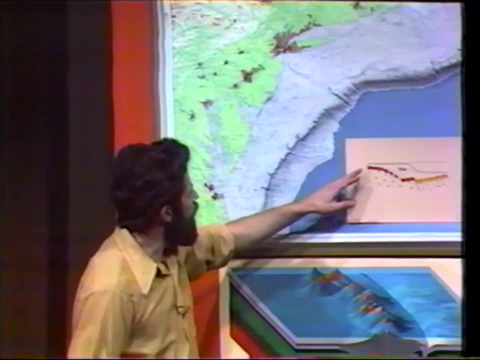 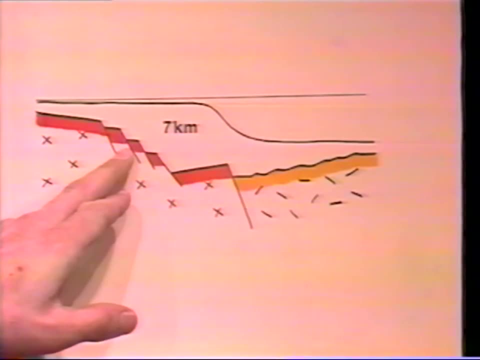 reveals that, in fact, the sediments are very thick. They're thick because, apparently, the basement on which they were deposited, the granitic kind of basement of the continental crust, is faulted, is broken by normal faults, which constantly slipping downward. allow the accumulation of sediment to thicknesses as great as seven kilometers, 7,000 meters- about 20,000 feet of sediment lies beneath the continental shelf of eastern North America, And then the sediment thickens and we meet the ocean floor. 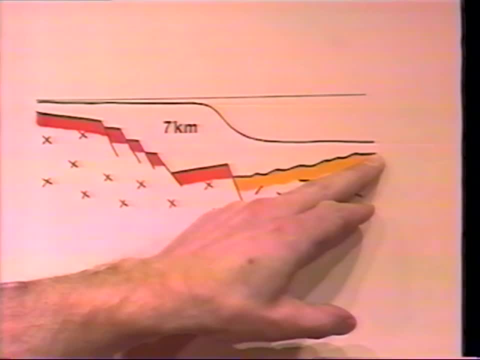 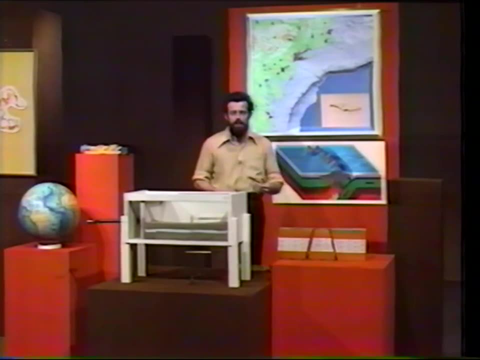 I'm sorry. the sediment thickens And we meet the ocean floor, So the kind of situation in which it seems the Rocky Mountains have their beginnings is as sediments on a continental shelf and the constant down-dropping of the basement on which the sediments were deposited. 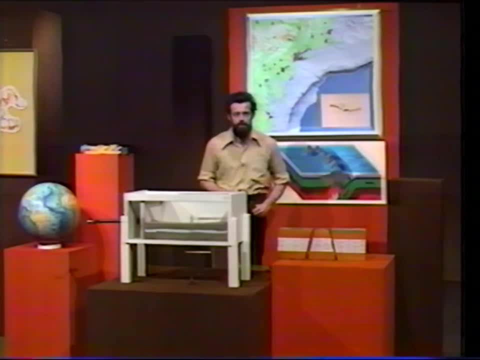 allows them to build up to very considerable thicknesses, And we find in fact thicknesses like 20,000 and 30,000 feet of shallow water sediments in mountain bolts such as the Rockies and the Appalachians. But that's just a passive situation. 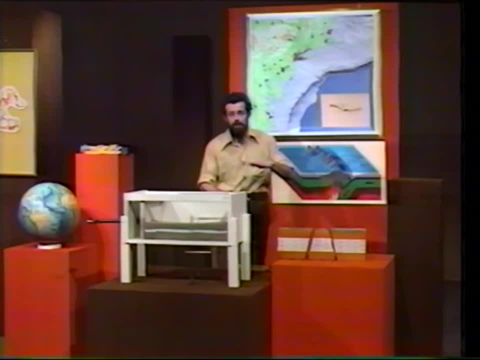 the accumulation of sediment getting thicker and thicker and thicker. How do we get from that stage into the mountain bolt stage, into the deformation stage? How do we convert that passive kind of continental margin such as we have on the Atlantic into an active continental margin? where mountain bolts are bolted, An active continental margin, for example, like the Andes, like the western coast of South America. How do we get to that stage? Well, you should be able to remember how we get an active margin to a plate. 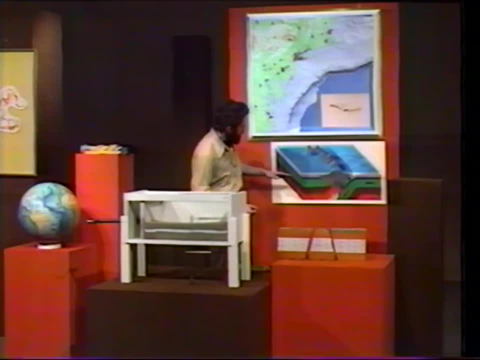 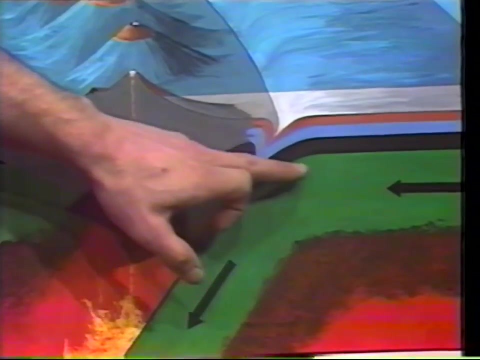 by the breaking of a plate. Here, oceanic lithosphere is diving down between beneath another piece of oceanic lithosphere, A break having taken place at this point, this piece having then dived down, producing volcanoes. You remember this situation. 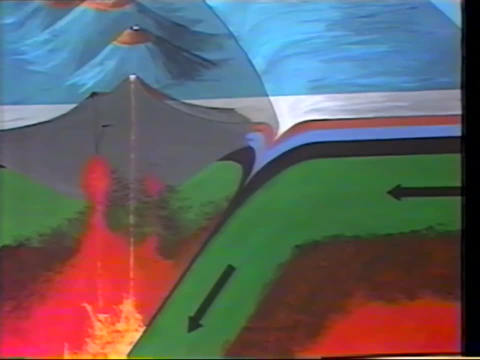 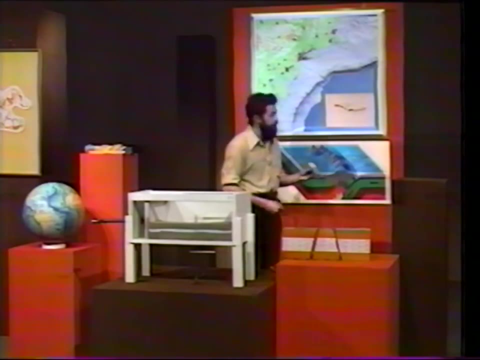 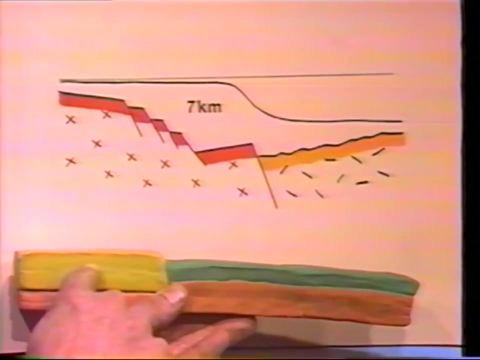 from plate tectonics and volcanoes. You should know it very well. So let's look at how that happens or might happen. in the case of the Atlantic continental margin, There is the continental margin as it is today Here: continent. 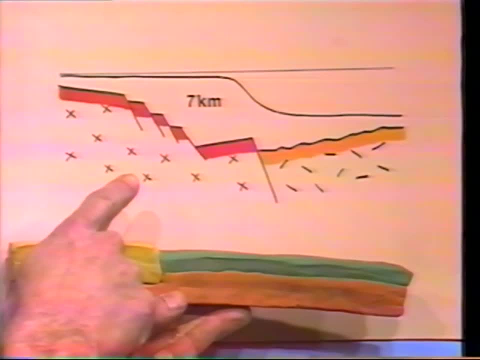 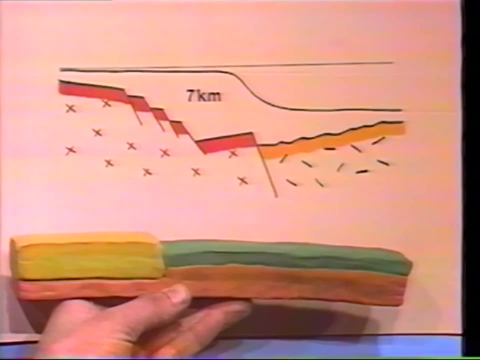 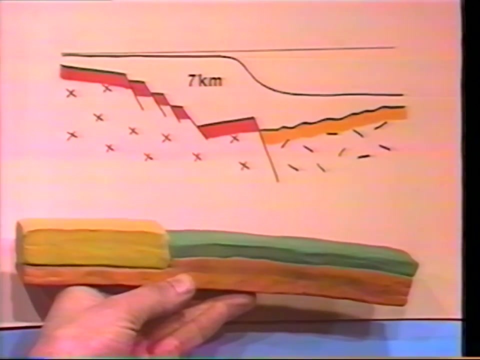 There continental shelf, very much enlarged in that upper diagram, And here ocean floor and beneath it all mantle. So that's a cross-section of the lithosphere at the edge of an Atlantic-type continental margin, the kind of margin on which 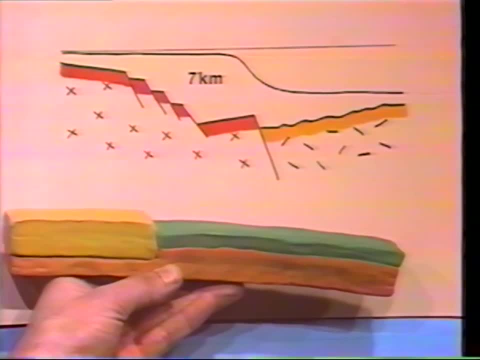 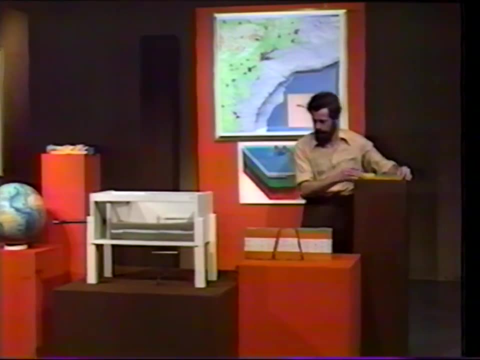 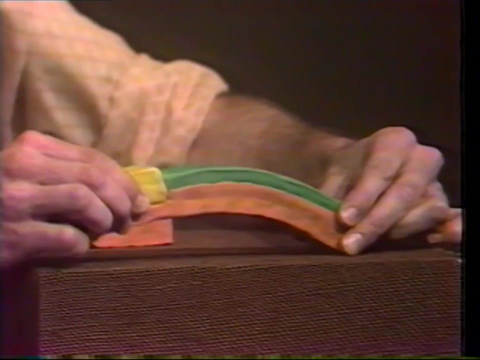 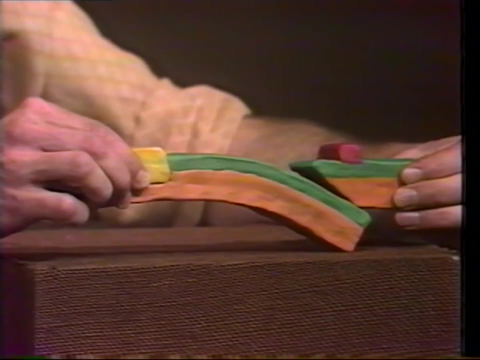 the sediments of the Rocky Mountains began their history. Now then, let's see what happens to that in order to turn it into an active continental margin. Well, imagine then that it breaks and begins to descend, And it descends beneath the piece of oceanic lithosphere. 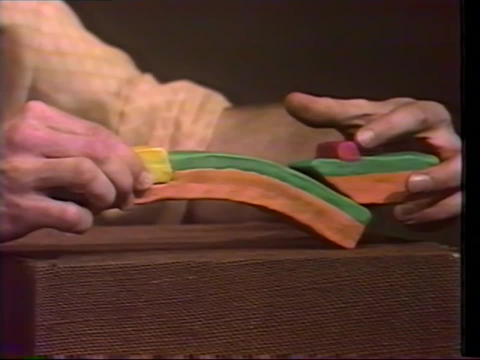 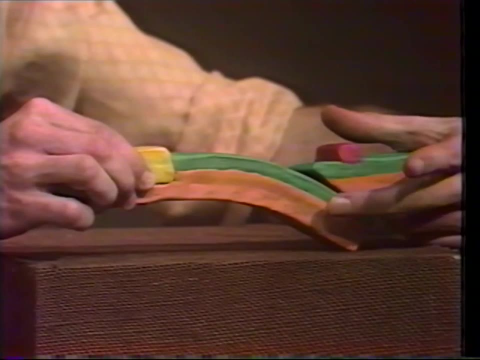 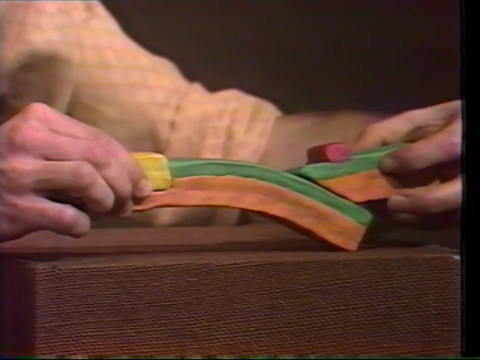 that was originally joined to it, And an island arc builds up. Now, then, what happens? as this piece of oceanic lithosphere continues to dive down, continues to subduct The island arc, which, remember, is formed of andesites. 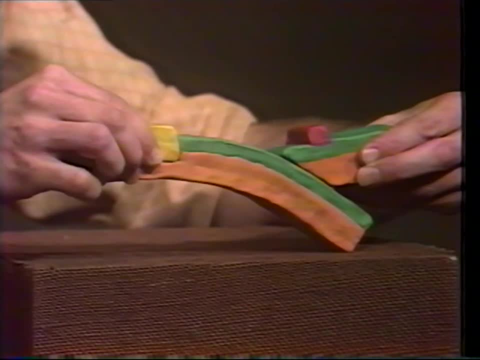 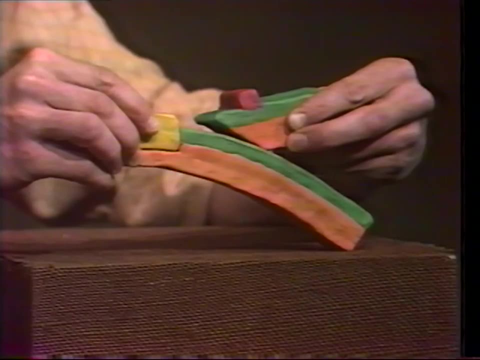 gets progressively closer and closer and closer to the continental margin. Well, we can't do it very accurately with plasticine because it doesn't bend enough. But you can see what's going to happen: That island arc is going to collide with the continental margin. 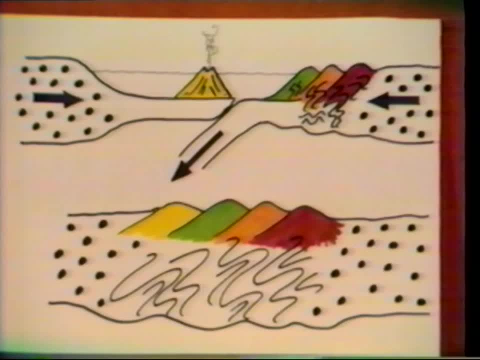 Now, of course, once the first island arc has collided with the edge of the continent, if the ocean is to continue to spread from the spreading ridge in the center of the ocean, then another fracture must take place in the ocean crust. And if that fracture takes place, 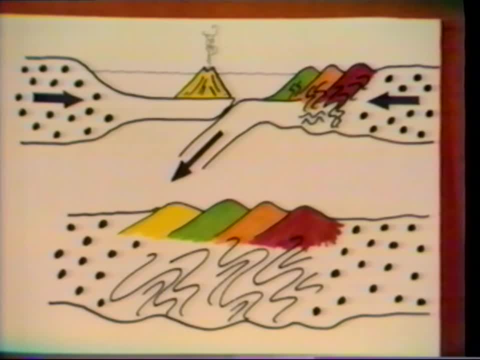 in the same fashion as it had originally, then another island arc will grow and that island arc will collide with the continent And in this way a succession of island arcs can be welded onto the edge of the continent. In this way, continents grow. 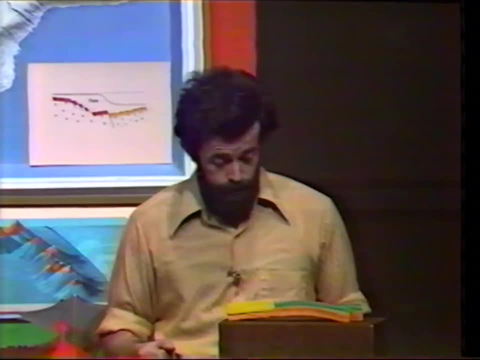 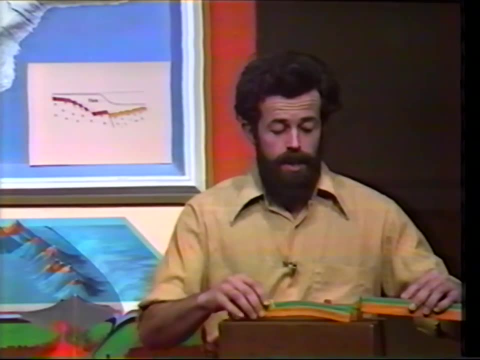 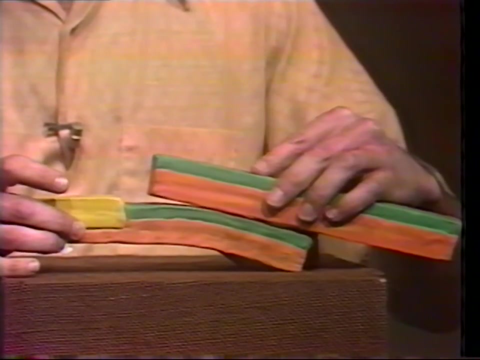 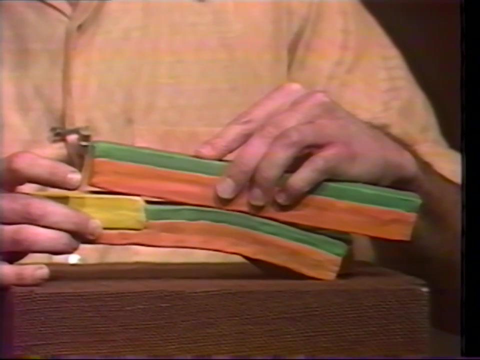 That's one of the ways. Anyway, another thing can happen which is indicative of this kind of event at the edge of the continental margin, and that is that the split may result in ocean crust being driven onto the continent. It's rather a peculiar thing to happen. 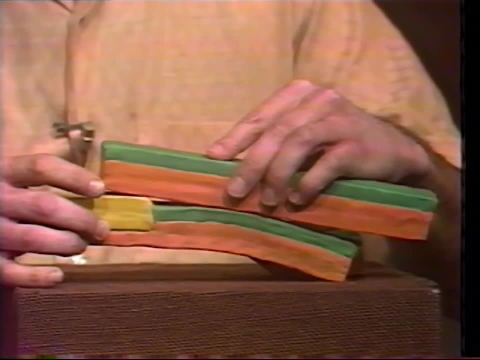 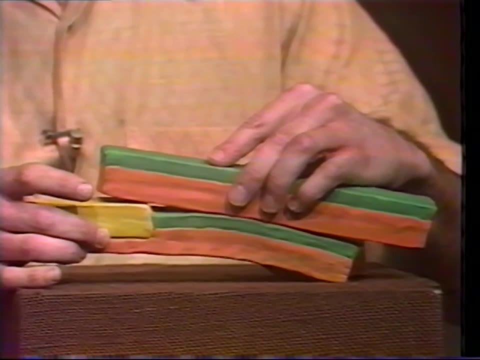 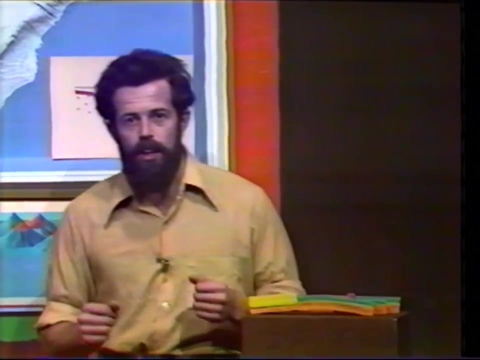 Usually, what takes place is that the ocean crust dives down, But now and again slabs are in fact driven up onto the continent, And we find that in, for example, the Appalachian Mountains. Now, the collision of the island arcs. 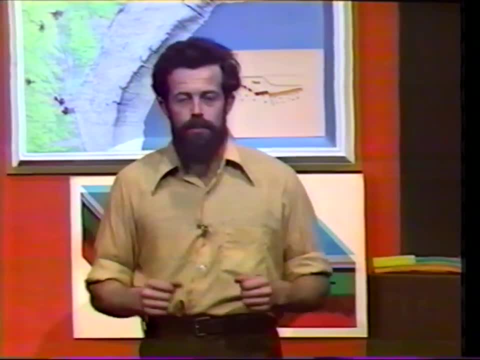 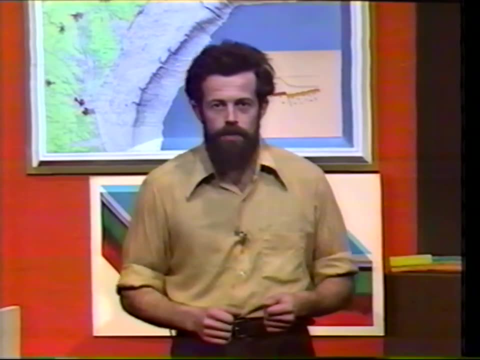 with the edge of the continent, with the sediments that have been accumulating there on the continental shelf, which is subsiding, leads to the compression of those sediments. So let's go to the squeeze box again, which we looked at in the unit on deformation. 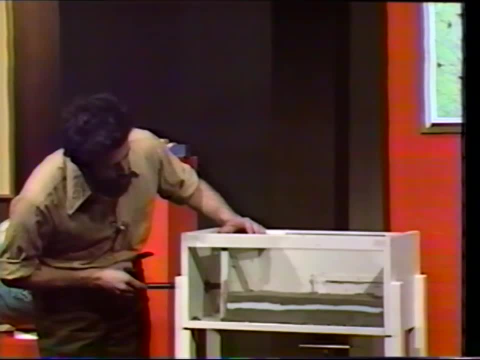 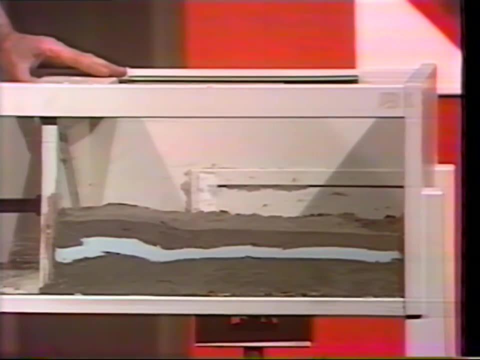 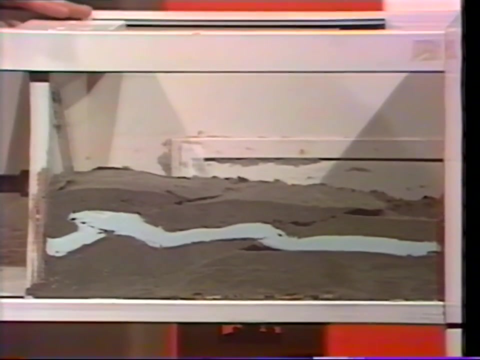 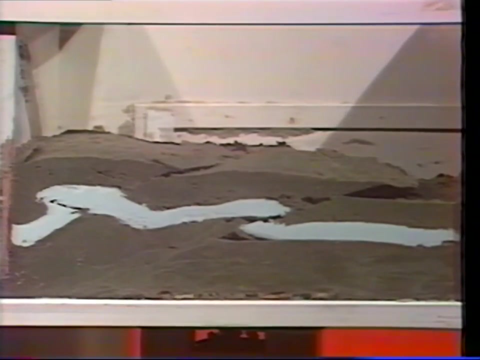 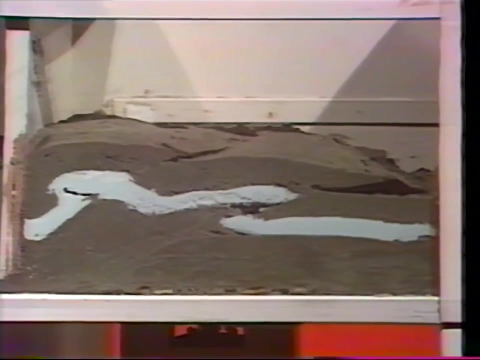 and see what deformation of the strata produce. this time, Imagine the island arc colliding with the continent. There's a very fine thrust fault developing just here. A slice is being driven over rock which is in fact younger than it, And quite a fine fold. 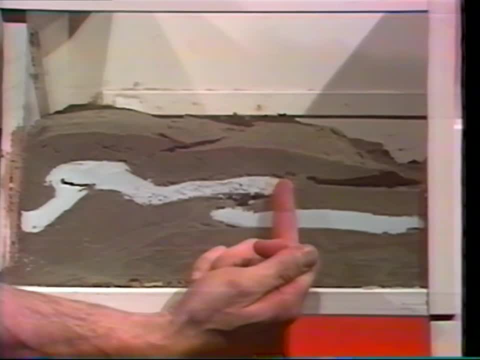 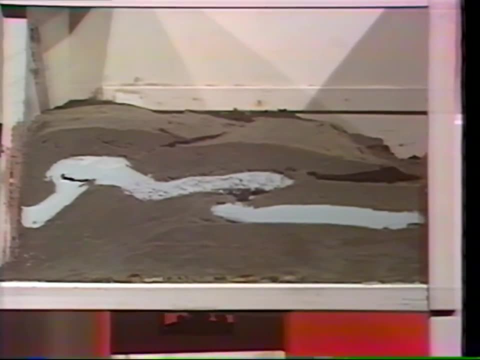 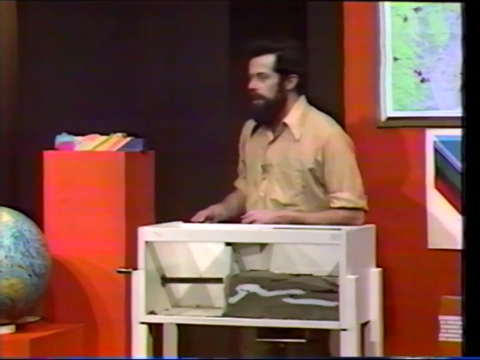 Which has also begun to fracture. There the sand has been thrust right over the strata which is younger than it. Quite a good example of the kind of thing that happens in a mountain boat. Compare it, for example, with the Rockies, with the model that we constructed earlier. 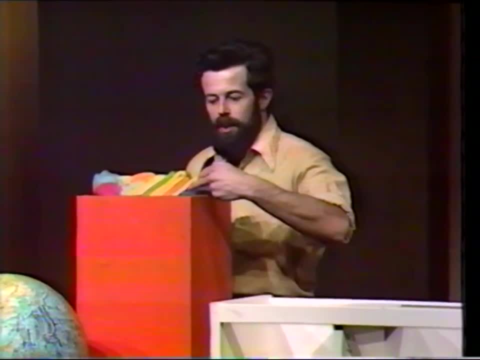 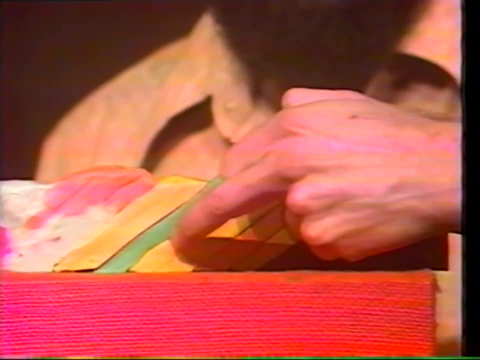 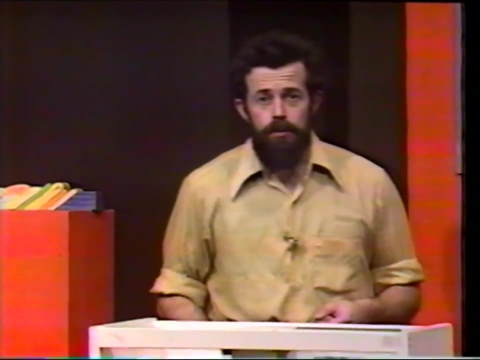 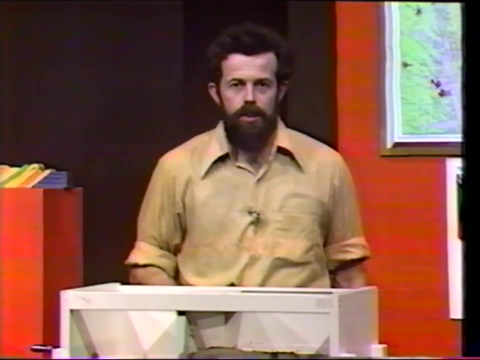 You can see in the model thrust sheets and folds Very similar to those that we've just produced in the squeeze box. Now that's a kind of mountain boat. we call a collision mountain boat At this time collision of island arcs with the edge of the continent. 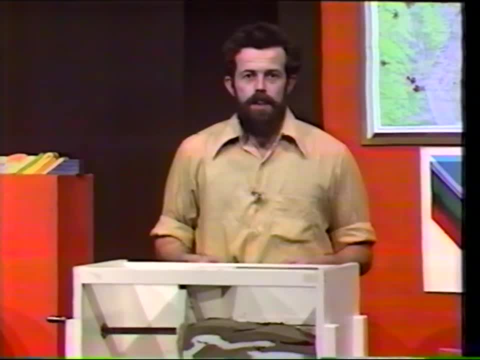 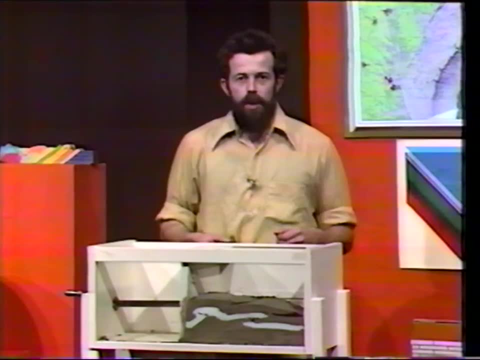 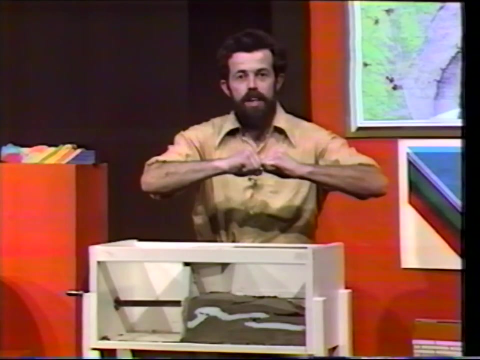 Now, if you imagine the ocean continuing to be subducted, continuing to be destroyed at the edge of the plate, then it's quite easy to imagine that the two continents, on both sides of the ocean, can also come together and provide us with another kind of collision. 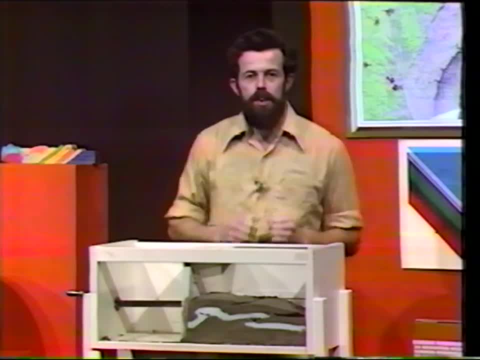 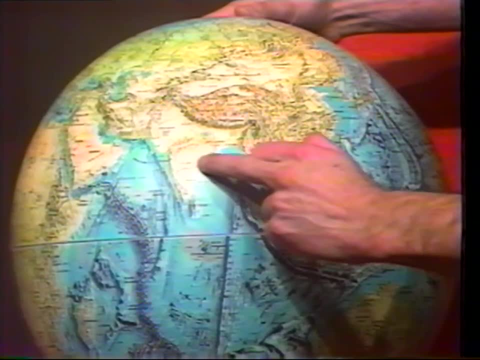 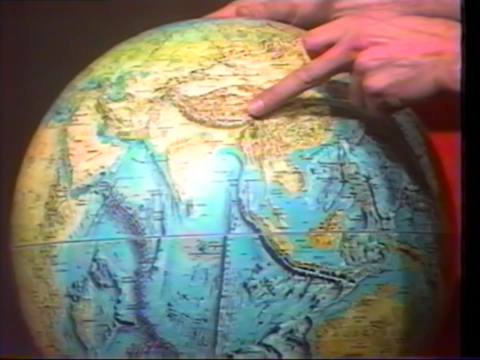 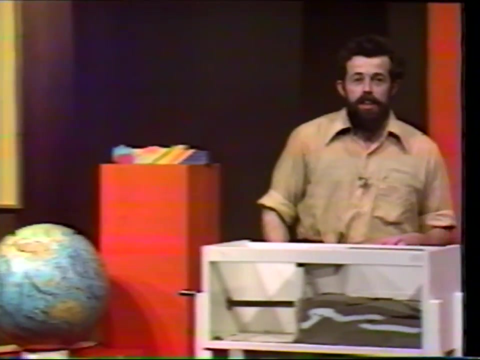 That's the kind of collision which took place between India and Asia, India moving north, colliding with Asia, producing the Himalayas. You probably remember that mountain boat from the plate tectonics program. Another case of a collision mountain boat between two continents is the Alps. 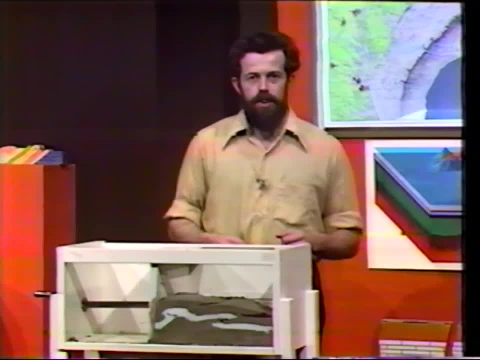 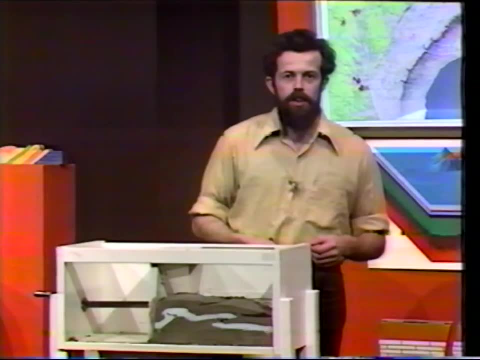 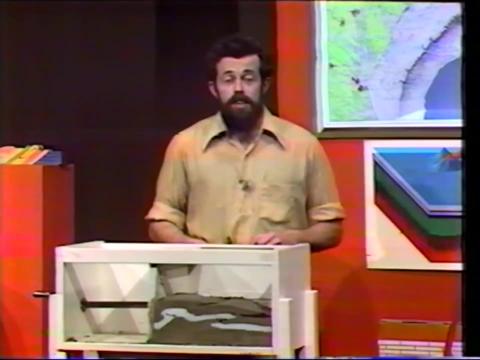 And there the ocean which lay between Africa and Europe is still present. Part of it is still The Mediterranean. That's the ocean that was destroyed as the two continents came together: Africa and Europe. Now there's another kind of mountain boat. 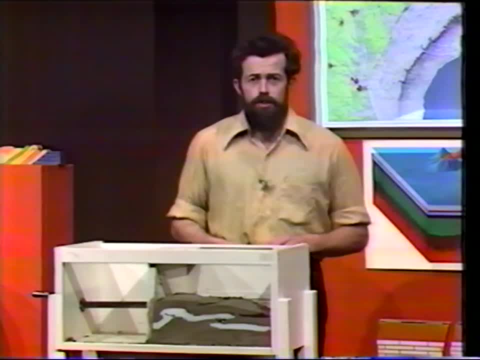 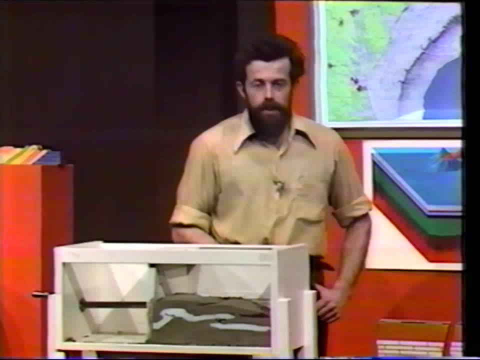 which you've also seen in the unit on plate tectonics, which is not caused by collision, And that is the Andes, The Andes on the west coast of South America. There the mountain boat is dominantly formed by the compression. 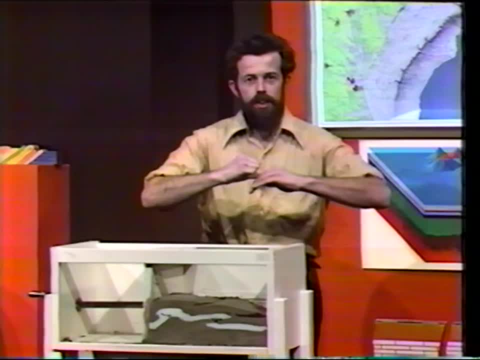 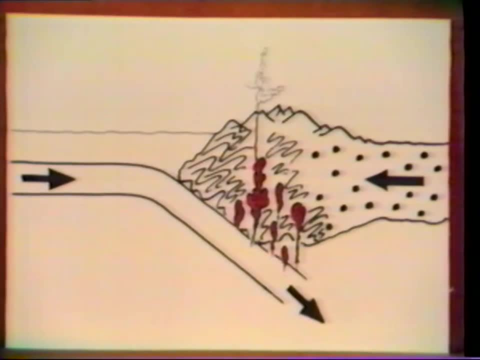 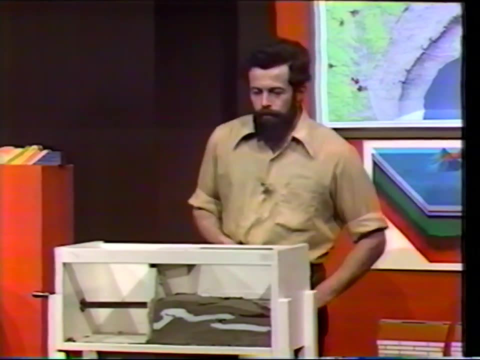 of a subducting plate beneath the edge of the continent, but also the vertical rise of molten liquid, molten rock, produced by the partial melting of the solid plate as it descends beneath the edge of South America. Let's do some vertical movement. 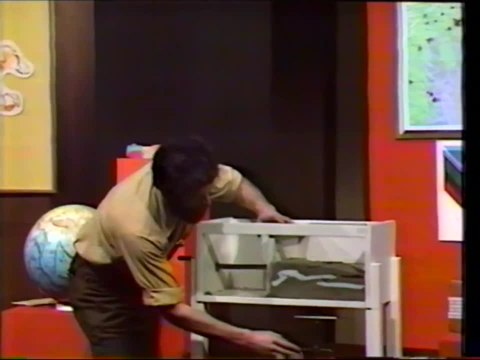 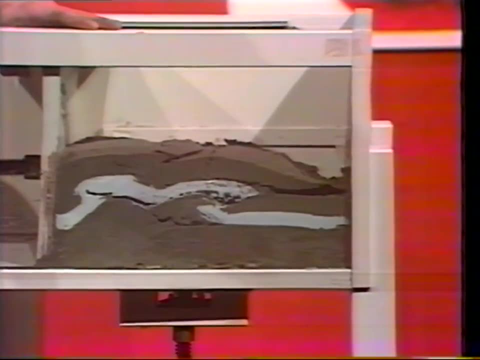 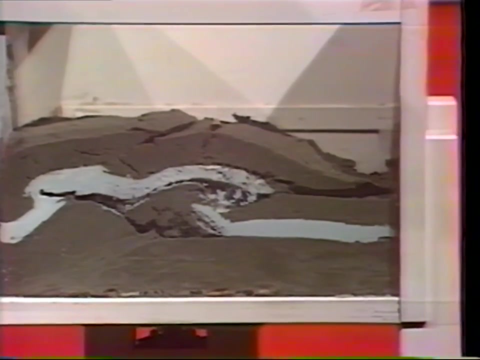 on the squeeze box this time and see what kind of effect that has There: the strata being dormed upward. Imagine the liquid from a subducting plate rising and forcing the strata upward And, of course, bursting through to the surface. 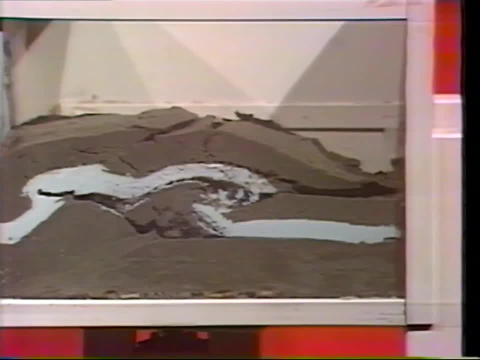 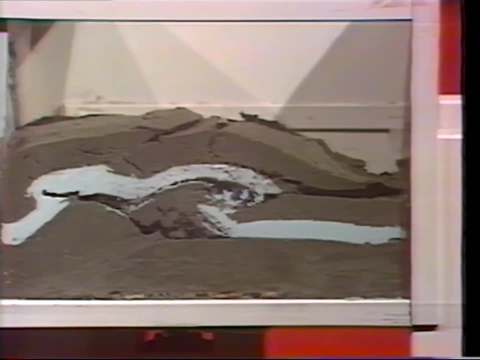 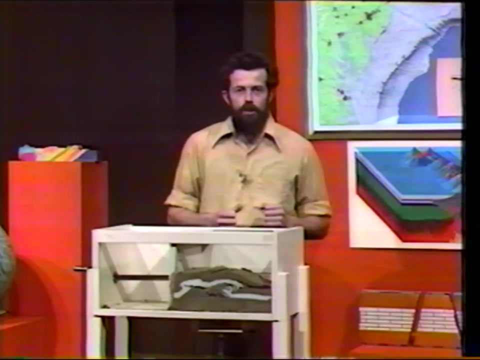 and producing volcanoes. And there you have the Andes. So the Andes show more vertical movement than the kind of mountain boat that we described as a collision mountain boat. So we've got two kinds of collision mountain boats and also what we could call 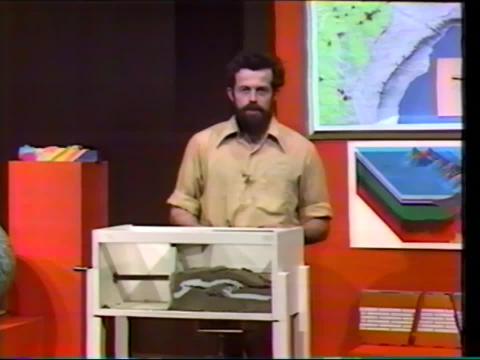 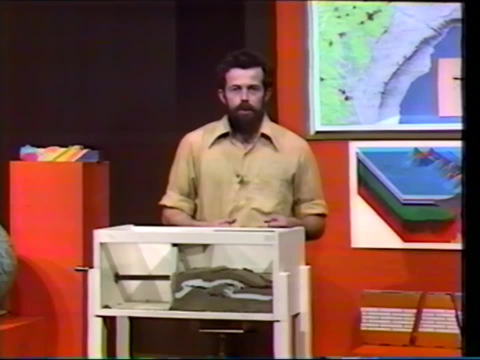 if you like, a dominantly thermal mountain boat. That is, a mountain boat in which a lot of the movement, the upward movement, is produced by rising molten liquid, That is, by rising molten liquid, Now, in all of the cases. 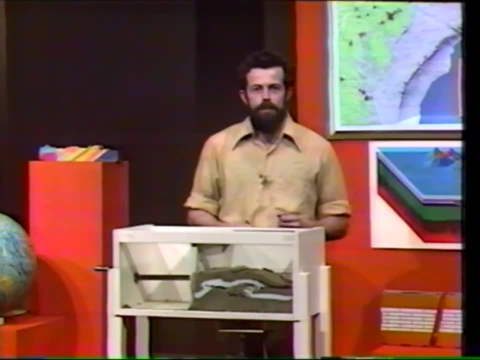 that we've discussed. the mountain boat has been produced at the margin of a plate, And when we look at ancient mountain boats, the good question to ask oneself is: well, where are the margins that those mountain boats grew on, so to speak? 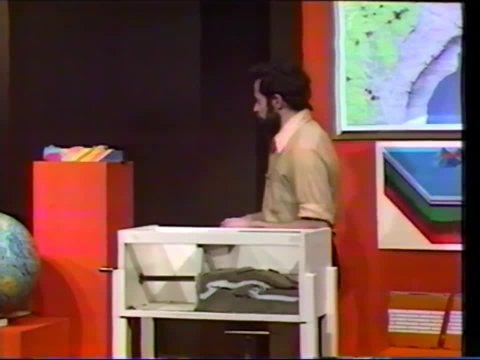 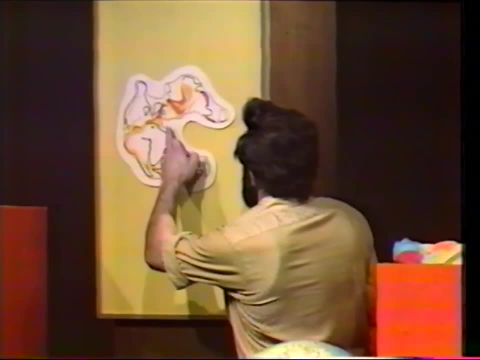 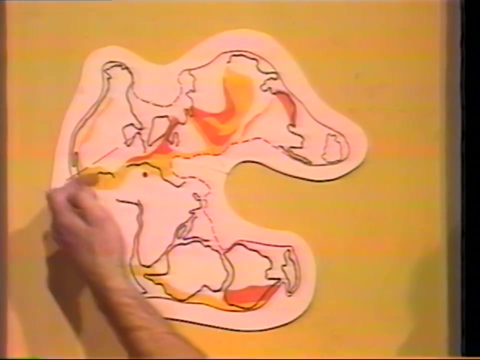 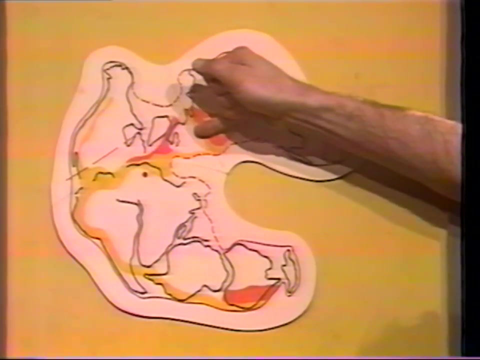 Well, let's have a look at some mountain boats, some ancient mountain boats, and see where the edge of the plates might be. The Appalachians lie in this position: Here is North America, Here is Greenland, Here is Europe And here are the southern continents. 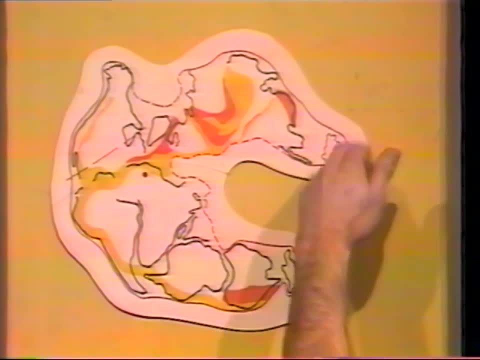 of Gondwanaland And the whole makes the supercontinent that you know already, Pangaea. So in fact in the reconstructed Pangaea the Appalachian Mountains lie inland, so to speak. There's no obvious margin, even in Pangaea. 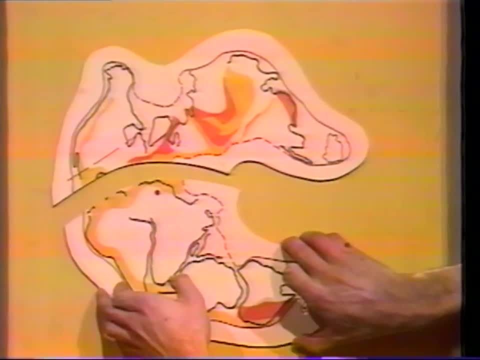 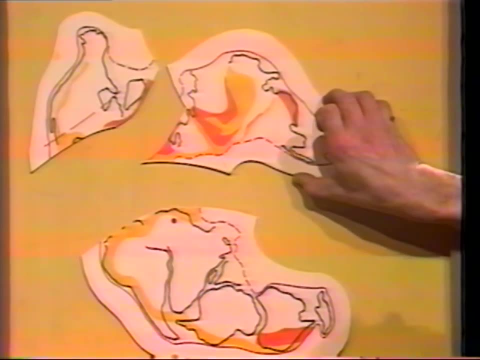 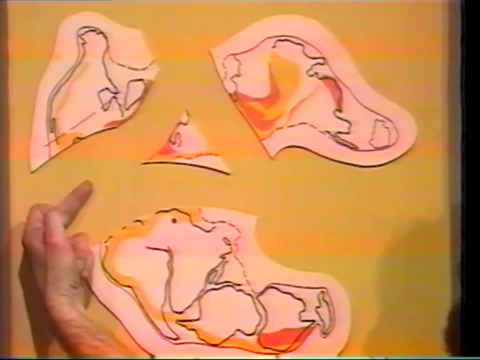 But if we remove this part, we remove this part, and then we also remove this and we imagine ocean in here and in, here, and in here, and we imagine the events we've just described: the coming together of continents by the consumption of ocean plate. 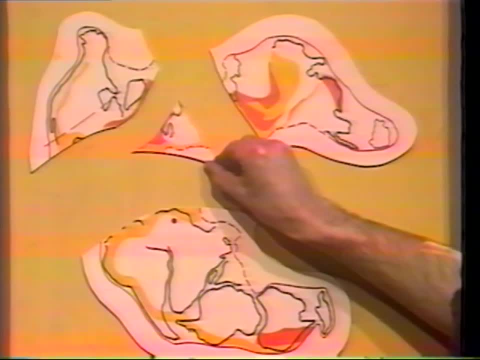 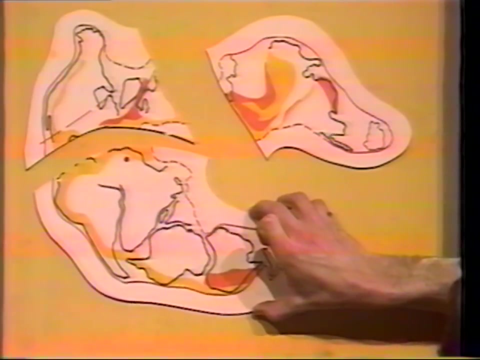 then this is the situation which created the Appalachians: Western Europe moving up toward North America and Greenland about 370 million years ago, producing a collision mountain boat. A second event: the movement upward of the southern continents, Africa in particular, about 280 million years ago. 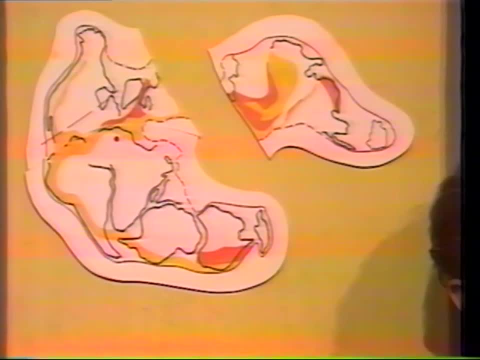 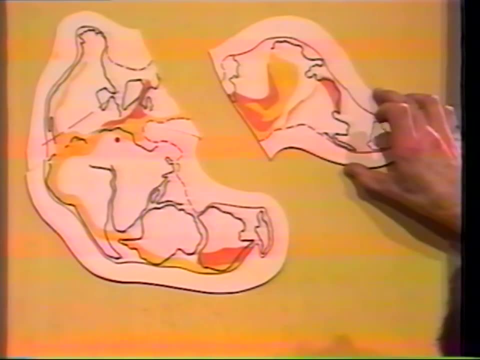 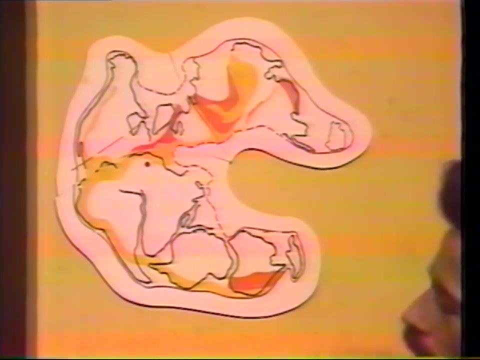 producing another collision on the North American continent, this time affecting particularly the southern part of the Appalachian Mountains And then finally, the Ural Mountains, which also seem to lie without being at an edge of an obvious plate. they were produced by the coming together. 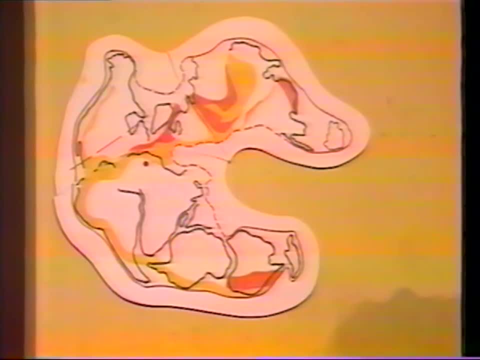 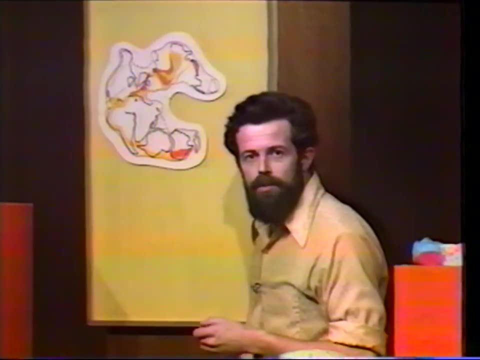 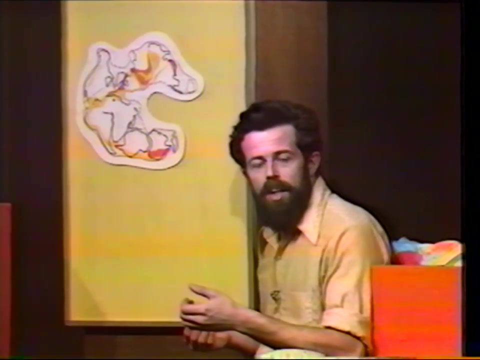 of Asia and Western Europe. So, although the mountains in Pangaea and the ancient mountain boats we see today don't seem to be obviously related to the edges of plates, in fact if we take apart the plates along the line of the ancient mountain boats, 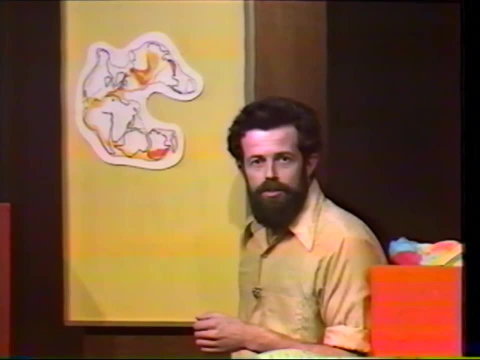 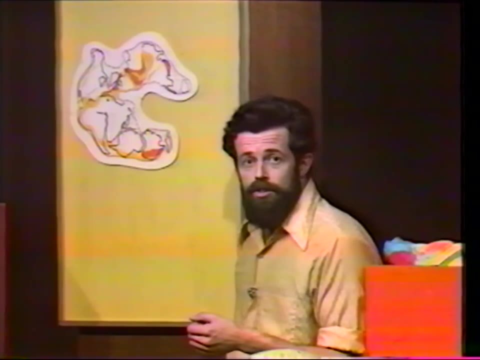 we can see very clearly how the ancient mountain boats were in fact related to the edges of plates. Now the Appalachians are of particular interest to us. We'll be looking at the Appalachians in detail in the next part of this unit, in the second part. 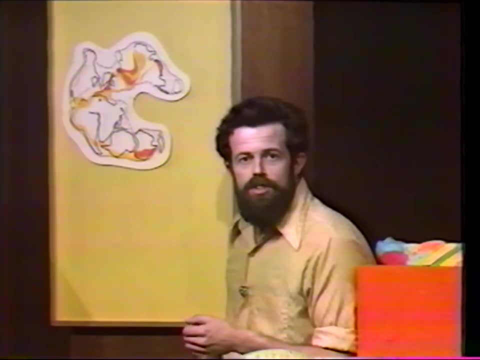 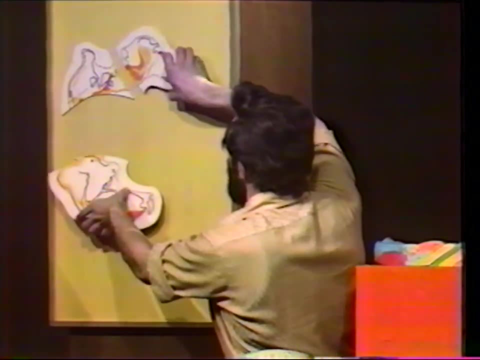 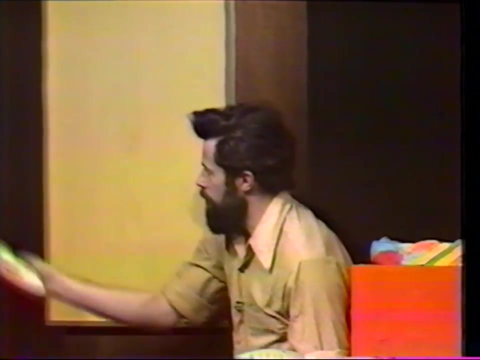 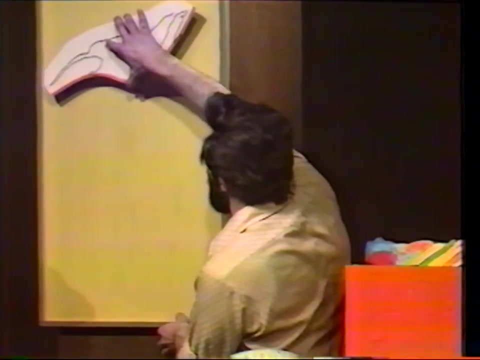 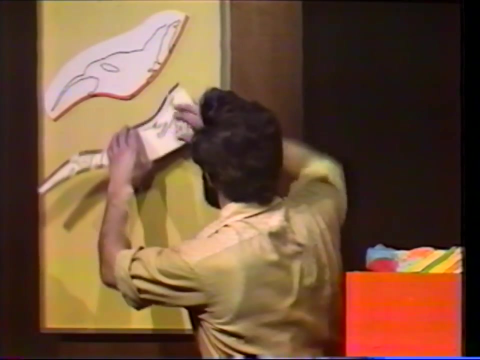 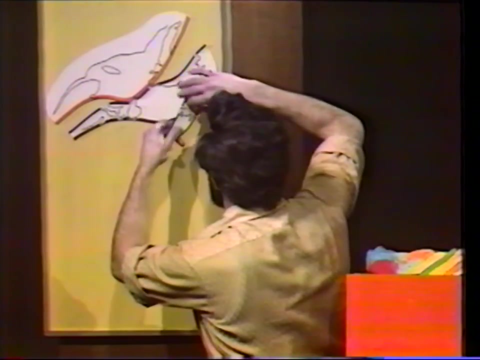 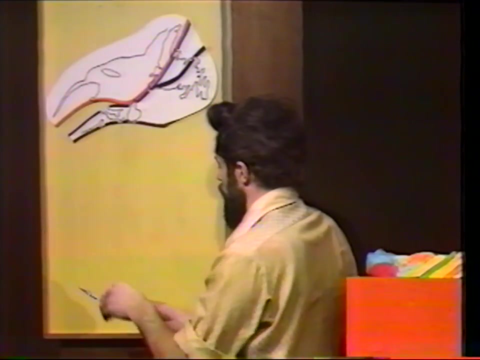 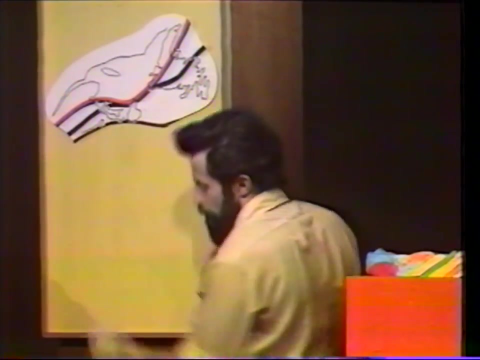 So let's look at the Northern Appalachians in Newfoundland and Nova Scotia in detail. Let me take these away first And replace them with the detailed parts of Nova Scotia and Newfoundland And explain each of these, Each of these pieces of that area of the Appalachians. 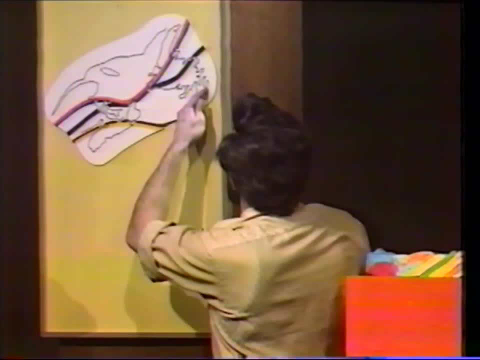 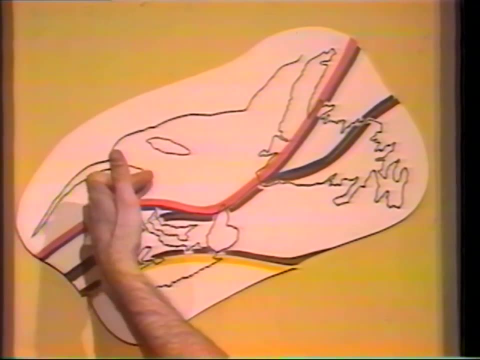 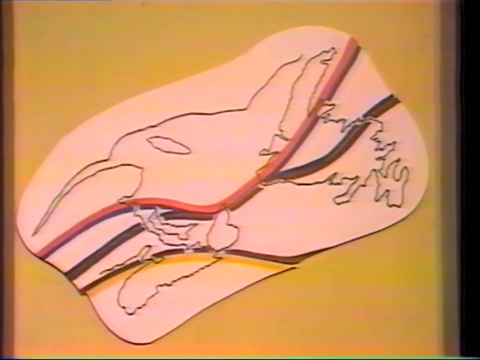 That's how it looks today. Here is Newfoundland, Here is then the mainland, the Gulf of St Lawrence, New Brunswick, Nova Scotia, Prince Edward Island. Now, as a result of the two collisions which produced the Appalachian Mountains and then the splitting apart again, 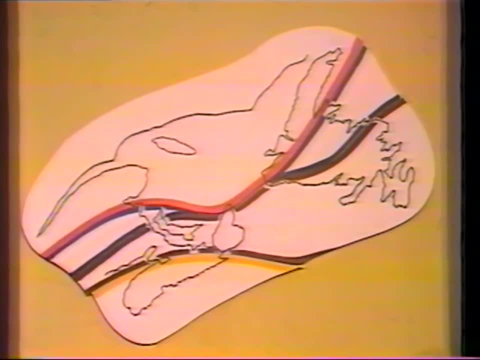 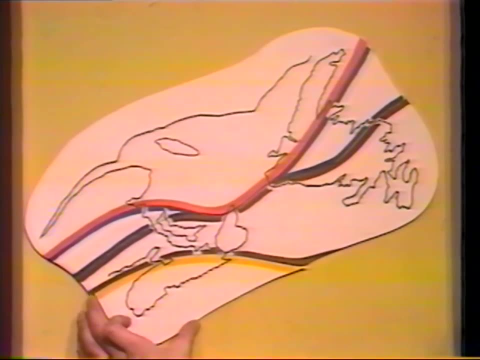 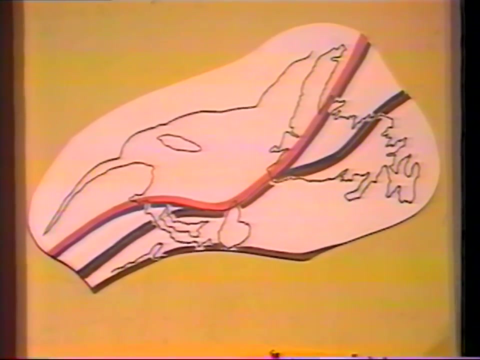 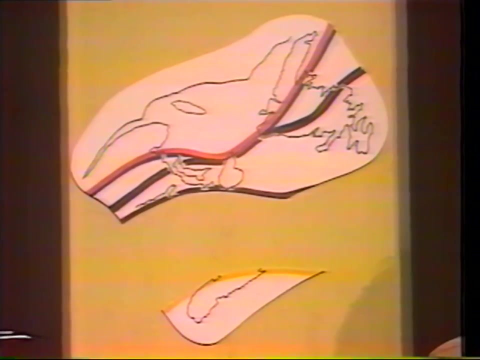 to produce the present Atlantic. we have in the Maritimes the following geological jigsaw, if you like. This part of Nova Scotia is in fact, a fragment of Africa that was left behind on the North American continent when the new split producing the present Atlantic took place. 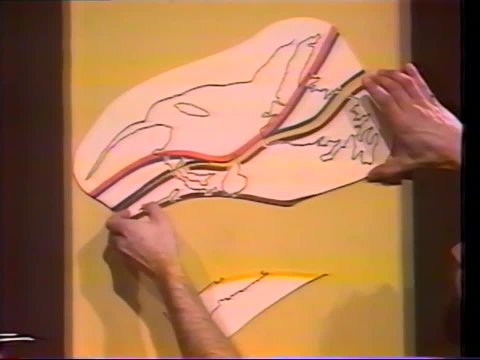 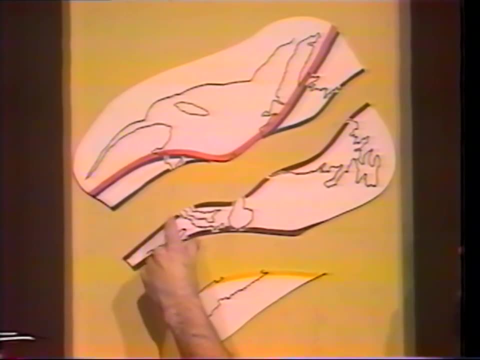 This part, which includes the southern part of Newfoundland, Prince Edward Island, part of New Brunswick, that is continental crust And seems to have been perhaps an island, rather like Madagascar, Although a very big one, that lay close to the shore of the North American continent. 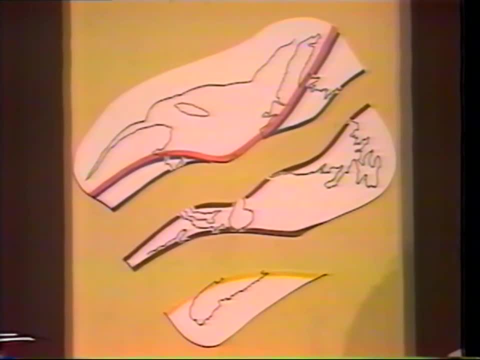 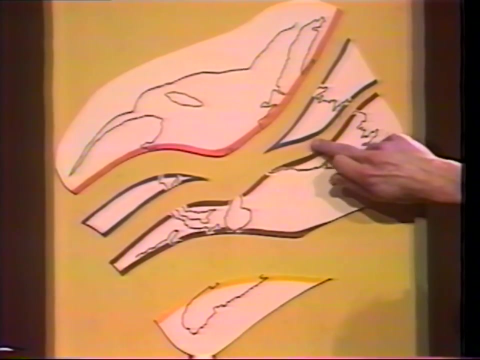 And was also rammed up against the continent during the two collisions Of Western Europe with North America and Africa with North America, And then forming the central part of Newfoundland and also forming part of the St Lawrence estuary area, are two wedges of what is left of the intervening ocean. 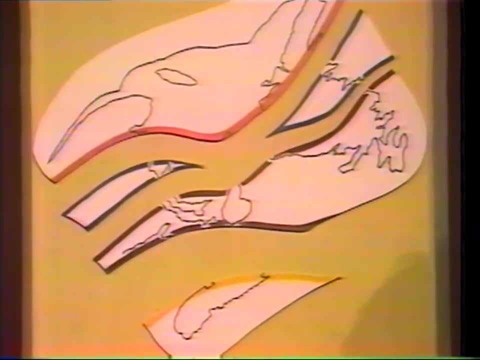 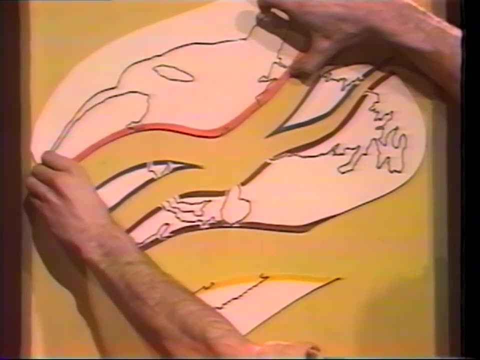 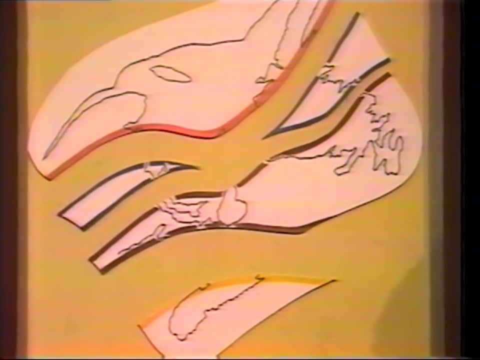 The ocean that was the Atlantic 280 million years ago. And finally, on the north we have the edge of the North American continent. So during the two collisions which produced the Appalachian mountain bolt, these fragments were welded onto the edge of the continent. An ocean destroyed, two fragments left. 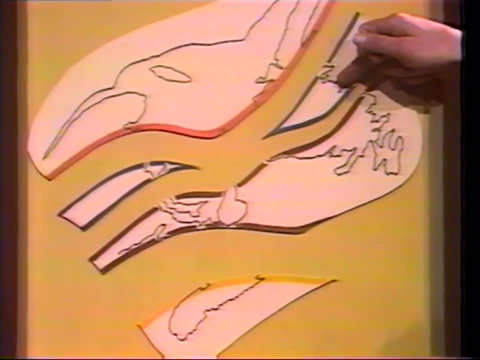 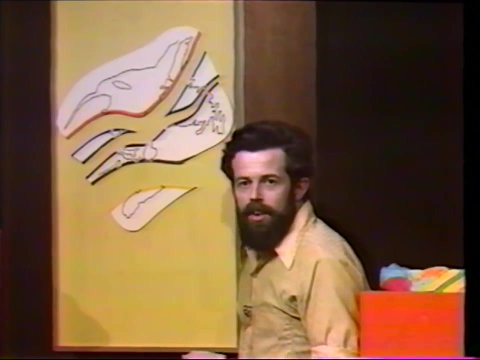 The major one in the central part of Newfoundland, A piece of continent that lay on the opposite side of that ocean, Forming the southwest part of Newfoundland, And finally, a piece of Africa which forms the most coastal part of the complex of the Appalachians. 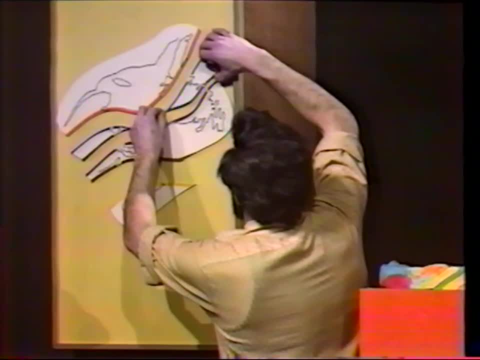 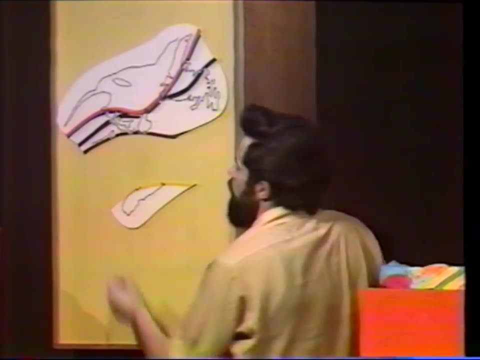 in the Maritimes. So remember that composite picture of Newfoundland while you look at the second part of this unit.